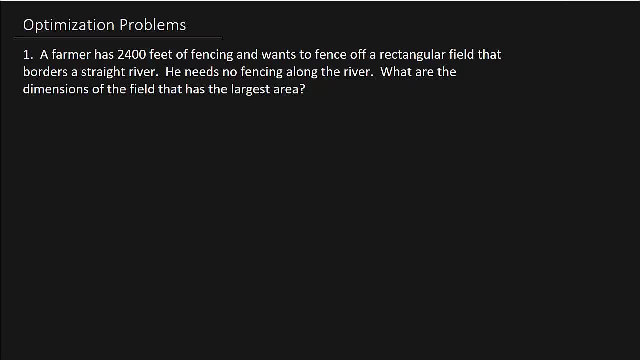 the river. what are the dimensions of the field that have the largest area? all right, so let's make a drawing, let's sketch it. so there's the river, and then we're going to have some fencing right here, all right, so here's, here's the three sides of fencing right here. 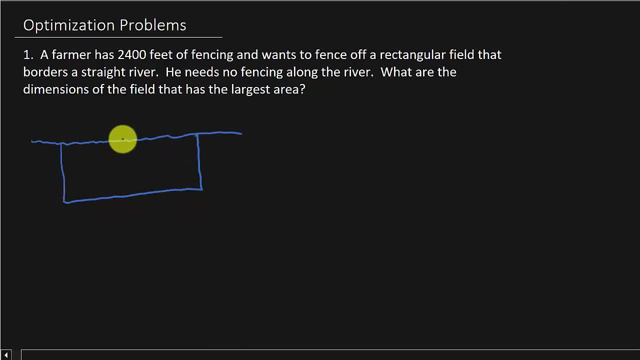 okay, these are the three sides. this is the river with no side, so let's label this X and Y. all right now let's take a look at and see what we have. so it says we have 2,400 feet of fencing. so that means, if I 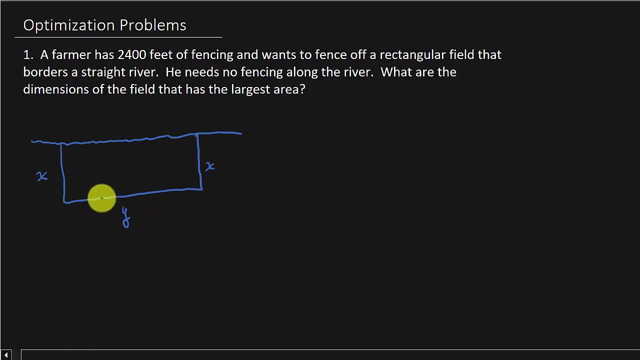 up all three sides, that should equal 2400. so if I have 2x plus y, that should equal 2400. all right, so that's, that's some information that I that I'm given. I've got an equation here and I want to maximize the area because it tells it. 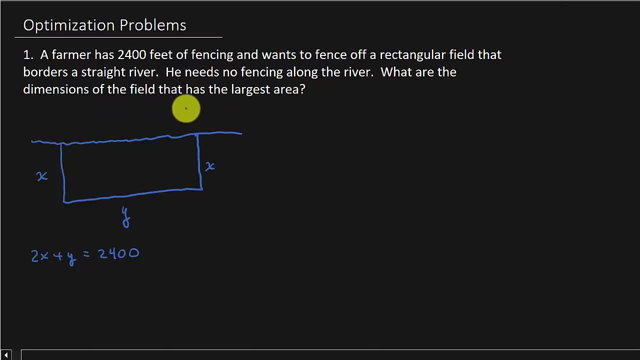 asked me what are the dimensions of the field that has the largest area? so what's the area of a rectangle? well, area is equal to length times width, or in this case, X times Y. so I want to maximize this, so I need to take the derivative of it. all right, but I want it in terms of one variable. so typically, 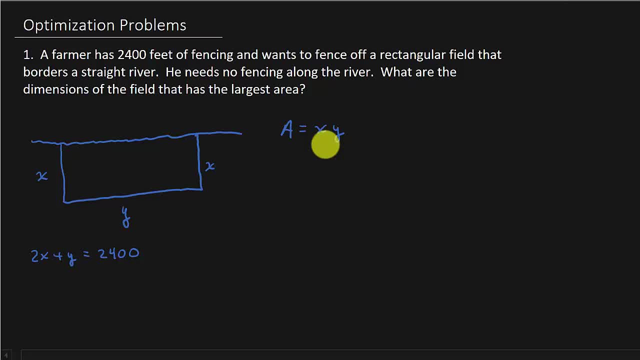 I want it in terms of one variable. so typically what I like to do is get everything in terms of X. so let's do that. well, how can I do that? well, over here I've got: 2x plus y equals 2400. so if I solve for Y, I 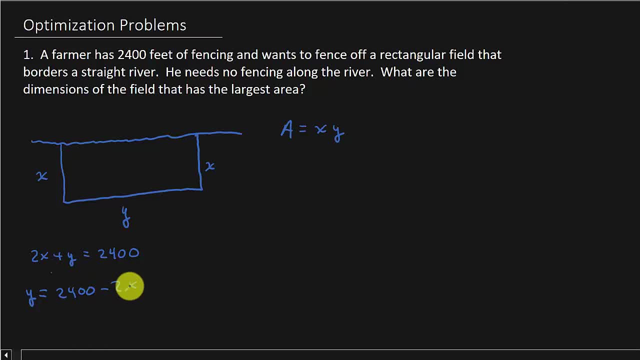 get. y equals 2400 minus 2x. so I can take this 2400 minus 2x, which that is equal to Y, and I can plug x. so if I solve for Y I can take this 2400, it in for Y, so I get area. let me switch color. so area is equal to x times 2400. 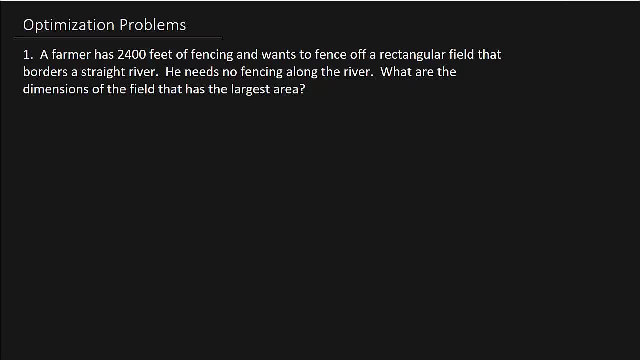 the river. what are the dimensions of the field that have the largest area? all right, so let's make a drawing, let's sketch it. so there's the river, and then we're going to have some fencing right here, all right, so here's, here's the three sides of fencing right here. 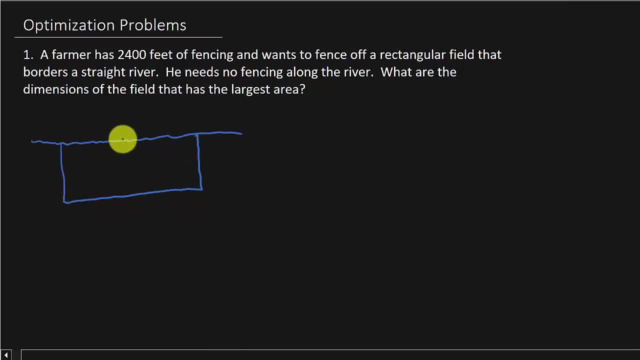 okay, these are the three sides. this is the river with no side, so let's label this X and Y. all right now let's take a look and see what we have. so it says we have 2,400 feet of fencing. so that means, if I 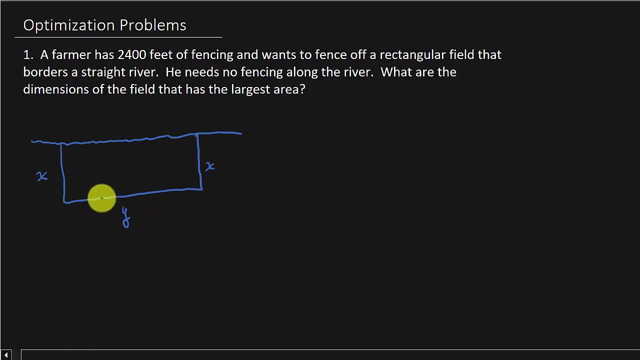 up all three sides, that should equal 2400. so if I have 2x plus y, that should equal 2400. all right, so that's, that's some information that I that I'm given. I've got an equation here and I want to maximize the area because it tells it. 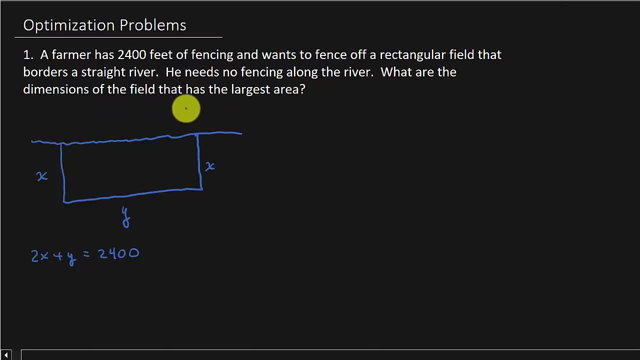 asked me what are the dimensions of the field that has the largest area? so what's the area of a rectangle? well, area is equal to length times width, or in this case, X times Y. so I want to maximize this, so I need to take the derivative of it. all right, but I want it in terms of one variable. so typically, 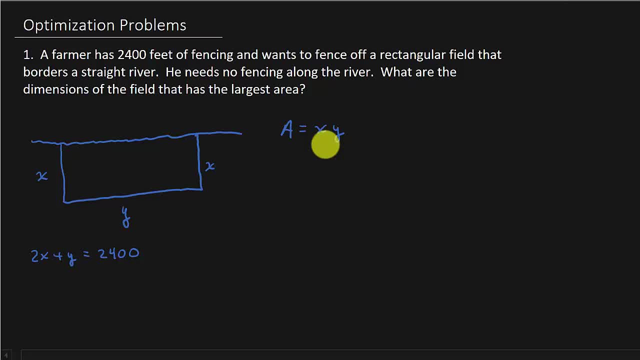 I want it in terms of one variable. so typically what I like to do is get everything in terms of X. so let's do that. well, how can I do that? well, over here I've got: 2x plus y equals 2400. so if I solve for y, I 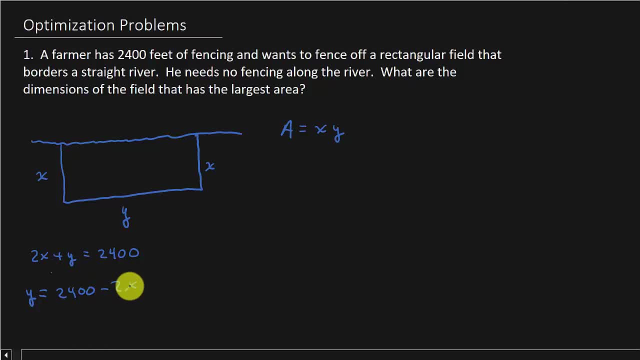 get. y equals 2400 minus 2x, so I can take this 2400 minus 2x, which that is equal to Y, and I can plug it in for Y, so I get area. let me switch color. so area is equal to X times 2400 minus 2x, and so my area is 2400 X minus 2x squared. all right now I was able to see a lot of the. 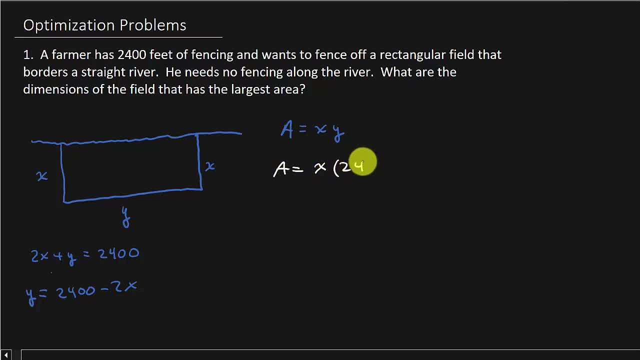 area is equal to X times 2400 minus 2x, and so my area is 2400 X minus 2x squared. all right now. Now the other thing that we want to look at also is we want to write down that X is going to be between 0 and 1,200.. 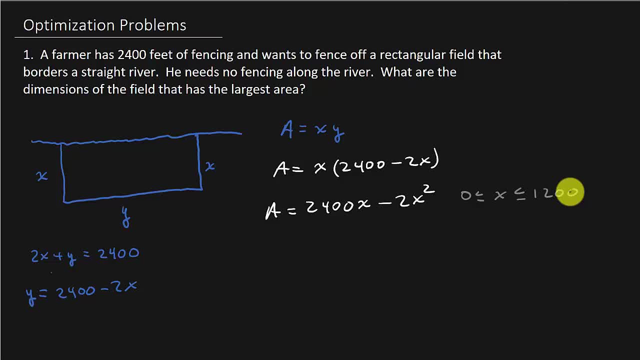 All right. Well, why is that? Well, I can't be less than 0. So if I have a number line up here and I have these two values here, well I know I can't be over here, because that would mean the side would be what? 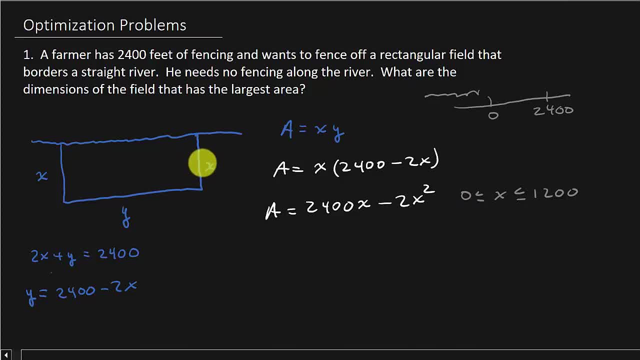 It would be negative and we can't have that. And if I'm more than 1,400, well, I'm sorry. if I'm more than 1,200, well, Well, that would do what? That would give me 0. 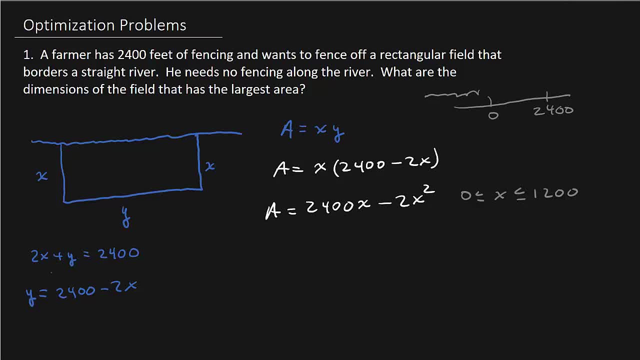 Okay, See, if I set this thing here equal to 0,, if I set this equal to 0,, well, look at it real quick: 2,400 X minus 2 X squared equals 0.. So that's going to be 2.. 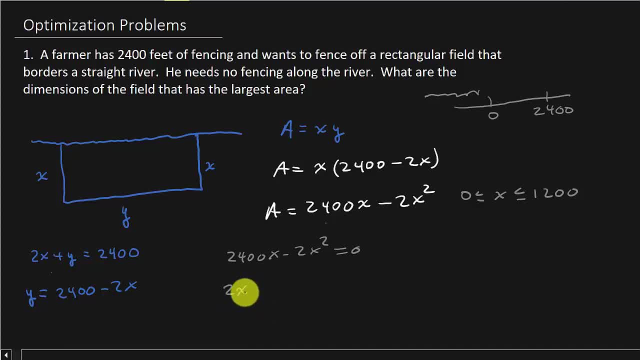 Ah, I'm sorry. So I've got 2 X times 1,200 minus X equals 0.. So you can see, if I set this equal to 0 and solve it, I get 0 and 1,200.. 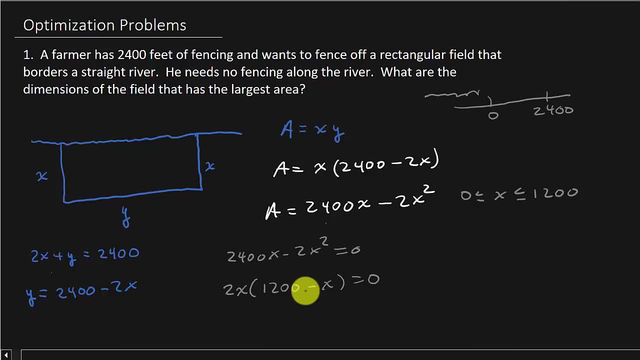 So I can't, I'm not going to be able to be outside of that. Okay, I'll get values that won't work. So here's my function. Here's my function that I want to maximize. Okay, I want to maximize this area here. minus 2x, and so my area is 2400 x minus 2x squared. all right, now I'm going to solve for x minus x and I can plug it in for y. I get area. let me switch colors. so area is equal to x times twenty-four-對2 subtitles are available, so I have to plug it in and I plug it in for y. so I get area and experience a lot. I'll do a. 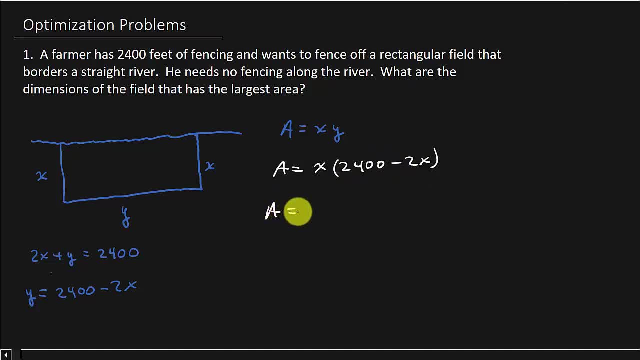 minus squared. all right now. I'm going to plug x and experience a lot inуб One'suvo window and check that for every fact: 2400 x minus 2x squared- all right now. the other thing that we want to look at also is we want to write down that X is going to be between 0 & 1200. all right. 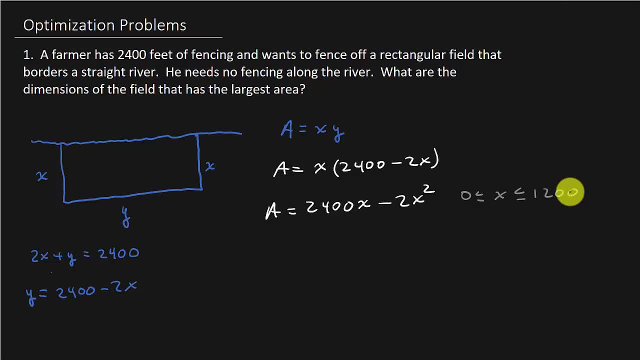 well, why is that? well, I can't be less than 0. so if I have a number line up here and I have these two values here, well i know i can't be over here because that would mean the side would be what, it would be negative and we can't have that. and if i'm more than 2400, 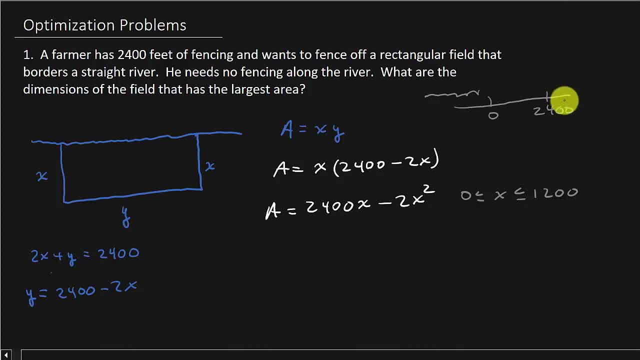 well, i'm sorry if i'm more than 1200. well, that would do what that would? that would give me zero. okay, see, if i, if i set this thing here equal to zero, if i set this equal to zero. well, look at it real quick. 2400. 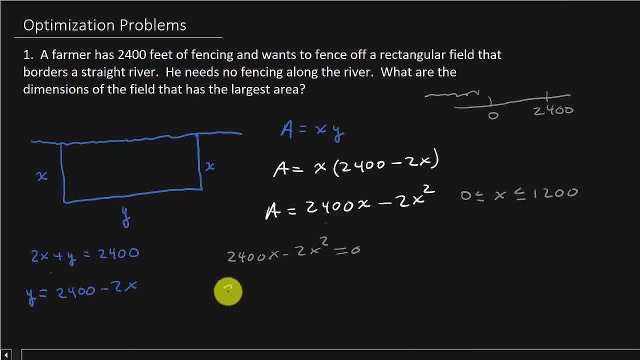 x minus 2x squared equals zero. so that's going to be 2. ah, i'm sorry, so i've got 2x times 1200 minus x equals zero. so you can see, if i set this equal to zero and solve it, i get zero. 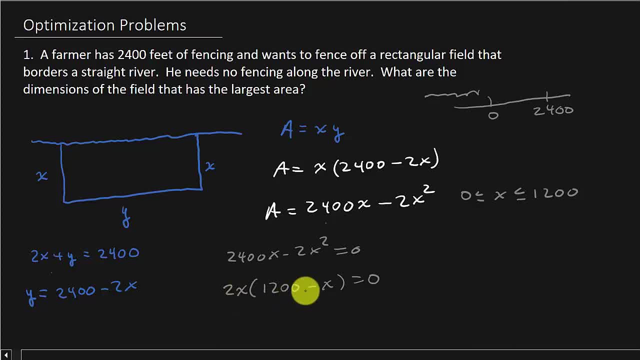 and 1200. so i can't- i'm not going to be able to be outside of that. okay, i'll get values that that won't work. so here's my, here's my function that i want to maximize. okay, i want to maximize this area here. 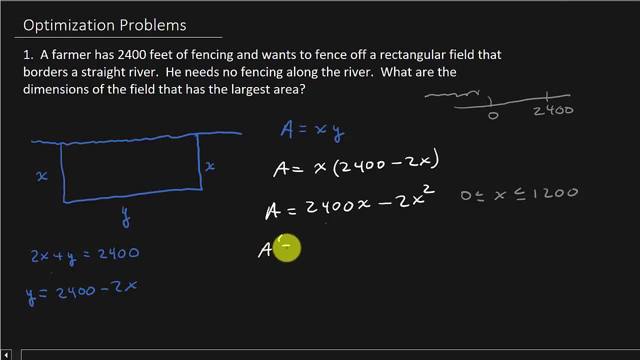 So we need to take the derivative. So I've got A prime is equal to 2,400 minus 4 X. And then what do we do? Well, we take the 2,400 minus 4 X, set it equal to 0.. 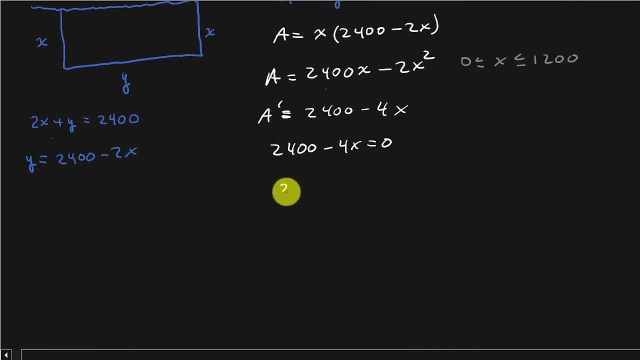 I'm finding my critical numbers, And so I get 2,400.. 2,400 equals 4 X, And so I get X is equal to: let's see 2,400 divided by 4. That's going to give us 600.. 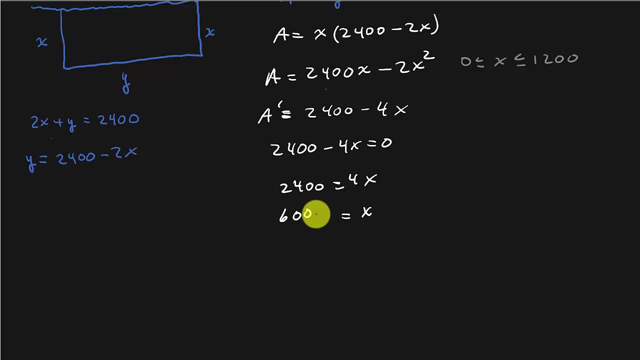 All right. Now what's going on here? Well, is this my solution? Well, remember, we're on a closed interval Interval here, So we need to see: is this is the 600, is that our maximum value? 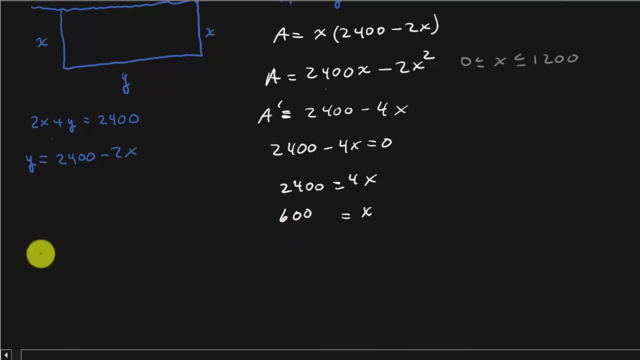 Okay, So do you remember how to do you remember how to do this? We've got A is equal. ah, I'm sorry, We've got A of 0. Remember, you test it at the 600.. And then you have to test it at each of these endpoints back into. 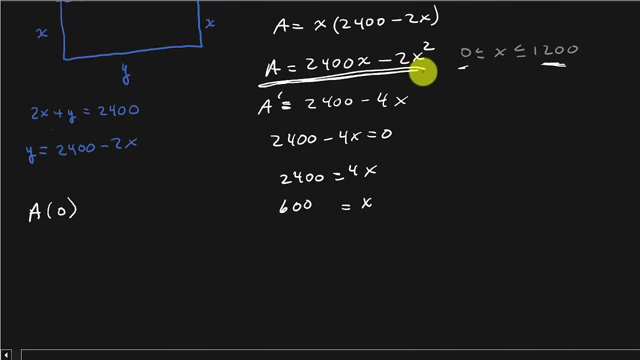 where is it? back into the original function. And remember: the smallest values gives you the minimum, The largest values gives you the maximum. All right, So that's going to be well. A of 0, if I plug that into here. 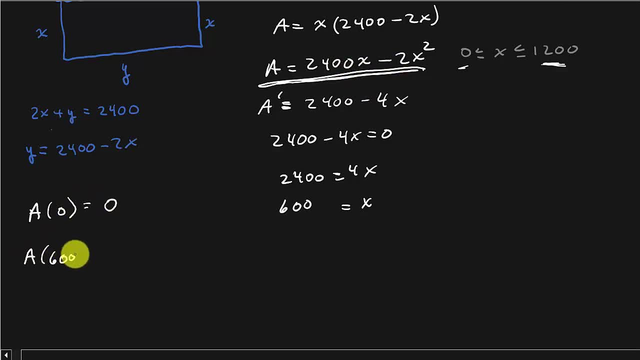 that's going to give me 0.. And then A of 600, well, if I plug the 600 in for X, that is actually going to give me 700.. And then, if I plug the 600 in for X, that is actually going to give me 1,620,000. 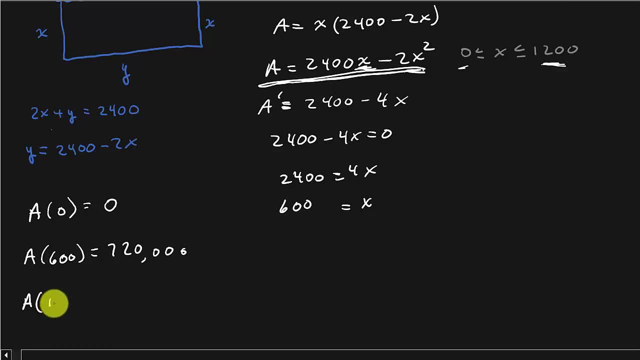 And then if I do A of 1,200, that's going to give me 0 also. So you can see that of the three, the 600 gave me the largest area. So the dimensions of the rectangle would be 600 feet. 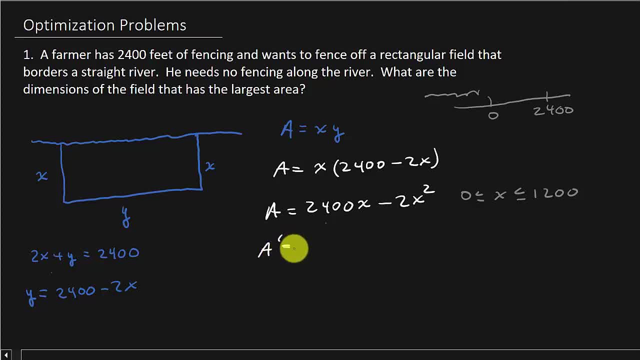 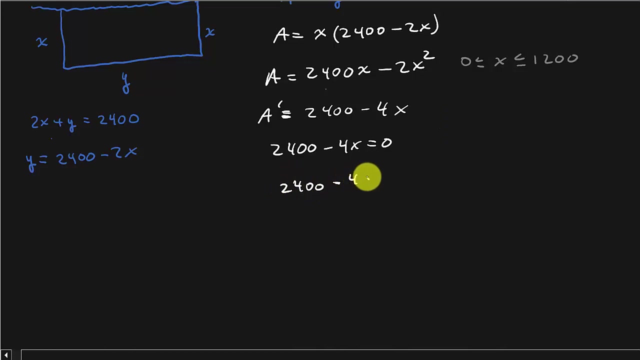 so we need to take the derivative. so i've got a prime is equal to 2400 minus the 4x. and then what do we do? well, we take the 2400 minus 4x says it equal to 0.. i'm finding my critical numbers and so i get 2400 equals 4x. 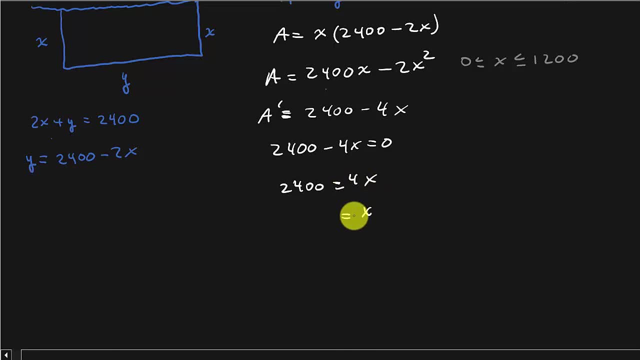 and so i get: x is equal to 0.. equal to, let's see: 2400 divided by 4, that's gonna give us 600. all right now, what's what's going on here? well is this. is this my solution? well, remember, we're. 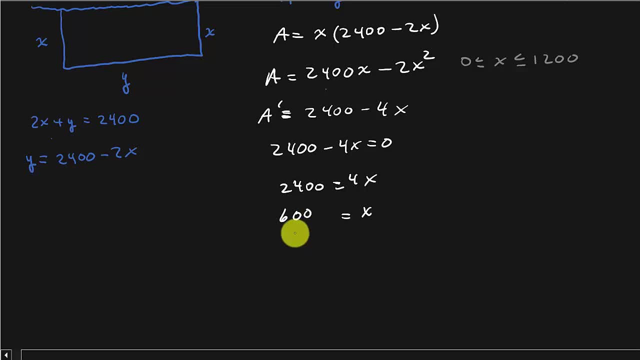 on a closed interval interval here. so we need to see: is this is the 600? is that our maximum value? okay, so do you remember how? to you remember how to do this? we've got a is equal. I'm sorry, we've got a of zero. remember you, you? 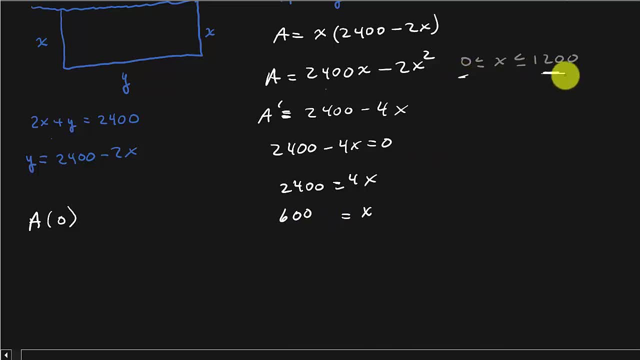 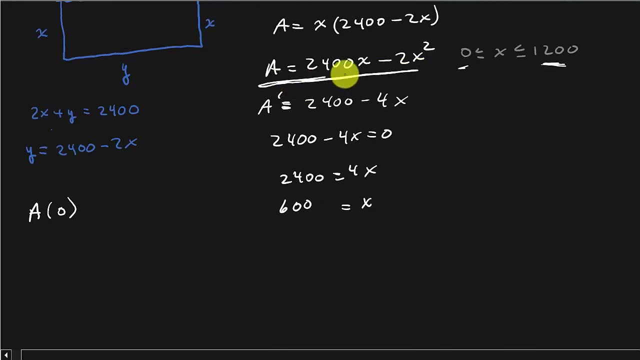 test it at the 600, and then you have to test it at each of these endpoints. back into where is it? back into the original function. and remember: the smallest values gives you the minimum, the largest values gives you the maximum. all right, so that's gonna be well a of zero if I plug that into here. 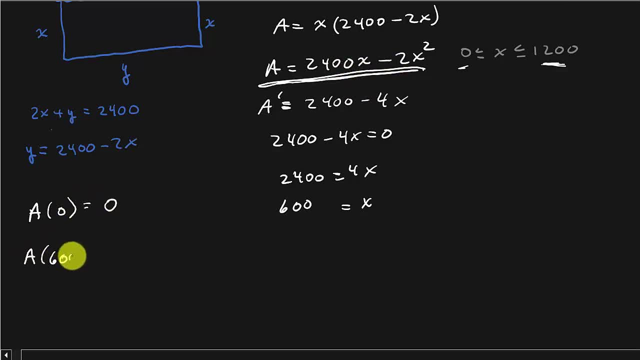 that's going to give me zero and then a of 600. well, if I plug the 600 in for X, that is actually going to give me seven hundred and twenty thousand. and then, if I plug the 600 in for X, that is actually going to give me, and if I do, a of 1200. 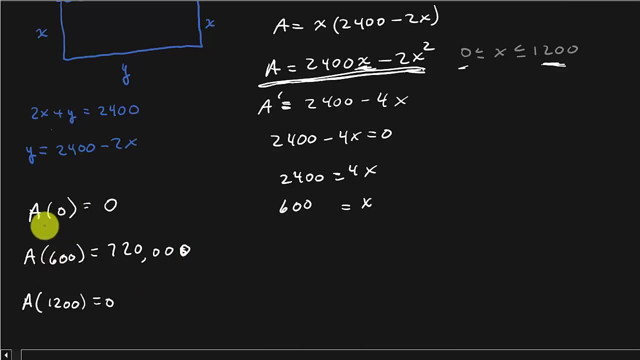 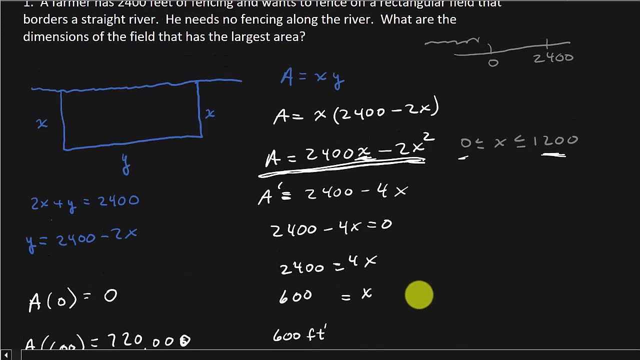 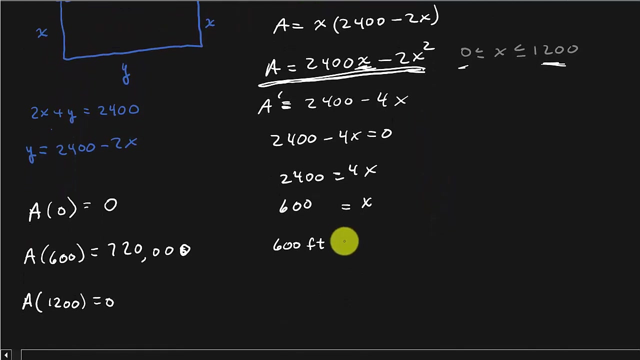 that's going to give me zero also. so you can see that, of the three, the 600 gave me the largest area. so the dimensions of the rectangle would be 600 feet. let's make sure we're in feet. yeah, 600 feet by what? Well, remember the 600 feet? that's the x value. Well, now I need the y value. 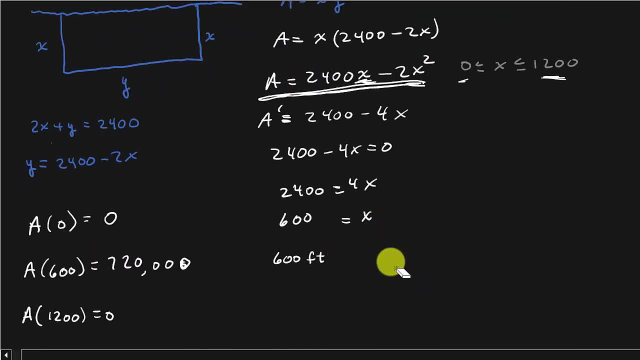 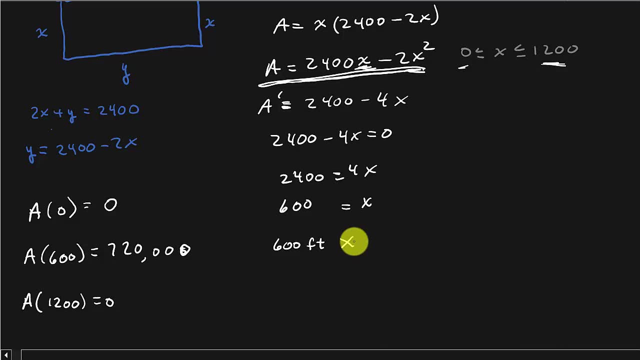 Let's make sure we're in. So 600 feet, yeah, 600 feet, by what? Well, remember the 600 feet? that's the X value. Well, now I need the Y value. Well, what's my Y value? 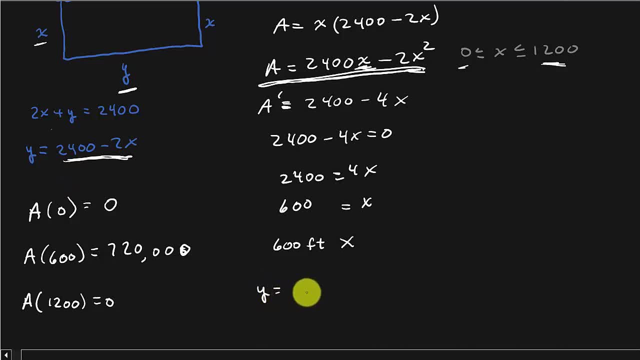 Well, that's this right here. So Y is equal to 2,400 minus 2 times 600, which that's going to be 1,200.. So that's by 1,200 feet. So that would be the dimensions. that gives me the largest area. 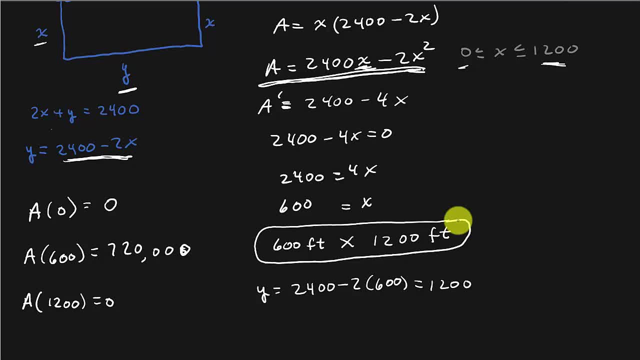 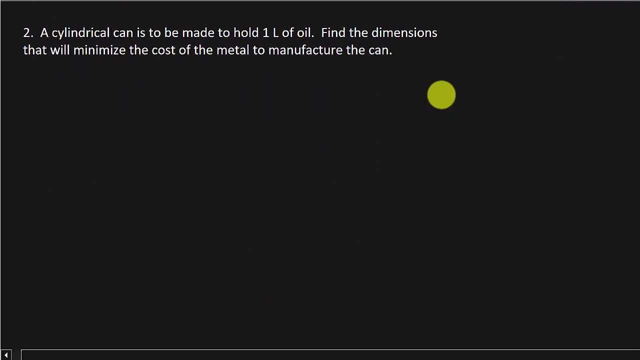 All right, All right, let's look at the next one. All right, it says a cylindrical can is to be made to hold one liter of oil to find the dimensions that will well find the dimensions that will minimize the cost of the metal. 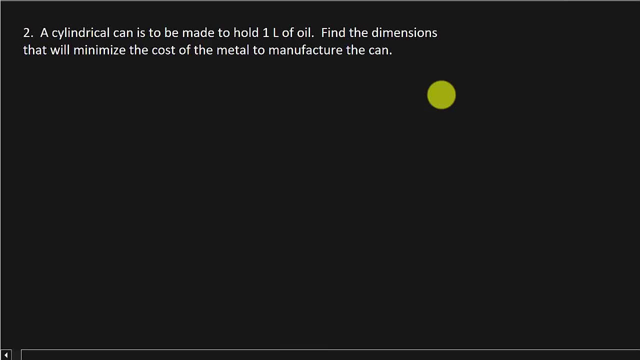 to manufacture the can, All right. So let's see what we've got. Let's draw a picture. So if I draw a cylindrical can, all right, let's draw the radius, and then we have the height. okay. 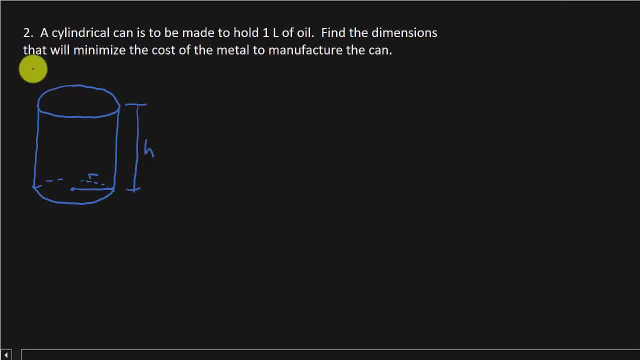 Now let's see what we're trying to find. Find the dimensions that will minimize the cost of the metal to manufacture the can. So that means we want the least surface area. okay, We want the least amount of the surface area. 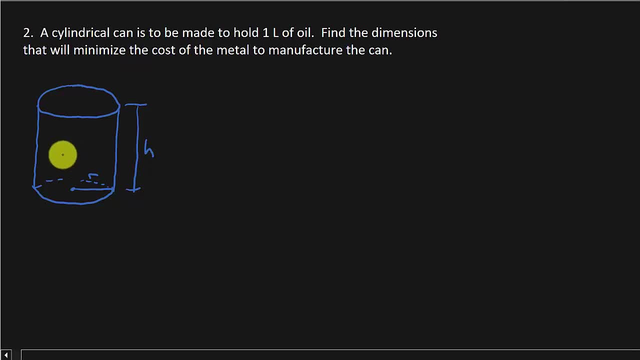 Now, of course we're going to have to assume in this problem that the cost to manufacture the cylinder and the cost to manufacture the top and the bottom all cost the same. okay, So we want to minimize that surface area, all right? 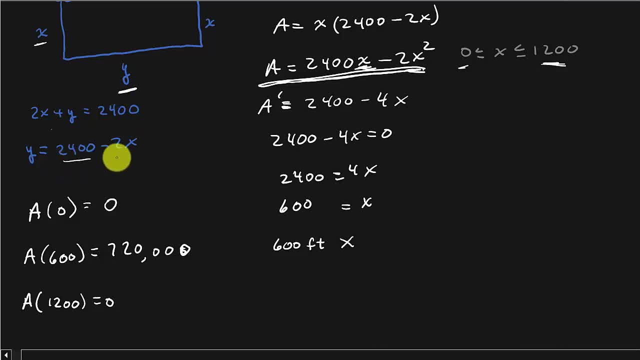 Well, what's my y value? Well, that's this right here. So y is equal to 2400 minus 2 times 600, which that's going to be 1200.. So that's by 1200 feet. So that would be. 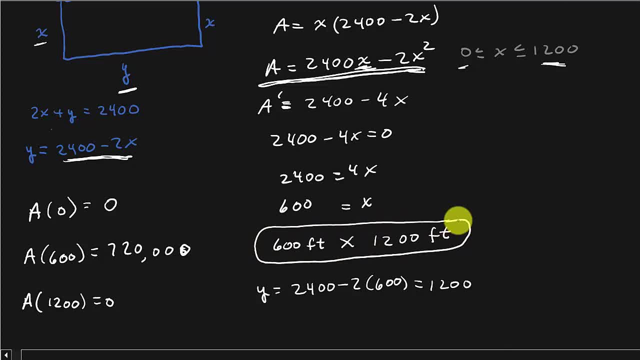 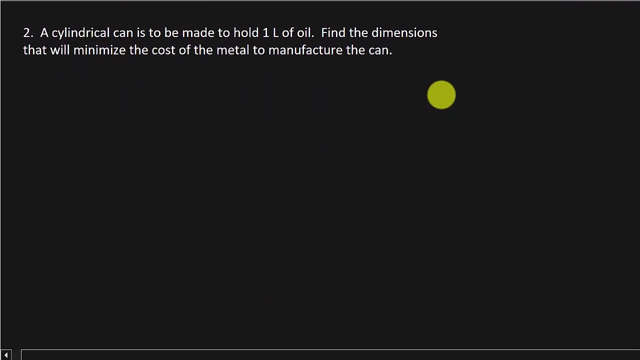 the dimensions. that gives me the largest area. All right, All right, Let's look at the next one. All right, It says a cylindrical can. It's to be made to hold one liter of oil. to find the dimensions, that will well find. 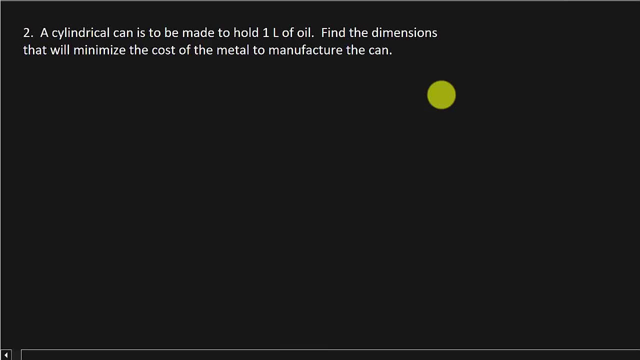 the dimensions that will minimize the cost of the metal to manufacture the can. All right, So let's see what we've got. Let's draw a picture. So if I draw a cylindrical can, all right, let's draw the radius and then we have the height. Okay, Now let's see what. 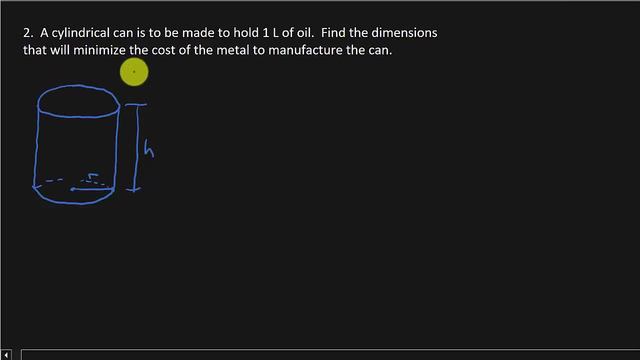 we're trying to find- Find the dimensions that will minimize the cost of the metal to manufacture the can. So that means we want a small amount of oil. That's going to be now. all we want is a large amount of oil and then we have a diameter of 2 meters. We 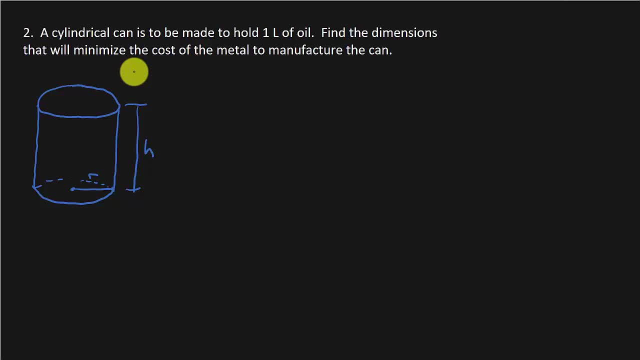 want a deep diameter? All right, Something that's big enough to hold a can is a small. we want the least surface area? okay, we want the least amount of the surface area. now, of course, we're going to have to assume in this problem that the the cost to manufacture the cylinder. 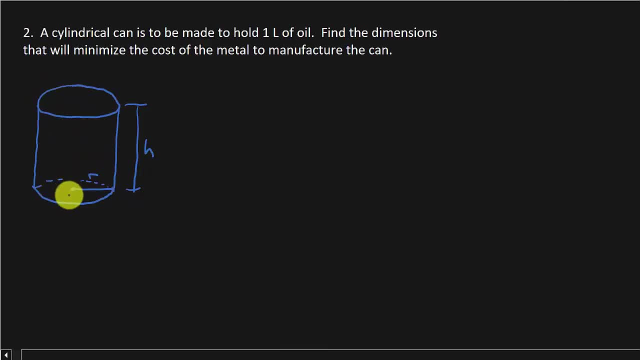 and the cost of manufacture. the top and the bottom all cost the same. okay, so we want to minimize that surface area, all right now. first let's, let's see. let's see what we have here. we're going to have two equations, the information that it gives us, and then we're going to come up. 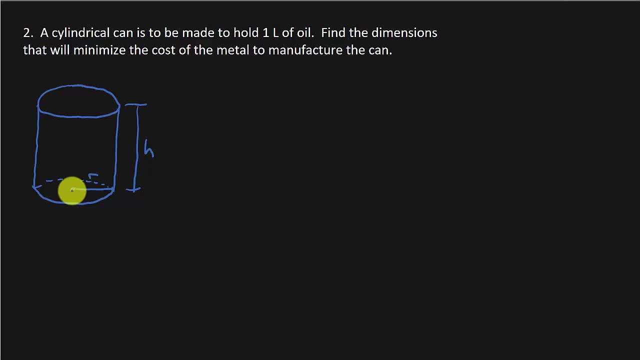 All right Now, first let's Let's see what we have here. We're going to have two equations, the information that it gives us, and then we're going to come up with an equation on that. you know, kind of like we did up here in this problem. 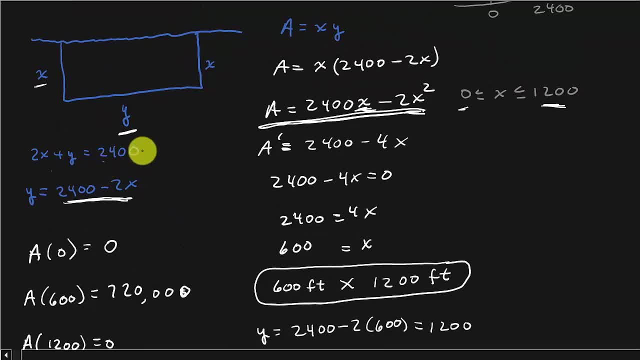 where we got the 2x plus y equals 2400, and then we're going to have to come up with a function that we've got. in this case, we need to minimize it, you know, like we did here. All right, 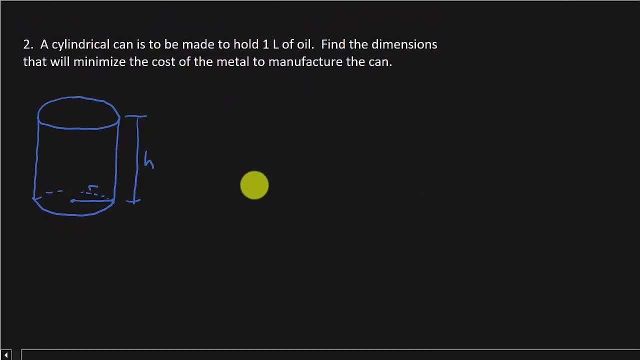 So let's look. So it tells us that a cylinder is to be made to hold one liter of oil. okay, Well, one liter is equivalent to what? 1,000 cubic centimeters? okay, We want to get it in units that. 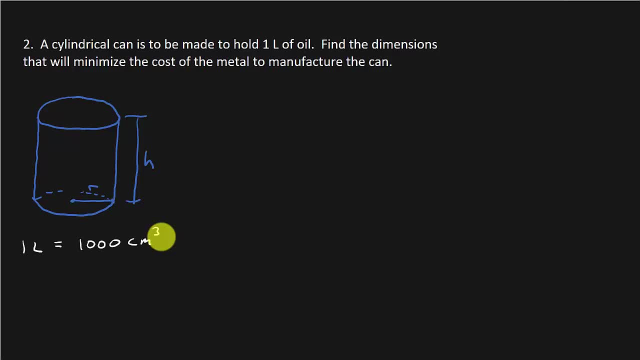 that we can measure. you know, you know height, you know a distance, So we're going to write the liters in terms of cubic centimeters. all right, All right. Now what's going to be the function that we want? to maximize or minimize? 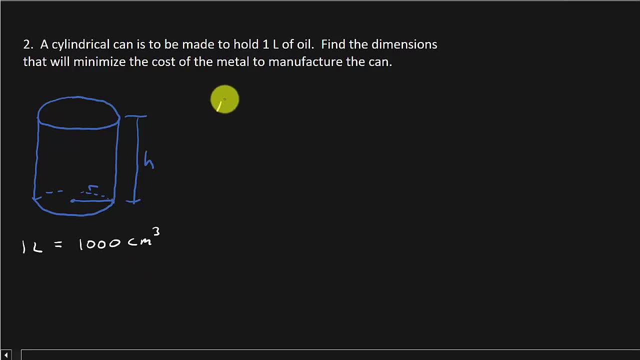 Well, that's the surface area. So, what's the surface area? Well, the surface area, We'll call that A. That is going to be the area of the top and bottom. Well, what's the area of the top? 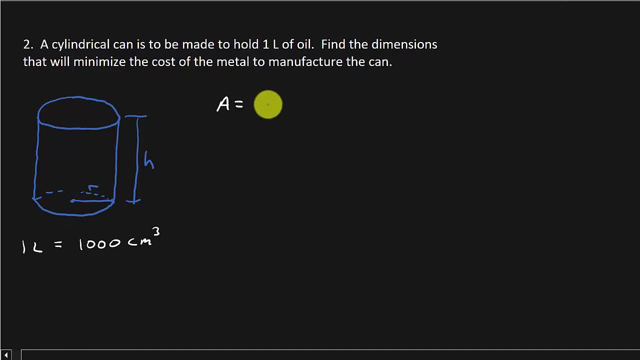 Well, the radius is r, So we know the radius of a circle is pi? r squared, and then that's going to be times 2, because we have the top and the bottom, We have two circles, And then plus plus. 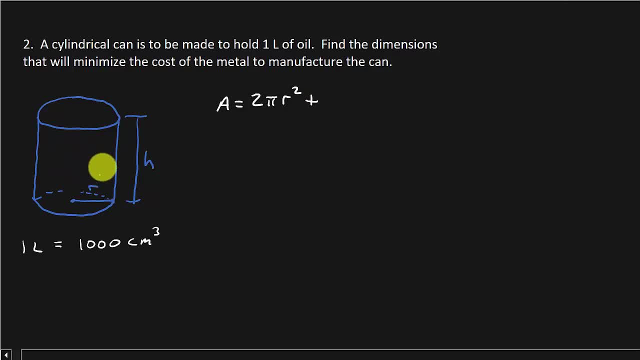 the surface area of what? The actual cylinder. okay, So what's the surface area of the cylinder? Well, remember that if you take a cylinder and you- and let's just assume we just kind of cut it right here and we fold it open, 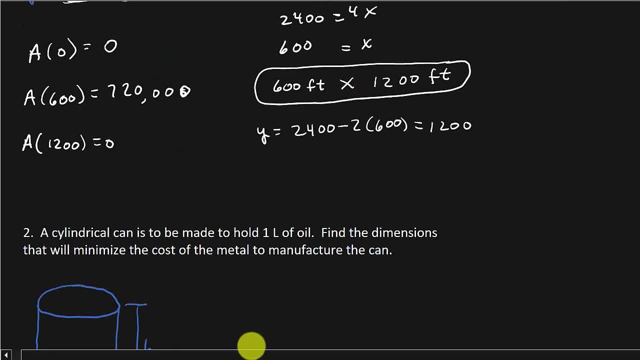 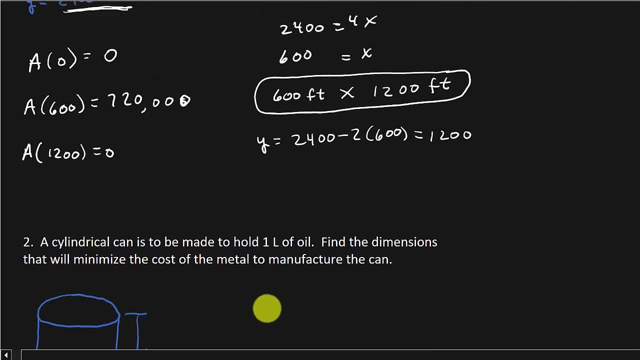 with an equation on that. you know, kind of like we did up here in this problem, where we got the 2x plus Y equals twenty four hundred, and then we're going to have to電ayo, alright, have to come up with a function that we've got. in this case we need to. 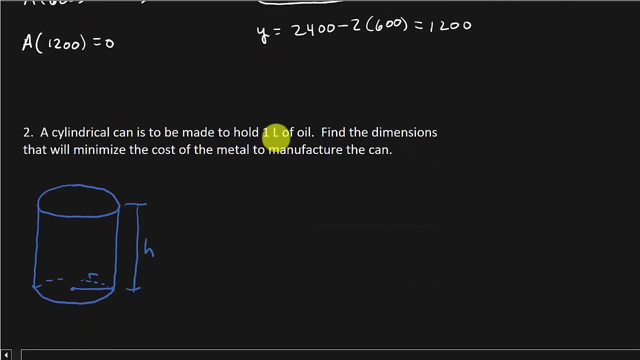 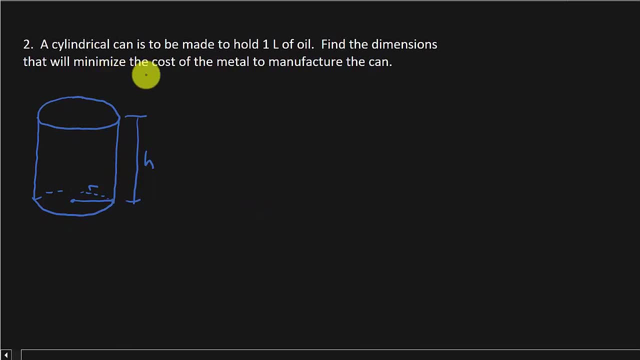 minimize it, you know, like we did here. all right, so let's look. so it tells us that a cylinder is to be made to hold one liter of oil. okay, well, one liter is equivalent to what? 1,000 cubic centimeters? okay, we want to. we want to. 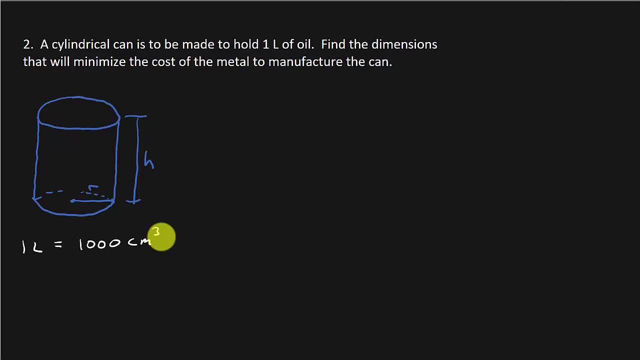 get it in units that we can measure. you know, you know height, you know a distance, so we're going to write the liters in terms of cubic centimeters. all right, all right, you, you, you. Now what's going to be the function that we want? to maximize or minimize? 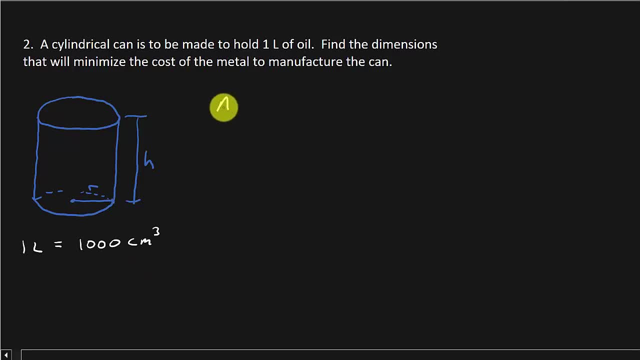 Well, that's the surface area. So, what's the surface area? Well, the surface area. call that a. that is going to be the area of the top and bottom. Well, what's the area of the top? Well, the radius is r. 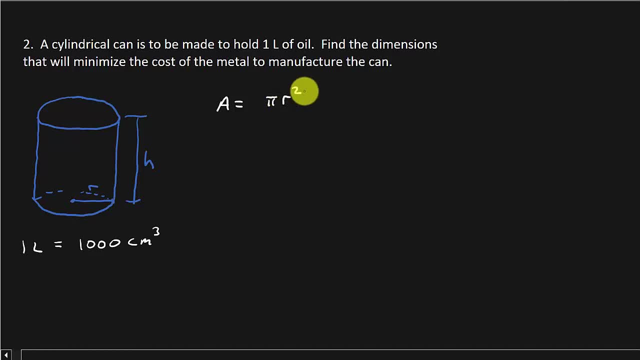 So we know the radius of a circle is pi r squared, And then that's going to be times 2, because we have the top and the bottom, We have two circles And then plus the surface area of what, The actual cylinder. 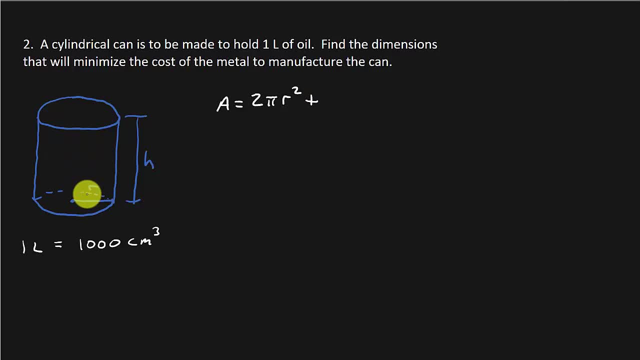 So what's the surface area of the cylinder? Well, remember that if you'd, if you take a cylinder and you- and let's just assume we just kind of cut it right here and we fold it open, that's just going to be like a rectangle, right? 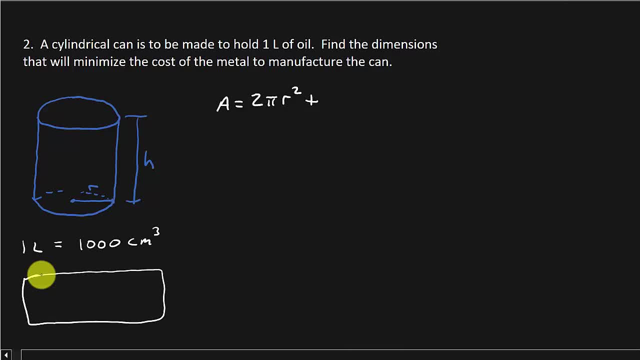 that's just going to be like a rectangle right. See this top here. when it unfolds, it'll unfold to this straight side here. and then here's the height. well, what's the distance of this right here? what's that distance there? well, it's the circumference of that circle. a is the circumference of the. 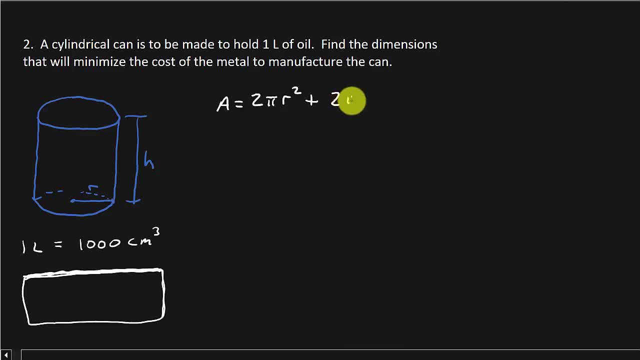 circle and the circumference of that circle is 2 pi R, or pi times the diameter, or 2 pi times the radius. okay, all this 2 R is just doubling the radius for the diameter, okay, and then this distance, here that's the height, so times H, all right. so there's our, there's our function, right there. now it does tell us: 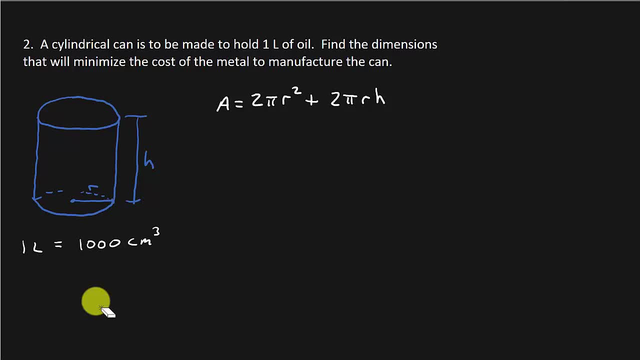 that the volume. okay, the volume is what the distance is where the circle is. so what we're really going to do is we're one liter or 1000 cubic centimeters. well, what's the? what's the volume of a cylindrical can? well, the 1000 is gonna equal to. well, what's the volume of this thing? well, remember the volume. if you take 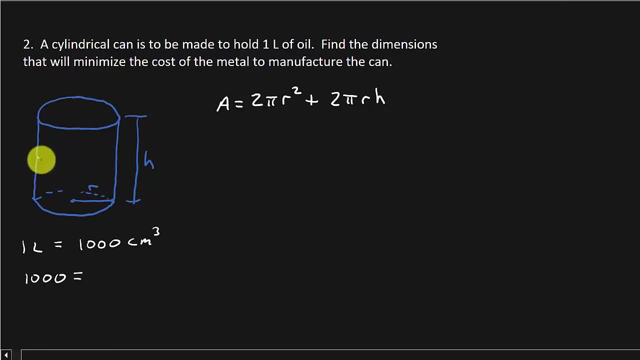 a cross-section, okay. so in other words, like, say, if you cut this can in half here and you and you look at it from the top or bottom, it's going to be a circle. so the volume would be the area of the cross-section, which is pi r squared times the height. all right, so what this is going to do. 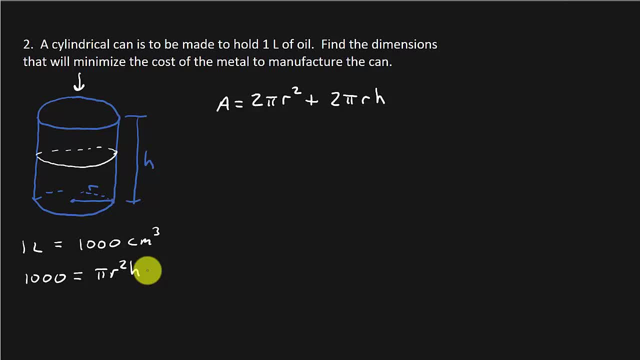 is. this is going to help us. it's going to help us get our function that we want to maximize or minimize, in terms of one variable, because you can see up here we've got everything. we've got it in terms of R and H for our variables. so 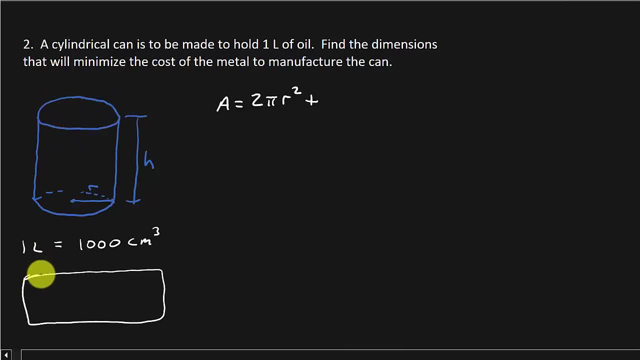 See this top here. when it unfolds, it'll unfold to this straight side here. And then here's the height. Well, what's the distance of this right here? What's that distance there? Well, it's the circumference of that. 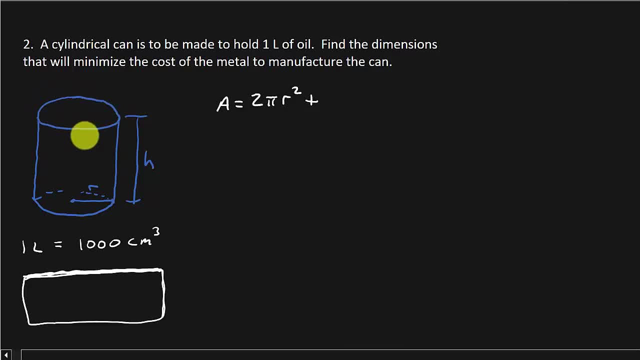 Well, it's the circumference of that. Well, it's the circumference of that. That circle is the circumference of the circle, And the circumference of that circle is 2 pi r or pi times the diameter, or 2 pi times the radius. 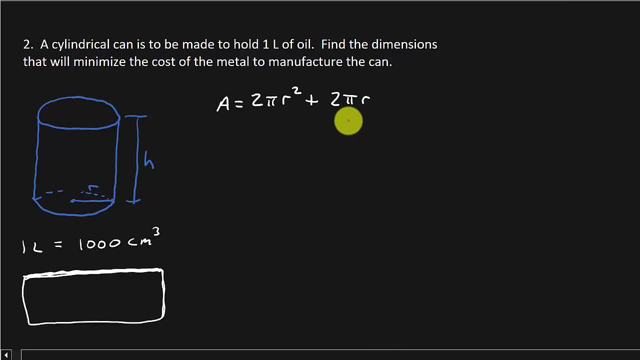 This 2r is just doubling the radius for the diameter And then this distance. here that's the height, So times h. So there's our, There's our function right there. Now it does tell us that the volume OK. 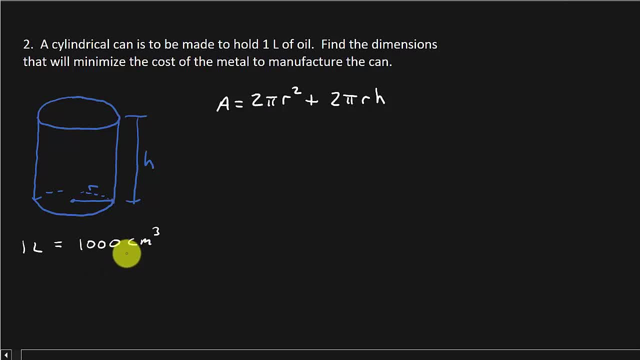 the volume is 1 liter or 1,000 cubic centimeters. Well, what's the volume of a cylindrical can? Well, the 1,000 is going to equal to. well, what's the volume of this thing? Well, remember the volume if you take a cross. 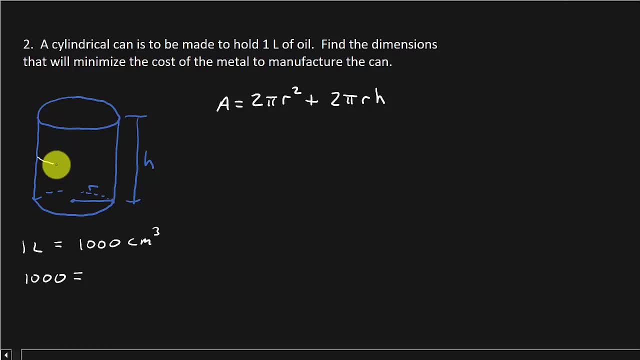 if you take a cross section, OK. so in other words, like say, if you cut this can in half here and you look at it from the top or bottom, it's going to be a circle. So the volume would be the area of the cross section which. 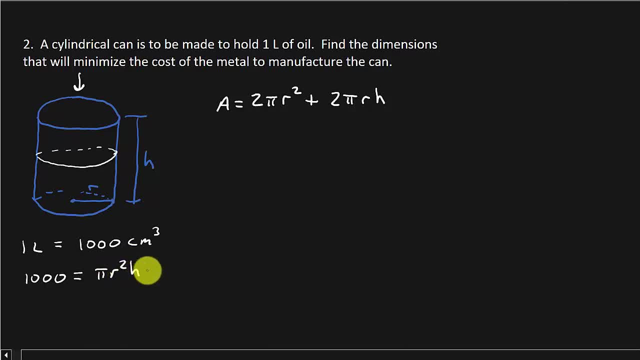 is pi r squared times the height. All right, So what this is going to do is this is going to help us- is going to help us get our function that we want to maximize or minimize in terms of one variable, Because you can see up here we've 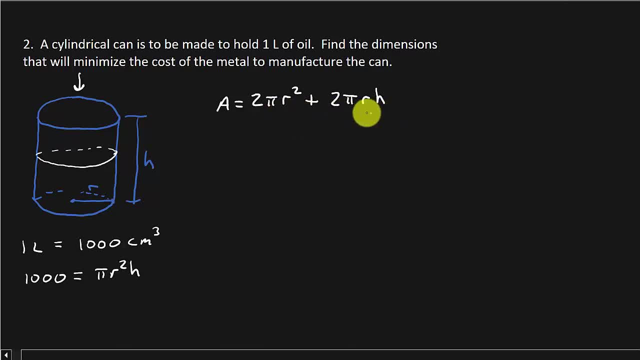 got every. we've got it in terms of r and h for our variables. So let's get everything in terms of r. So I need to know what h is in terms of r. Well, here I can see: h is 1,000 over pi r squared. 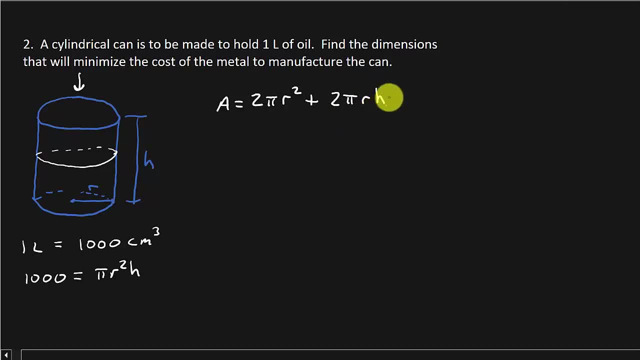 let's get everything in terms of R, so I need to know what H is in terms of R. well, here I can see H is 1000 over pi r squared, so I can replace H with a thousand over pi r squared. so a is equal to 2 pi r squared plus 2 pi r times 1000 over pi r squared, and so area is 2 pi r squared. 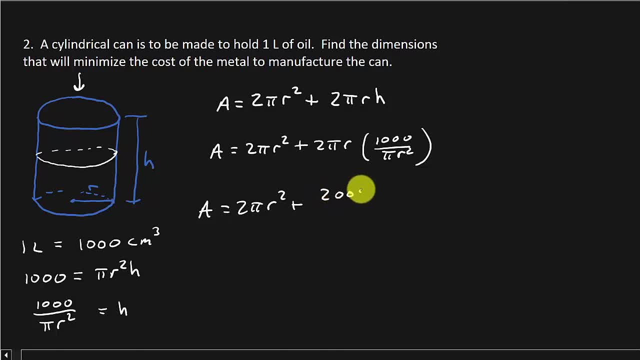 plus. and let's say, was it going to be 2000 over R? okay, now, what do we know about this? well, we know it's positive, right? R can't be negative. it's going to have to be larger than zero because the radius can't be negative. so if I take the derivative I get a prime is equal to 4 pi r. 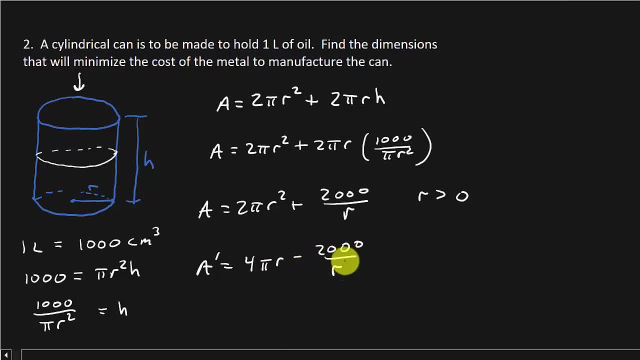 minus 2000 over R squared. so remember the 2000 over R. if we take the derivative of that 2000 over R, we take the derivative. well, what would that be? that would be 2000 R to the negative 1, and then we just use the power rule: negative 2000 R to the negative 2, and then that would: 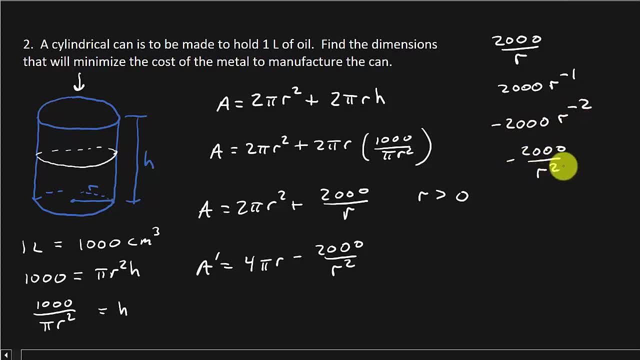 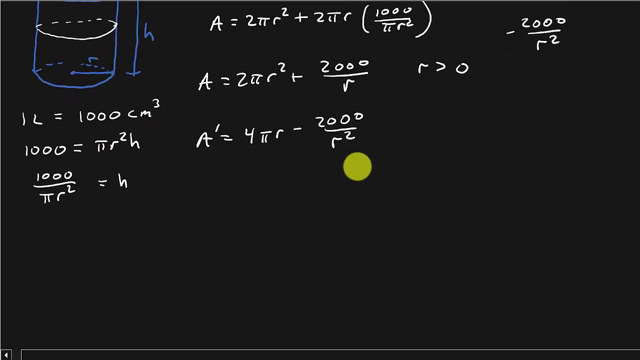 be negative 2000, and then move the R squared down there to the denominator, and that's where that 2000 R squared comes from. all right, and so now? what do we do? well, now, we set the derivative equal to zero. so, and I'm going to do, 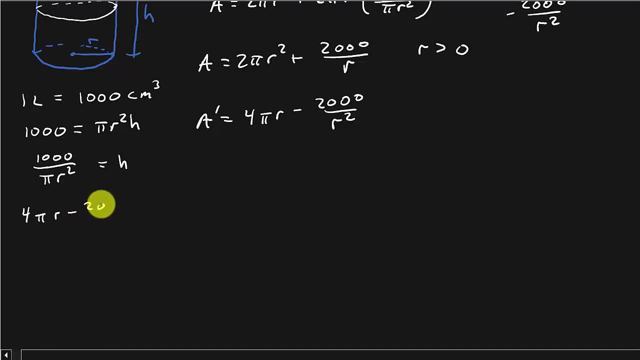 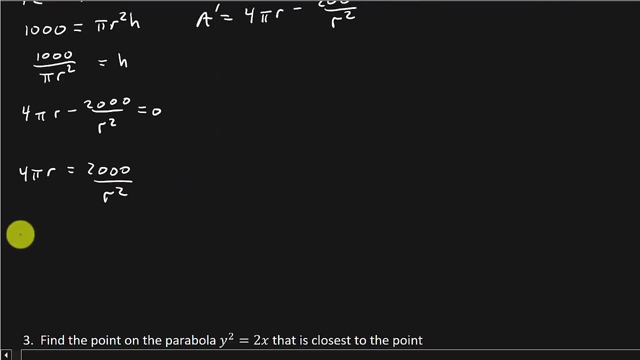 that here I got: 4 pi r minus 2000 over R squared equals zero. so 4 pi r equals 2000 over R squared. and so I get- let's see: r cubed is equal to what is that? 500 over pi? and so r is equal to the cube root of 500 over pi. 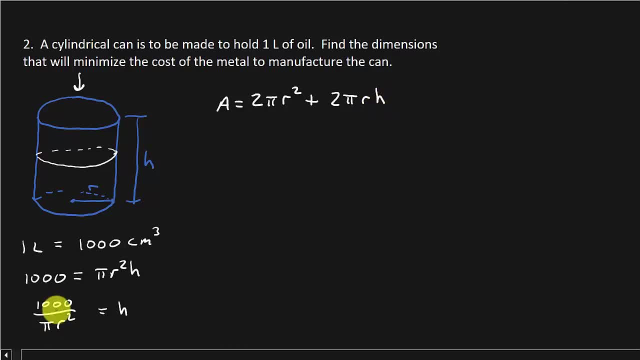 So I can replace h with 1,000 over pi r squared. So a is equal to 2 pi r squared plus 2 pi r times 1,000 over pi r squared, And so the area is 2 pi r squared plus. and let's see: 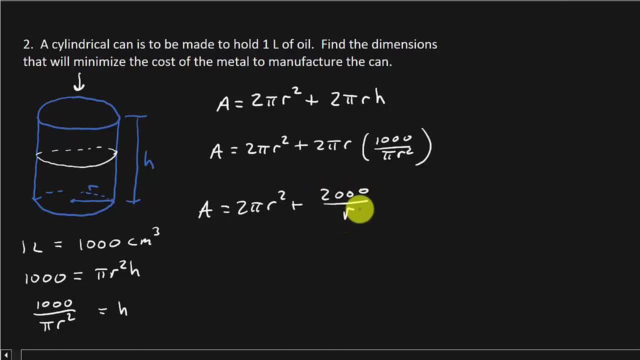 what is that going to be? 2,000 over r, 1,000 over pi, r squared. OK, All right. OK, Now what do we know about this? Well, we know that r is positive right, r can't be negative. 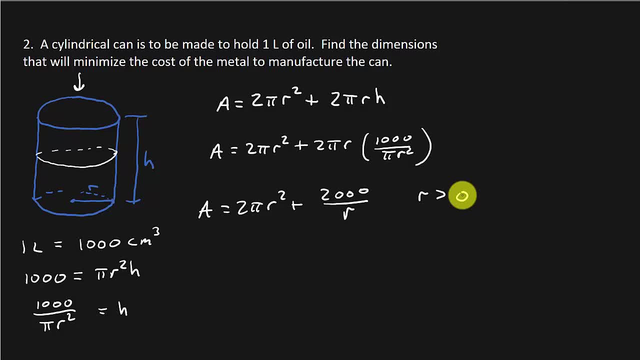 It's going to have to be larger than 0 because the radius can't be negative. So if I take the derivative I get a prime is equal to 4 pi r minus 2,000 over r squared. So remember the 2,000 over r if we take the derivative of that. 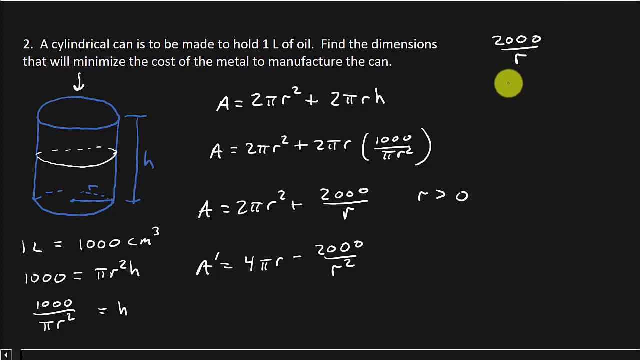 2,000 over r and we take the derivative. well, what would that be? That would be 2,000 r to the negative 1.. And then we just use the power rule: Negative: 2,000 r to the negative 2.. 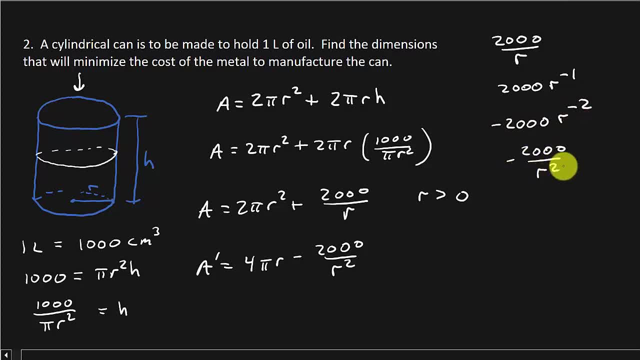 And then that would be negative 2,000, and then move the r squared down there to the denominator. OK, And that's where that 2,000 r squared comes from. All right, And so now? what do we do? 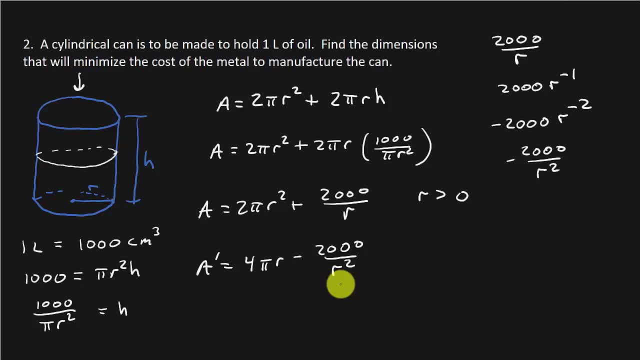 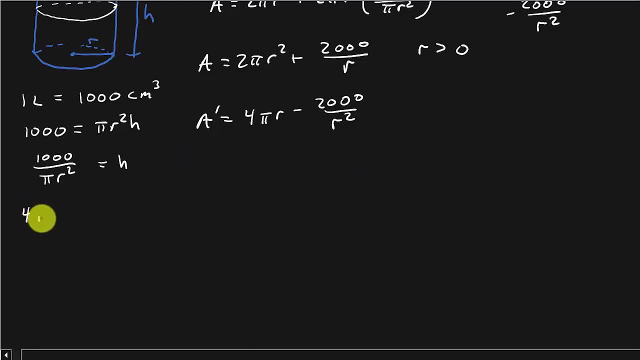 Well, now we set the derivative equal to 0.. So I'm going to do that here. I've got 4 pi r minus 2,000 over r, squared equals 0.. OK, All right. So now what do we do? 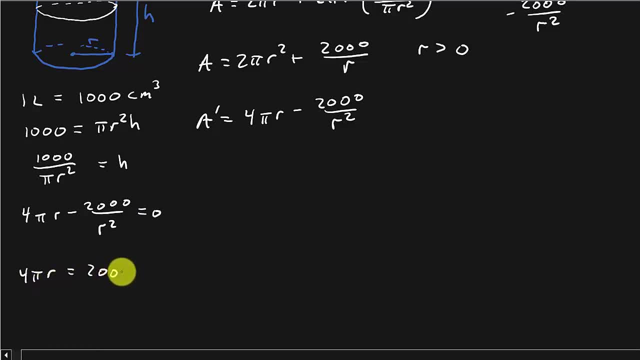 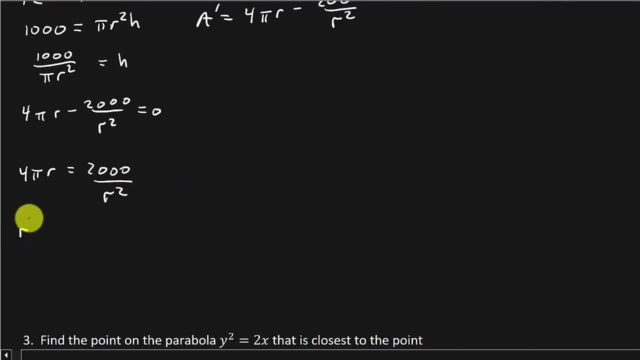 Well, we set the derivative equal to 0.. So 4 pi r equals 2,000 over r squared. And so I get, let's see: r cubed is equal to what is that? 500 over pi? And so r is equal to the cube root of 500 over pi. 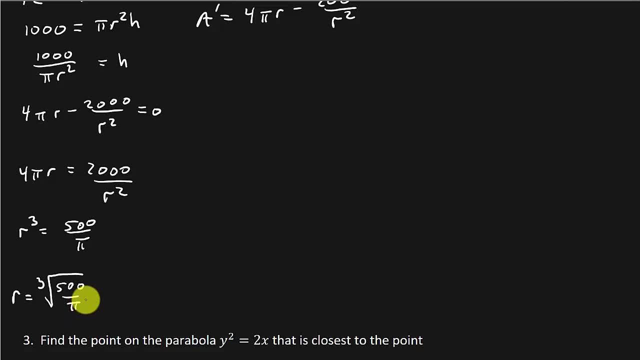 OK, All right. So now, what can we do? All right? Well, let's look at, maybe- I don't know- if we can do something to maybe simplify this a little more. I don't know, Maybe we can, maybe we can't. 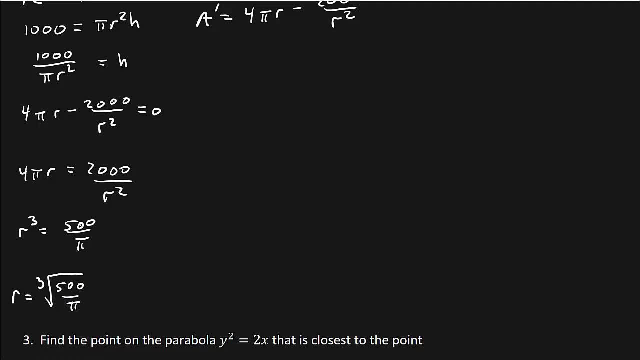 Let's look and see what we've got. All right. So I don't think there's. I don't think there's anything. I don't think there's much else we're going to be able to do with that r. So that would be, that would be r. 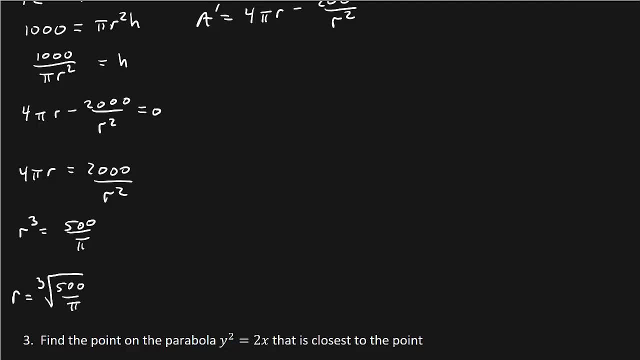 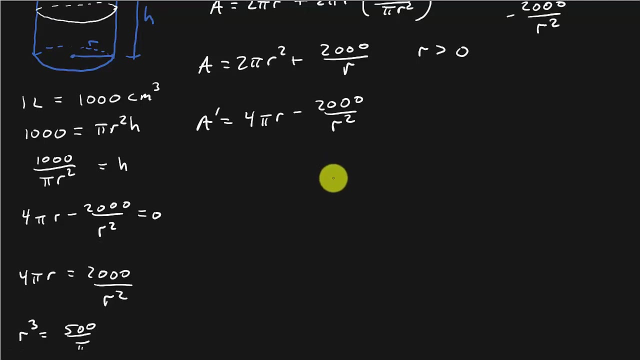 Now, well, we need to what We need to know the dimensions of the can And look, and we can show that this is a minimum You can. you can do your number line. OK, You can do your number line and everything. 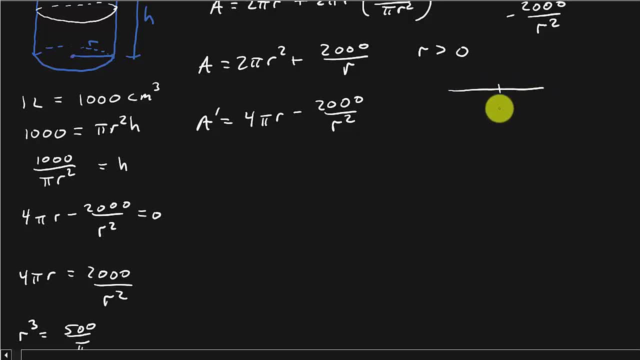 And it'll show that it's a minimum. You know what I mean. OK, You know what I mean When you take the, the cube root of 500 over pi, and you choose a number over here, choose a number over here and it'll show here it's decreasing and here it's increasing. 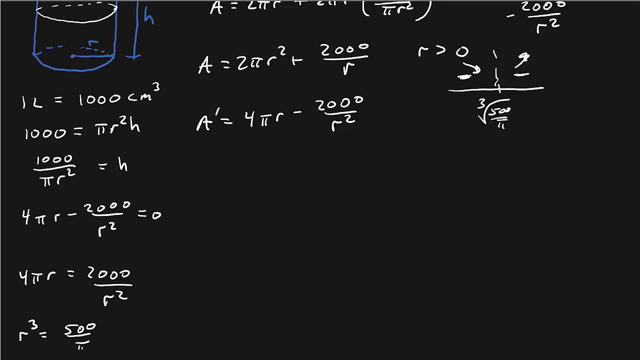 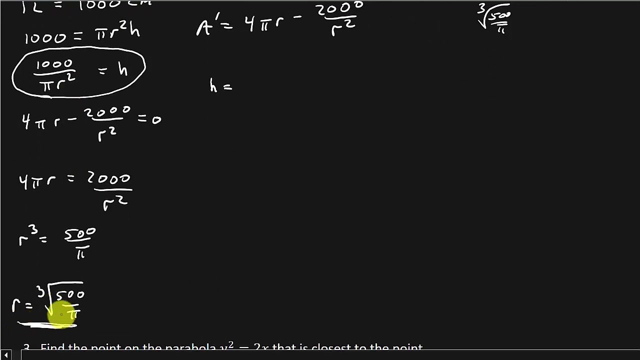 OK, All right. So anyway, let's, let's find h. All right, So h is equal to this. All right, So h is equal to this. So we need to plug r in what we got for r, which is the cube root of 500 over pi. 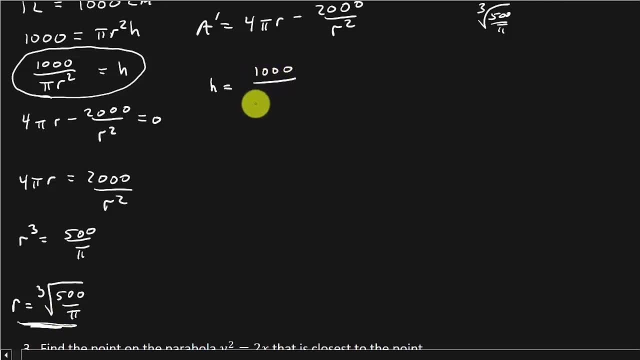 So h is equal to 1,000 over pi times the cube root of 500 over pi squared. All right, And so this is going to give us 1,000.. 1,000 over pi times 500 over pi to the 2 thirds. 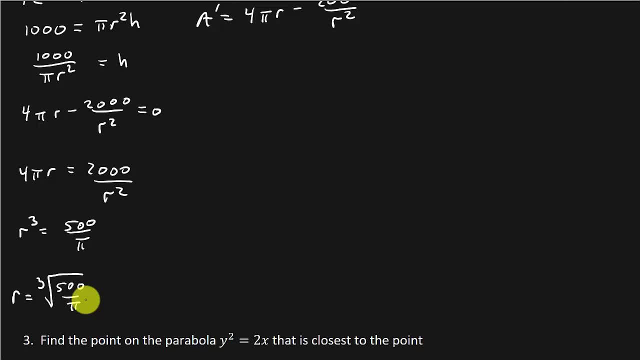 all right, so now, what can we do? all right? well, let's, let's look at- maybe- I don't know- if we can do something to maybe simplify this a little more. I don't know, maybe we can, maybe we can't. let's, let's look and see what we've got. 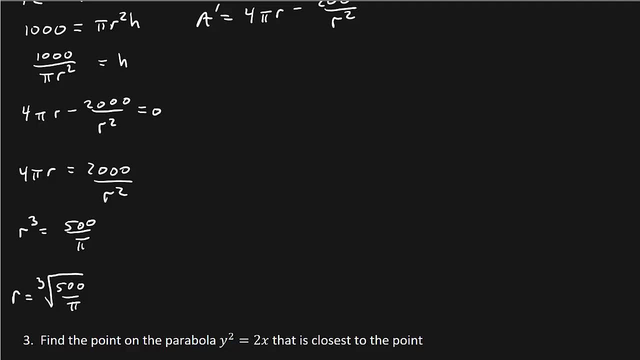 all right. so I don't think there's, I don't think there's, much else we're going to be able to do with that R. so that would be, that would be R. now, well, we need to what, we need to know the dimensions of the can and look and we can show that this is a minimum you can. you can do your. 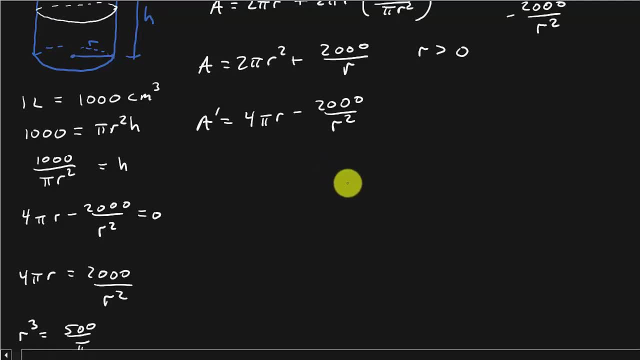 number line. okay, you can do your number line and everything and it'll show that it's a minimum. you know what I mean when you take the, the cube root of 500 over pi, and you choose a number over here. choose a number over here and it'll show: here it's decreasing, in, here it's increasing, okay. 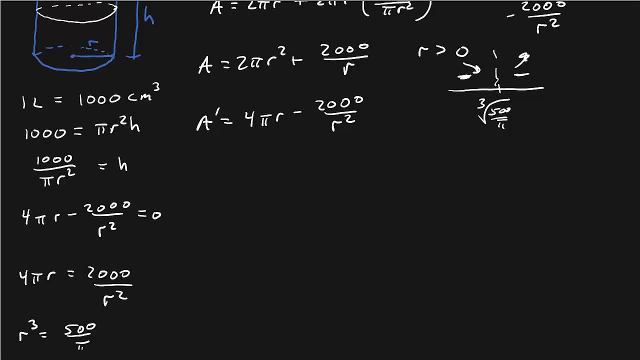 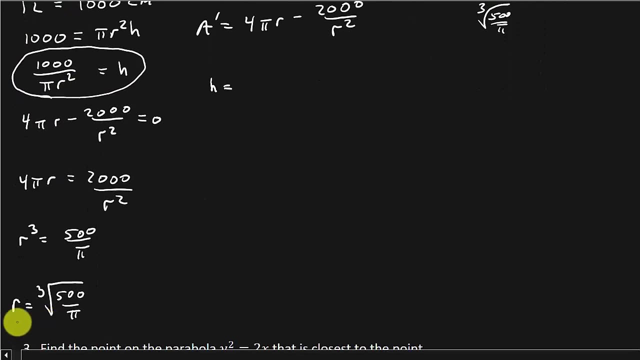 all right. so, anyway, let's, let's find h all right. so h is equal to this. so we need to plug are in what we got before we go intoич in what we got before we go into each of them, et al, and then, by default, r and possaiones are EH. 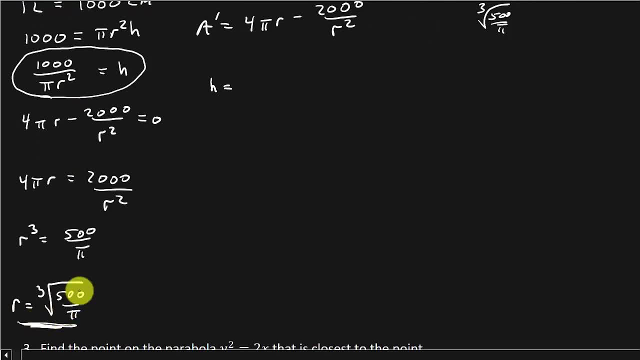 non 각 unique它 對還有渠讓 и他اء ლ. h equal to this date, and then h⃣ for R, which is the cube root of 500 over pi. so H is equal to 1000 over pi times. 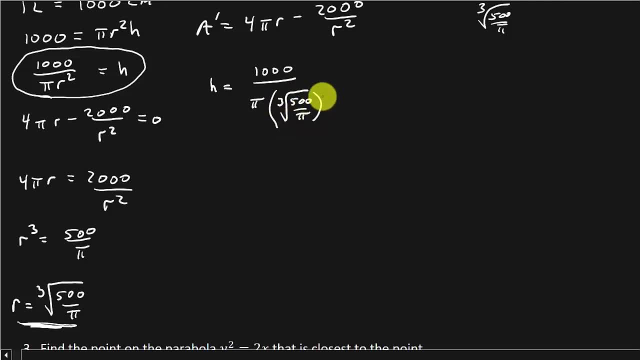 the cube root of 500 over pi squared all right, and so this is going to give us 1000 over pi times 500 over pi to the two-thirds. I just converted the, the radical, into exponential form. now let's see. let's see if we can. if we can. 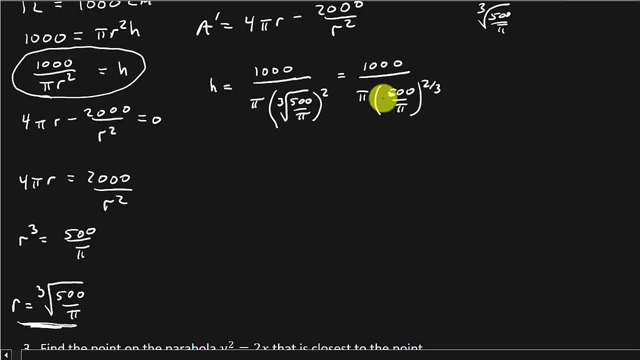 I just converted the, the radical, into exponential form. Now let's see. let's see if we can, if we can simplify this a little more, All right. So I noticed the 1,000.. I can write that as 2 times 500, and that's over pi times 500, over pi to the 2 thirds. 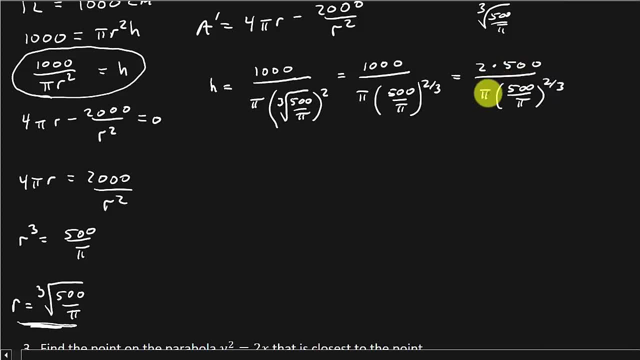 And then, if I separate this out, you see, you see this 500 over pi here and then this 500 over pi to the 2 thirds. Let's write this as 2 times 500 over pi, over 500 over pi. 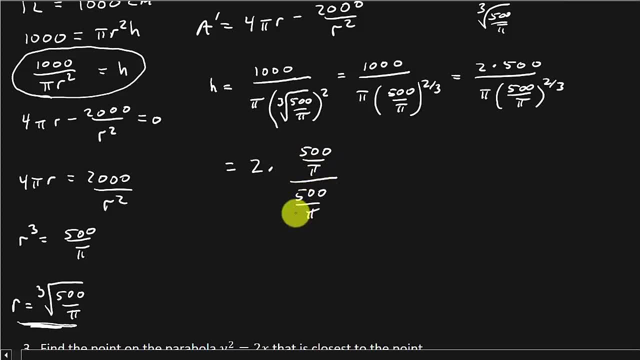 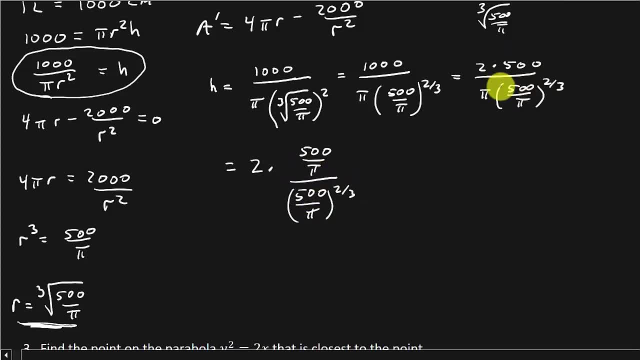 pi. I just wrote it up here in the numerator. Well, this is 2 times, and that's going to be 500 over pi to the what To the 1.. Okay, And so what we're going to write here is 500 over pi, and then this 500 over pi to: 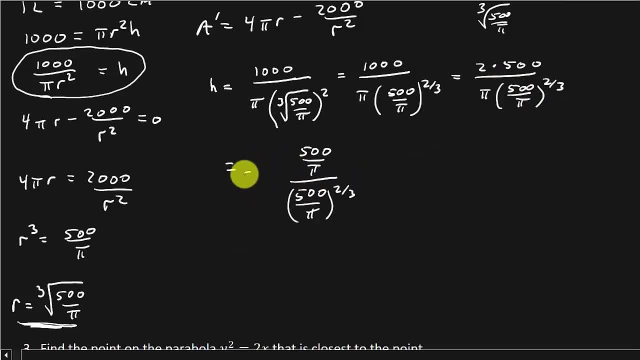 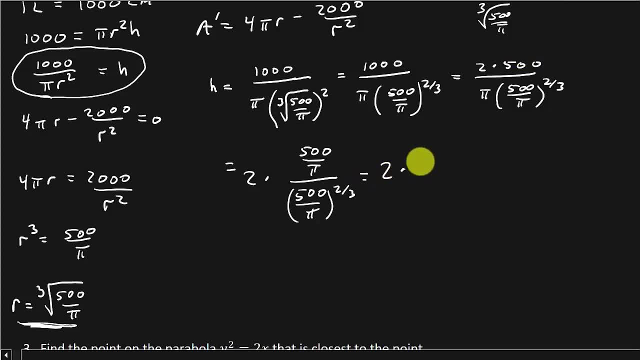 1,000. 1,000. 1,000. 1,000. 1,000.. that's going to be 500 over pi. to the what? To the 1 minus 2 thirds which that's going. 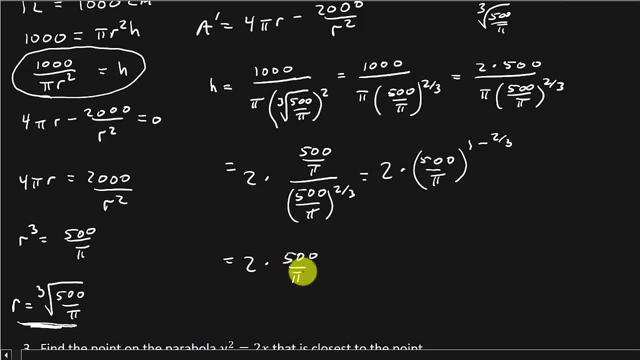 to be 2 times 500 over pi, to the 1 third, which is going to be 2 times the cube root of 500 over pi, And so I can actually write the height as what 2r. okay, There's your. 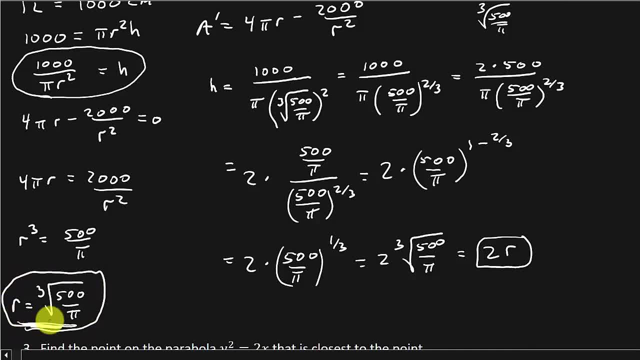 height and there is your radius. okay, Now, where did the r come from? Well, what's r? It's the cube root of 500 over pi, and I just replaced the cube root of 500 over pi with r, all right. 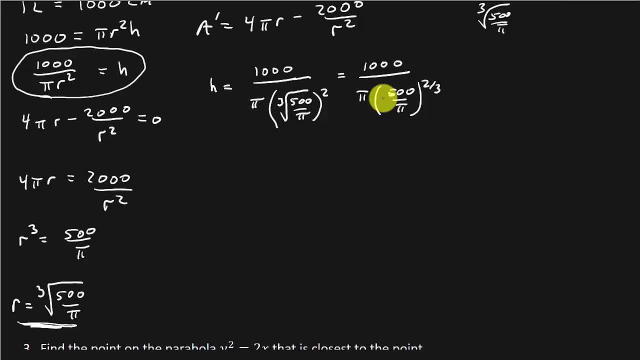 simplify this a little more. all right, so I noticed the thousand. I can write it down, and I can write it down, and I can write it down, and I can write that as 2 times 500, and that's over pi times 500, over pi to the two-thirds, and 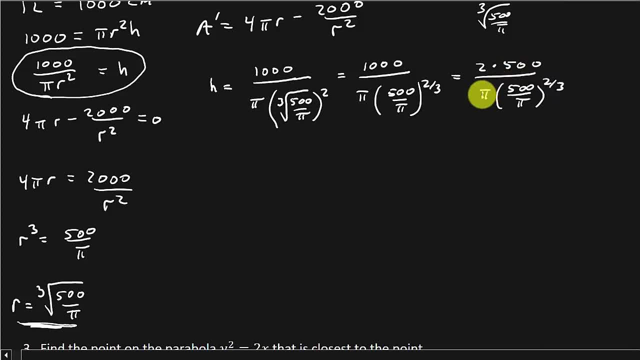 then if I separate this out, you see, you see this 500 over pi here and then this 500 over pi to the two-thirds. let's write this as 2 times 500 over pi over 500 over pi, pi to the two-thirds. all right, so this right here is the same thing as this: 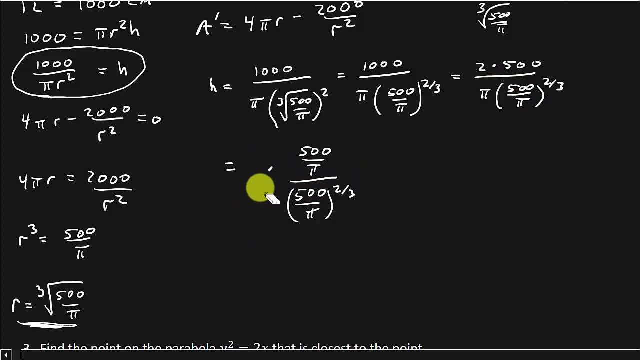 okay, I just separated it out. I've got the two away from at the two out here. and then this 500 over pi, this 500 and this pie. just wrote it up here in the numerator. well, this is two times and that's going to be 500 over pi to the. 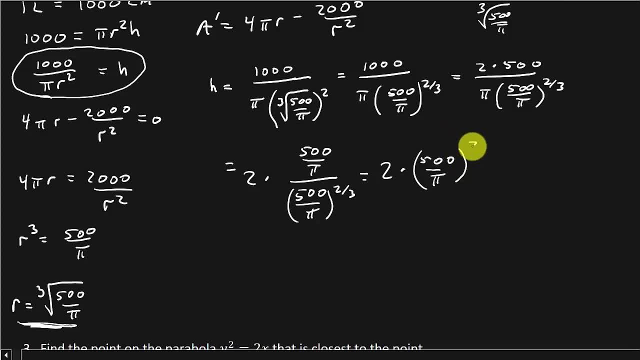 what? to the one minus two-thirds, which that's going to be two times 500 over pi, to the one-third, which is going to be two times the cube root of 500 over pi, and so I can actually write the height as what two are. okay. 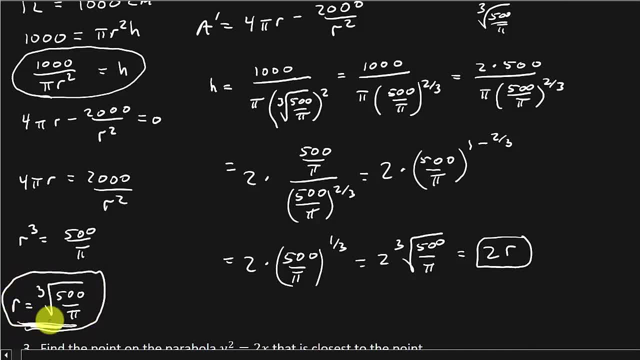 there's your height and there is your radius. okay now, where did the R come from? well, what's R? it's the cube root of 500 over pi, and I just replaced the cube root of 500 over pi with R. all right, so hopefully, that example, hopefully that. 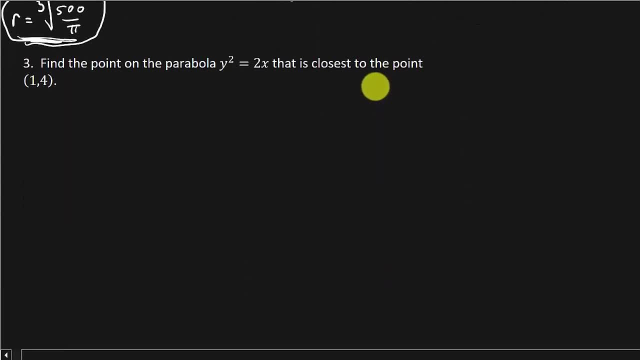 made sense. all right, let's look at this one we've got. it says: find the point on the parabola: y squared equals 2x. that is closest to the point one four. all right, so let's see what we've got here. so first thing we 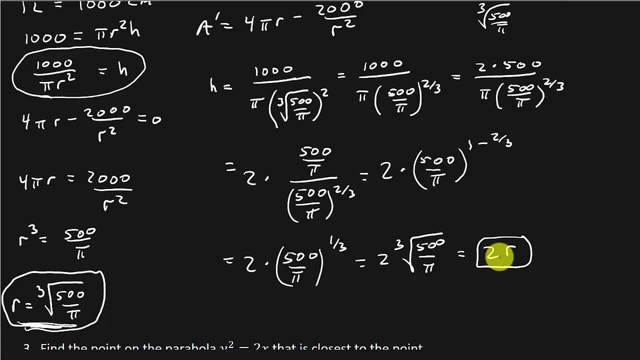 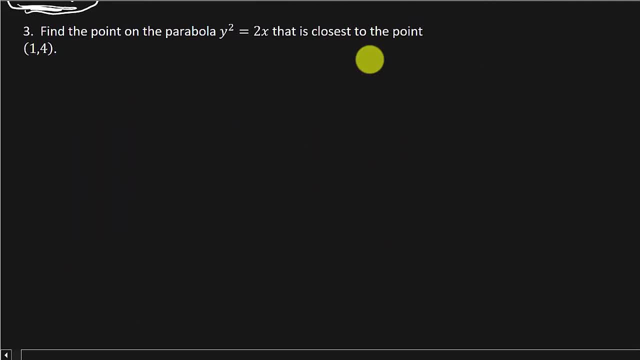 All right. so hopefully that example, hopefully that made sense. All right, let's look at this one. We've got it says: find the point on the parabola, y squared equals 2x that is closest to the point 1,, 4,. all right, So let's see what we've got here. So, first thing, 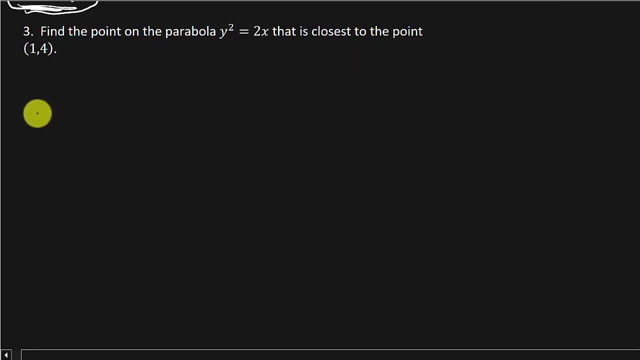 we want to do is: let's sketch, Let's sketch the graph. And you know, when you sketch this, it doesn't have to be. you know, you don't have to just draw it exactly, you know, just sketch it close, And so we. 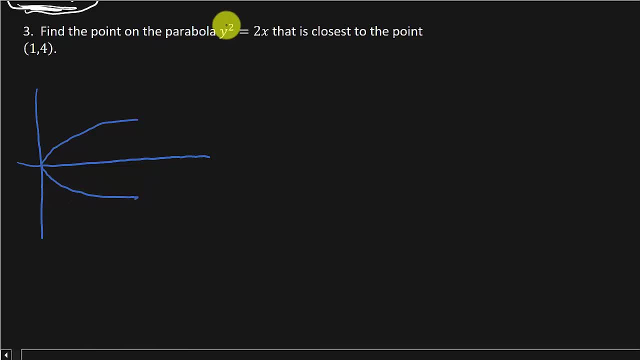 know this is a parabola that's going to open to the right. We've got the y squared here and our point 1, 4 is going to be up here. That's 1, 4.. We want to find a point on this graph that's closest to that point, right there, You see. 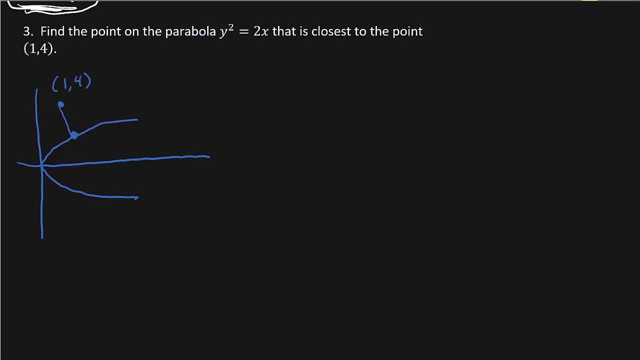 that That's closest to that point. All right, so let's think about this for just a second. Well, here's my point x y. okay, Some point x y on the graph. What's that point? I don't know. okay, That's what we're going to figure out, But what do we want to do? 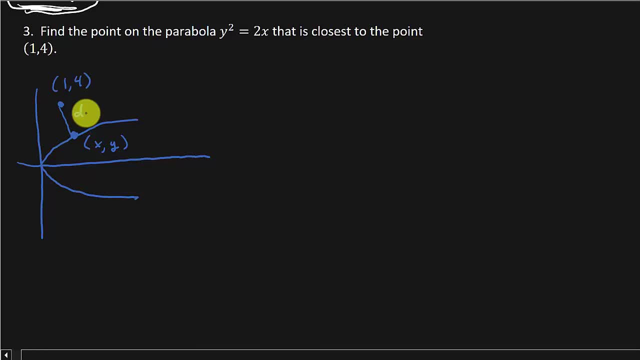 We want to minimize this distance here. okay, That's what it's asking for. Find the point on the parabola that is closest to the point 1, 4.. So we want this distance to be a minimum. So, if you remember back from algebra, if you have, 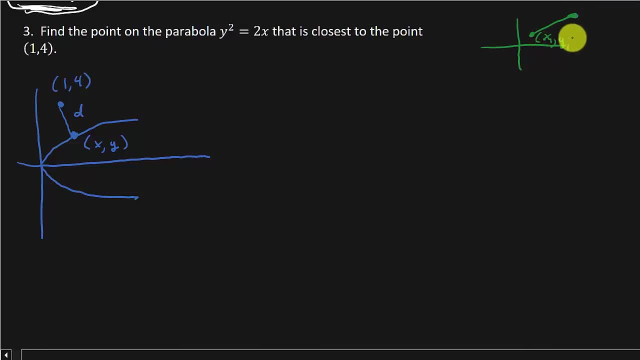 two points on a graph, say x1, y1, and x2, y2.. Remember, the distance between the two points is x2 minus x1 squared, plus y2 minus y1 squared. okay, That's the distance between two points. 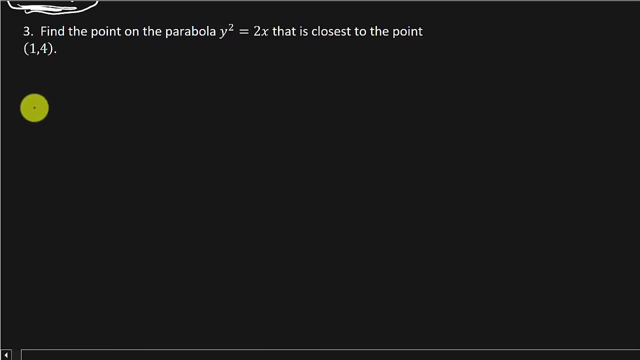 want to do is: let's sketch, let's sketch the graph, and, and you know, when you sketch this, it doesn't have to be, you know, you don't have to just draw it exactly, you know, just sketch it close. and so we know this is a parabola, that that's. 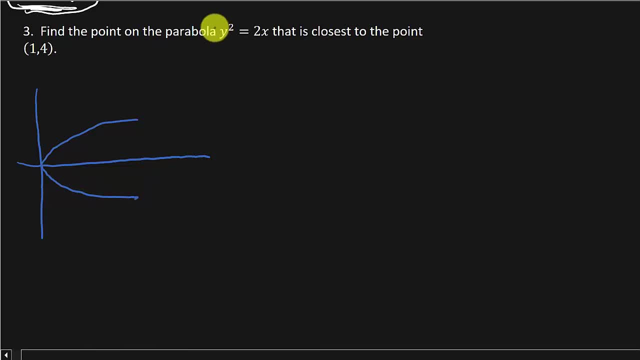 going to open to the right. we got the y squared here and our point one four is going to be up here. that's one for this. we want to find a point on this graph that's closest to that point, right there. you see, that's the point that's closest to that point, right there. 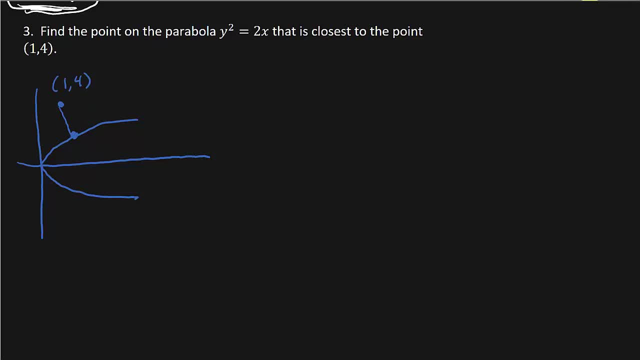 that that's closest to that point. all right, so, so let's, let's think about this for for just a second. well, here's my point X Y. okay, some point X Y on the graph. what's? what's that point? I don't know. okay, that's what we're gonna what. 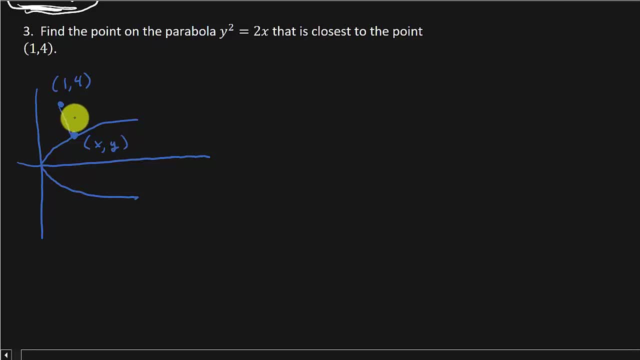 we're gonna figure out. but what do we want to do? we want to minimize this distance here. okay, that's what it's asking for. find the point on the parabola that is closest to the point one four. so we want this distance to be a. 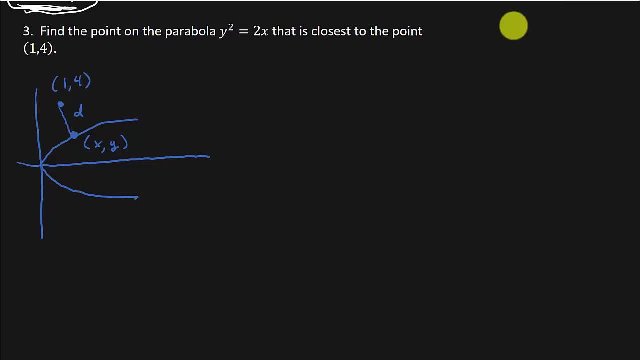 minimum. so if you remember back from algebra, if you have two points on a graph, say X 1, Y 1 and X 2, Y 2, remember the distance between the two points is X 2 minus X 1 squared plus Y 2 minus Y 1 squared. okay. 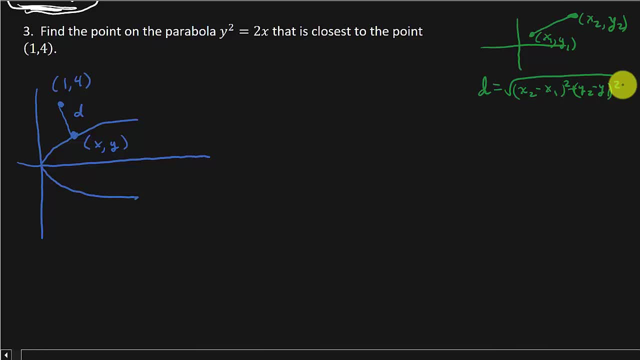 that's the distance between two points. so let's do X 2 minus X 1 plus Y 2 minus Y 1, so the distance we have is the square root of X 2 minus x1 squared, plus what y2 minus y1 squared. okay, I'm just calling. I'm. 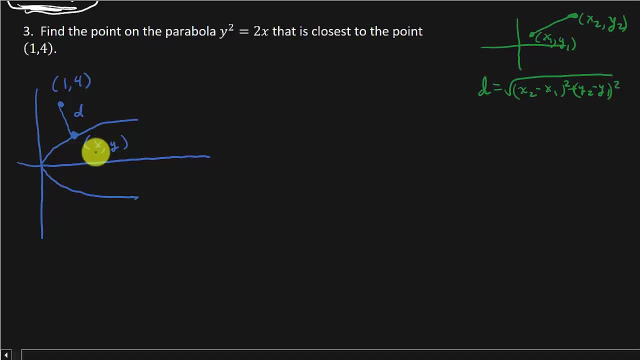 So let's do x2 minus x1 plus y2 minus y1.. So the distance we have is the square root of x2 minus x1 squared, plus what y2 minus y1 squared. okay, I'm just calling. I'm calling this x2, y2, and I'm calling this one x1, y1.. 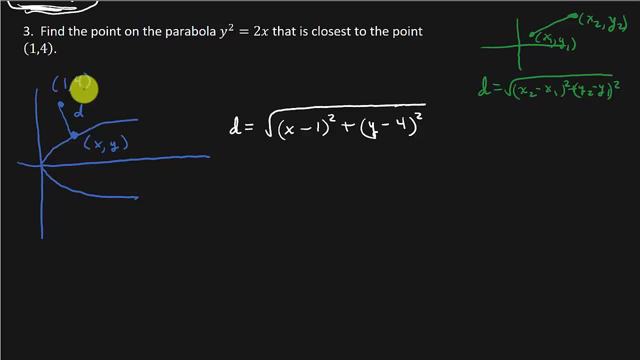 And now we're going to what? We're going to take the derivative, But before I take the derivative, okay, Before I take the derivative, what do I need to do? okay, What do I need to do? Well, I want to get everything in terms of one variable. I want to get everything in terms of x. 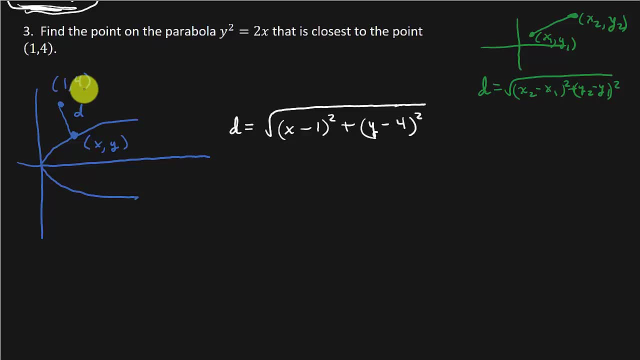 or everything in terms of y. Well, in this problem, I think it, I think it might probably be easier if we got everything in terms of y. Let's do that, So I would have. the distance is equal to the square root of 1 half y squared. 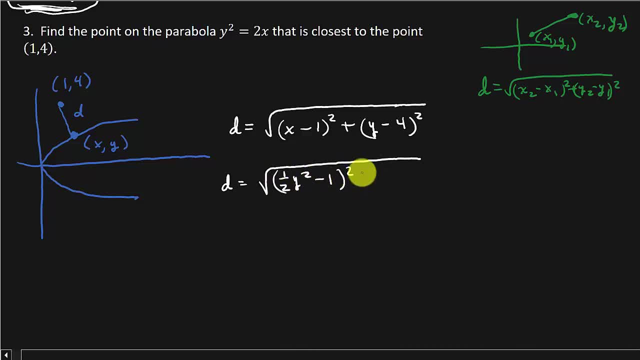 minus 1 squared. okay. So well, where did that come from? Well, you can see here: x is equal to 1 half y squared, So okay, so x is equal to 1 half y squared, minus 1 squared. Well, you can see here: x is equal to 1 half y squared. 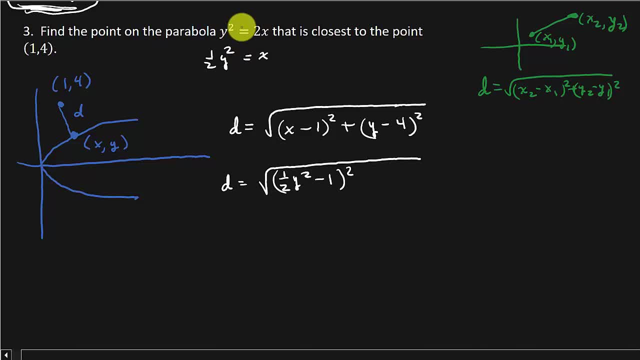 squared. okay, based on the our function here or our equation we have up here, y squared equals 2x. so I'm just replacing the X, but this one-half y squared, and then that's plus y, and then that's plus y minus 4, and then all of that squared. 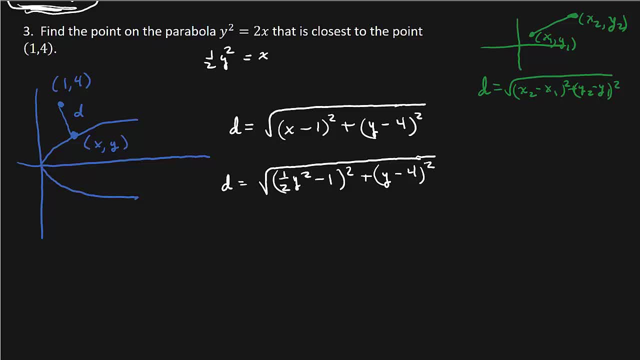 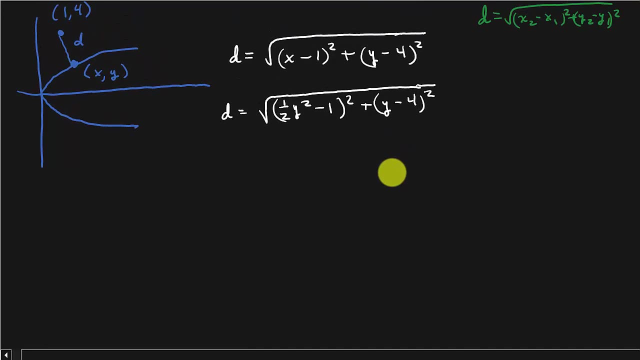 all right. so what do we need to do now? we need to take the derivative right. all right, so to take the derivative there's. I don't know if you've watched a lot of my videos, but I have a video out on shortcut for finding the derivative. 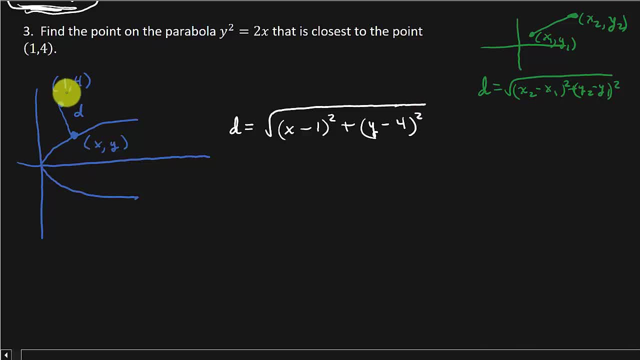 calling this x2- y2, and I'm calling this one x1- y1. and now we're gonna what? we're gonna take the derivative. but before I take the derivative- okay, before I take the derivative- what do I need to do? okay, what do I need to do? well, I want to get. 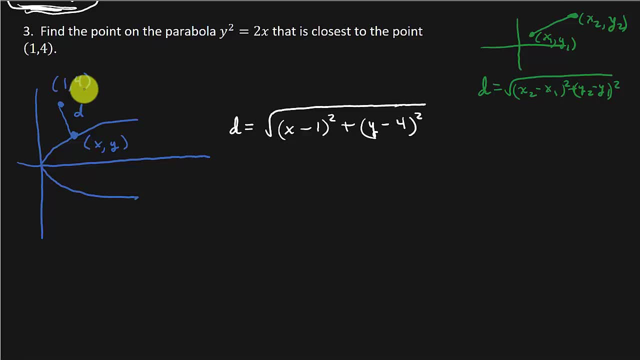 everything in terms of one variable. I want to get everything in terms of X or everything in terms of Y. well, in this problem, I think it. I think it might probably be a little bit complicated, but I think it might be a little bit easier if we got everything in terms of Y. let's do that, so I would have the 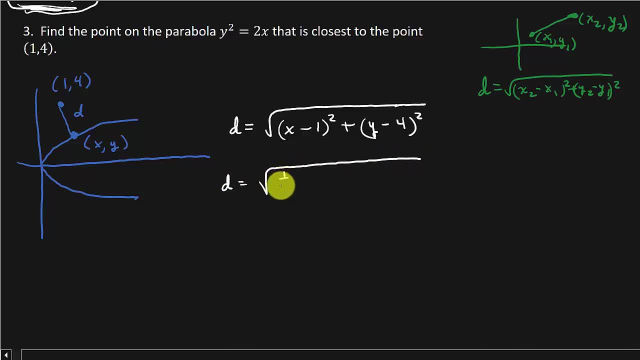 distance is equal to the square root of 1 half y squared, minus 1 squared. okay, so well, where did that come from? well, you can see, here X is equal to 1 half y squared. okay, based on the our function here, or our equation we have up here: y squared equals 2x. so I'm 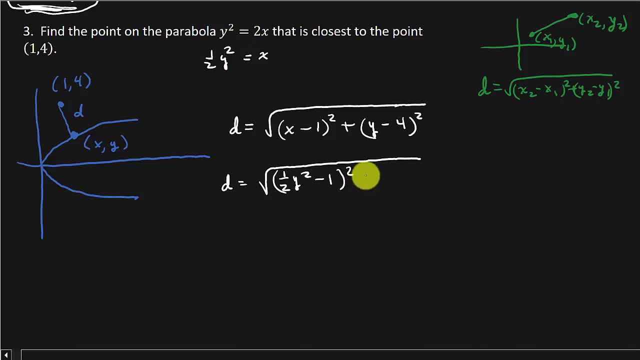 just replacing the X with this: 1 half y squared, and then that's plus y, and then that's plus y minus 4, and then all of that squared, all right. so what do we need to do now? we need to take the derivative right, all right. so to take the derivative there's- I don't know if you've. 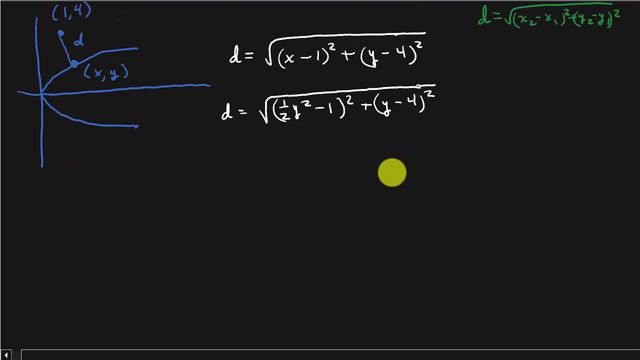 watched a lot of my videos, but I have a video out on shortcut for finding the derivative of a square root. so what you can do- and I'm going to just do it right here- D prime is equal to all right, so look at this. so the derivative of a square root. there's a shortcut. single pneuval function can x, x and y can be a short cut. if you keep parents, even if you continue to watch classes, you're going to occasionally get error reviews. we're also going to have peuvent t. we're subtopics. we're going to have problems with terms of this integral. 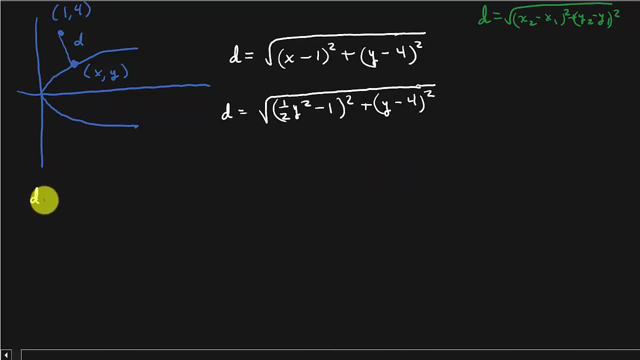 of a square root. so what you can do, and I'm going to just do it right here: D prime is equal to all right, so look at this. so the derivative of a square root. there's a shortcut: it's just 2 times the square root of 1 half y squared, minus 1 squared. 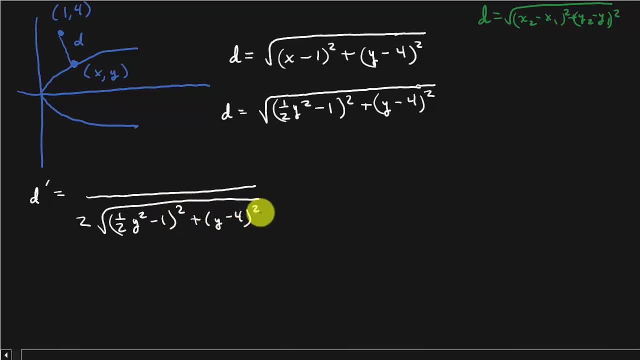 plus 1 minus 4 squared. so whenever you're taking the derivative of a square root, it's 2 times, whatever your square root is. okay, that's. that goes in the denominator every time, and then what goes in the numerator is the derivative of what's. 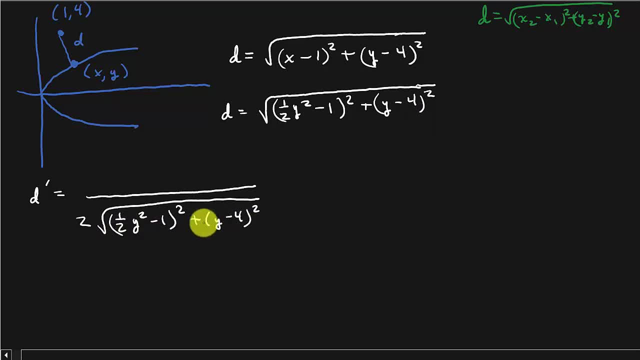 underneath the square root. so what's the derivative of what's underneath the square root? well, I've got chain rule here right, so the 2 comes down times 1, half y squared minus 1, subtract 1 from the exponent. so that's to the first. 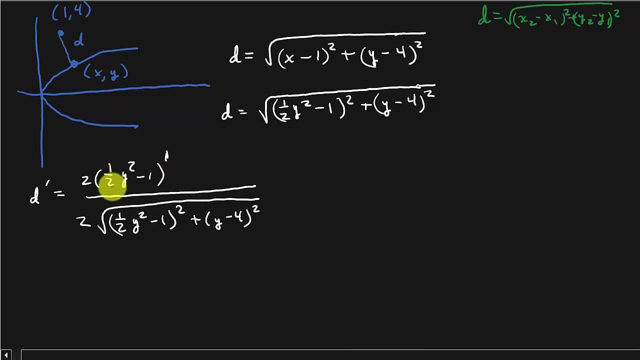 power times, the derivative of what's inside the parentheses, which in this case is just y, and then plus chain rule, again 2 y minus 4, that's to the first power times, the derivative of what's inside the parentheses, which is 1. all right, and so. 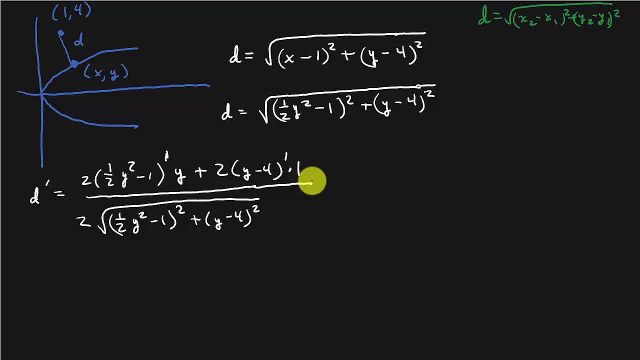 now all I need to do is just distribute, you know, distribute clear the parentheses here combined like terms, if I can. so so let's see what we get. so this is going be, this is going to be y cubed, right, let's see? yeah, y cubed minus. 2y plus, 2y minus. 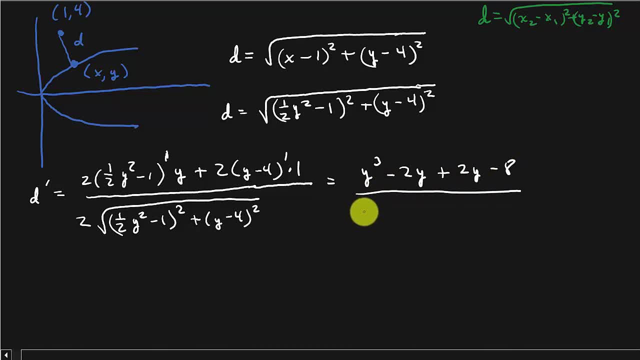 8, over 2 square root of 1 half y squared minus 1 squared plus y minus 4 squared. alright, alright. so this is going to give us d prime. is well, that worked out nice, didn't it? y cubed minus 8 over 2 square root. 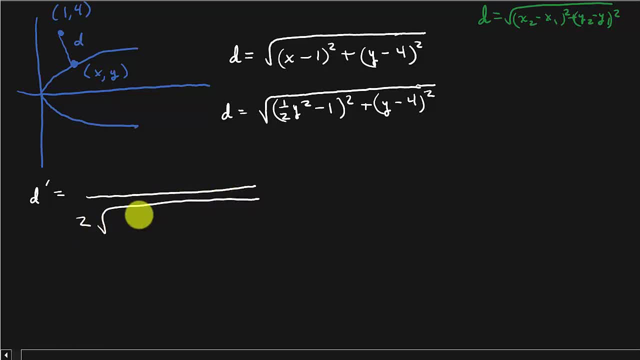 and how things. second term right, all right. so I want this to be 1 half y Q. It's just 2 times the square root of 1 half y squared minus 1 squared plus y minus 4 squared. So whenever you're taking the derivative of a square root, it's 2 times, whatever your square root is. 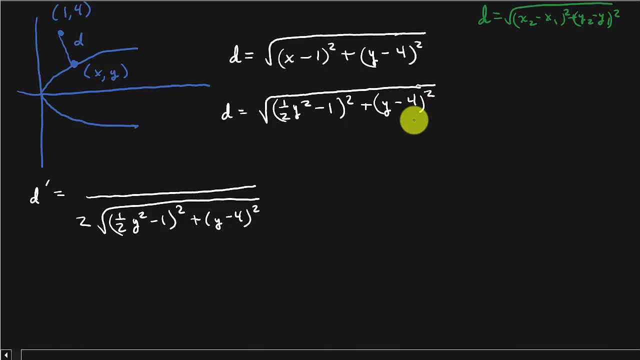 Okay, that goes in the denominator every time. And then what goes in the numerator is the derivative of what's underneath the square root. So what's the derivative of what's underneath the square root? Well, I've got chain rule here, right? 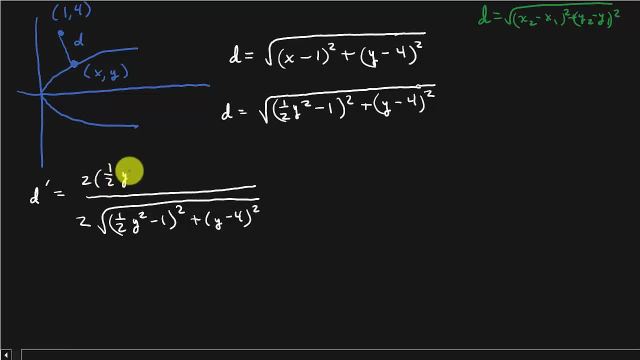 So the 2 comes down, times 1, half y squared minus 1.. Subtract 1 from the exponent, so that's to the first power times, the derivative of what's inside the parentheses, which in this case is just y. Okay. 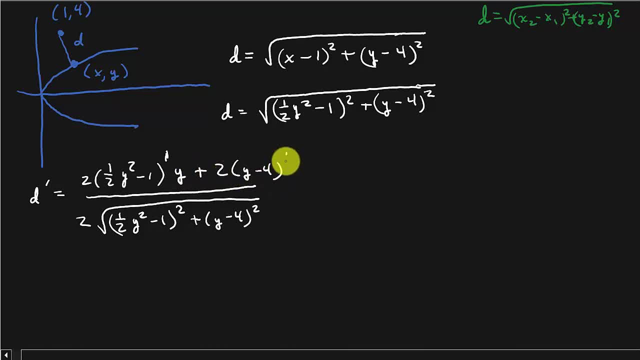 And then plus chain rule, again 2y minus 4, that's to the first power times, the derivative of what's inside the parentheses, which is 1.. All right, And so now all I need to do is just distribute, you know, distribute, clear the parentheses here. 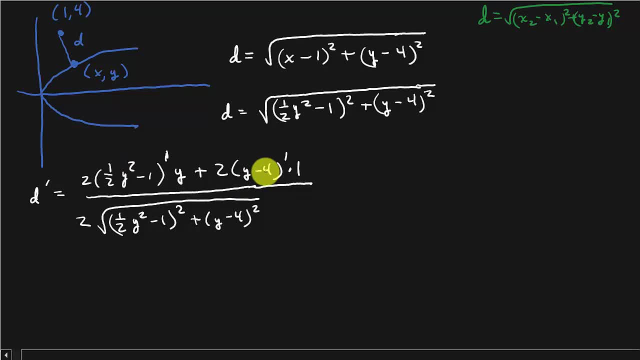 combine like terms, if I can. So let's see what we get. So this is going to be, this is going to be y cubed, right? Let's see? Yeah, y cubed minus 2y plus 2y minus 8. 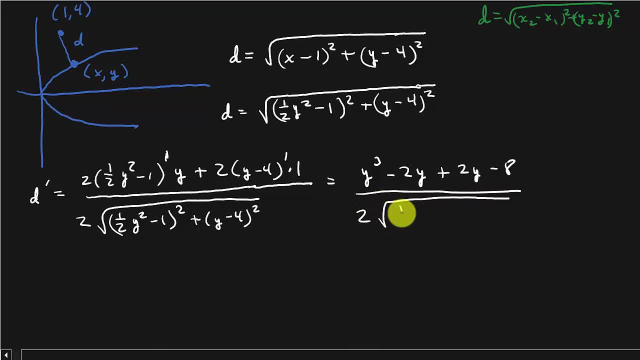 over 2 square root of 1 half y squared: Square root minus 1 squared plus y minus 4 squared. All right, All right. So this is going to give us d prime. is well, that worked out nice, didn't it? 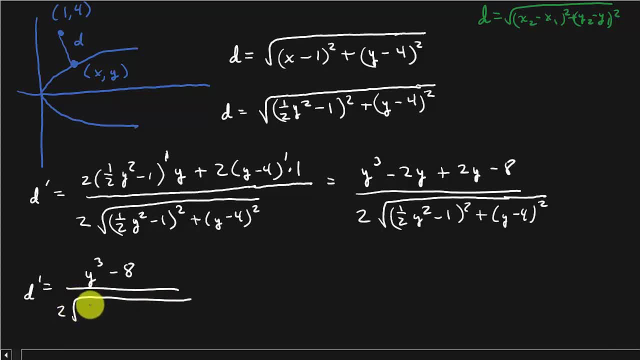 y cubed minus 8 over 2 square root. 1 half y squared minus 1 squared. plus y minus 4 squared. All right, Now what do we want? What do we want now? Well, remember, you've got to set this equal to 0 and solve for, in this case, y. 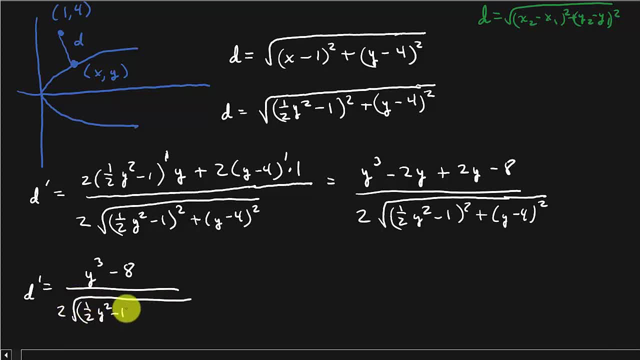 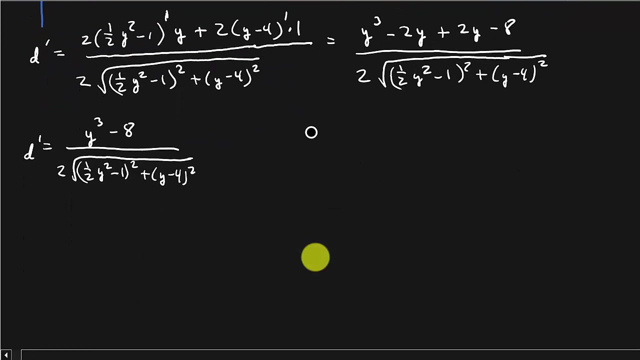 1 half y, squared minus 1, squared plus y minus 4, squared. alright, now, what do we want? what do we want now? well, remember, you got to set this equal to 0 and solve for, in this case, y. alright, so we know that a fraction is 0,. 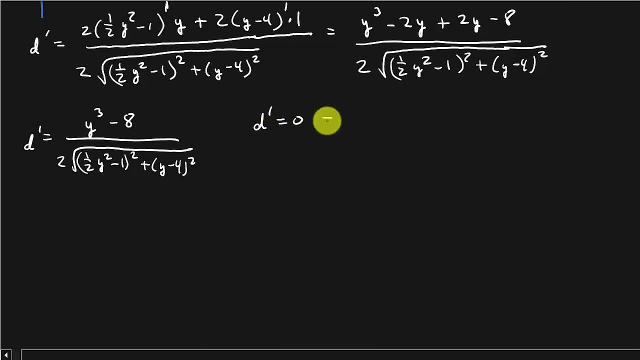 okay, so we know d prime is 0 when y cubed minus 8 is 0, so y cubed equals 8 and y equals 2, alright, so so look, you can test this, you can put the 2, we can, we can do x equal 1,. 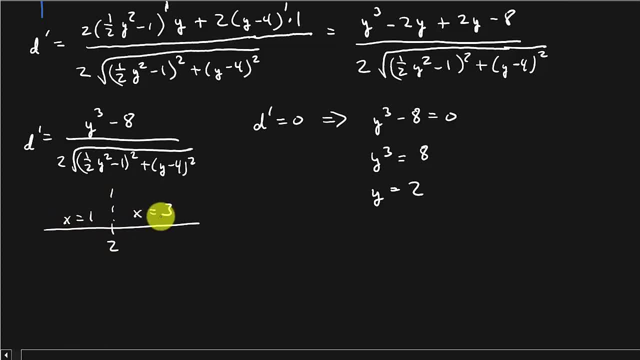 we can do x equal 3, and just keep in mind the denominator is going to always be positive. so if we plug the 1 in, that's going to give us a negative. if we plug the 3 in, that's. 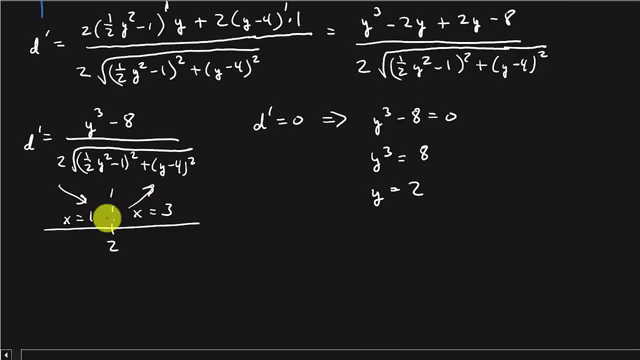 going to give us a positive, and you can see: y equals 2 is a minimum, okay, and so this is the y coordinate of the point we're looking for. well, now we want what. We want: the x coordinate of the point. well, what was our? 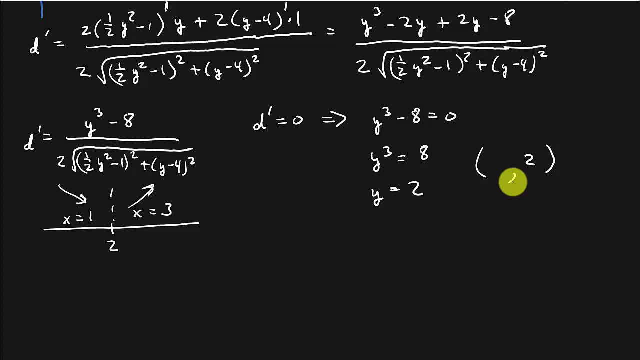 let's see: our function was y squared equals 2x. so if I plug the 2 in for y squared, that's going to be 2 squared equals 2x. so we get X is equal to 2, and so that's the point. that's the closest. this is the point on the parabola, that's. 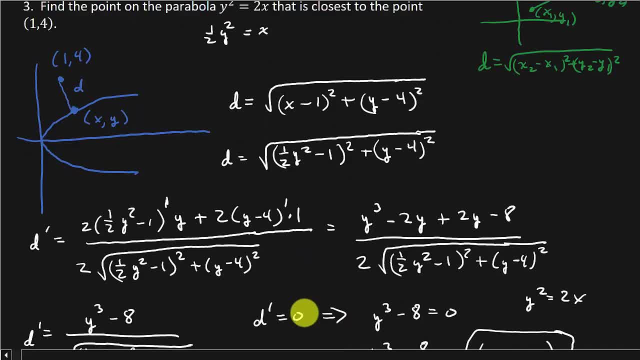 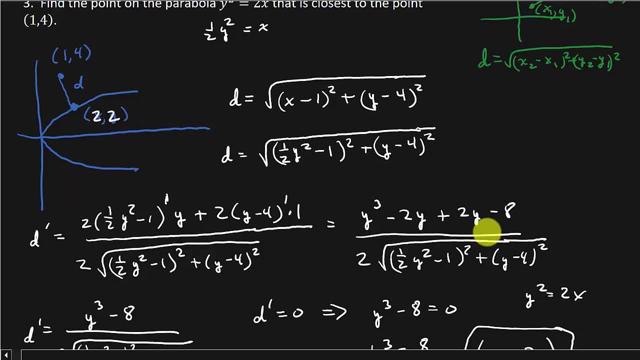 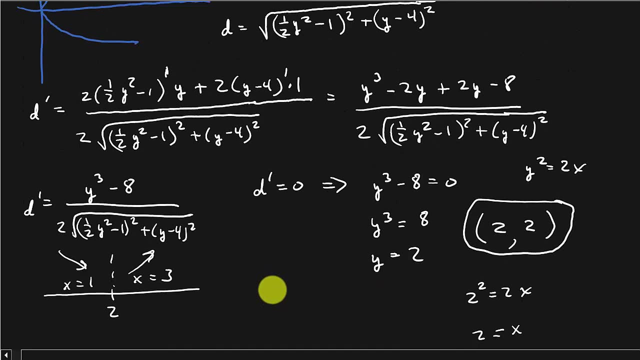 closest to the point one. four: okay, that would be this point here. this would be the point two. two, all right, so you know that it wasn't too bad. I mean it. it got a little messy on the derivative, but it's not bad, I mean, you know, luckily it. 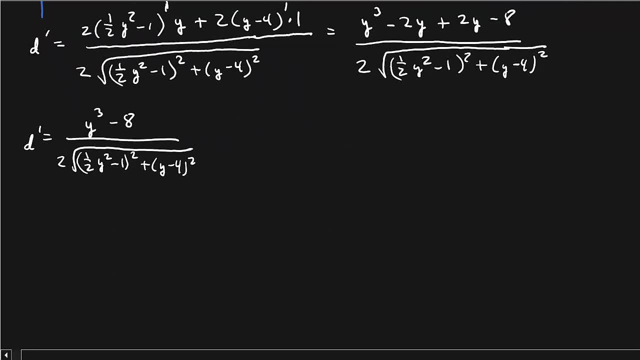 All right, So we know that a fraction is 0.. Okay, So we know d prime is 0 when y cubed minus 8 is 0. So y cubed, y cubed equals 8 and y equals 2.. 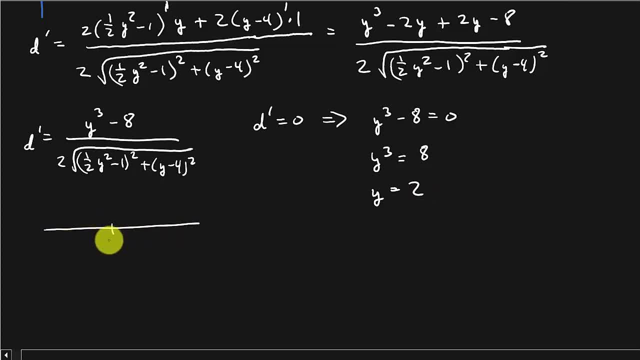 All right. So so look, you can test this. You can put the 2.. We can. we can do x equal 1.. We can do x equal 3.. And just keep in mind, the denominator is going to always be positive. 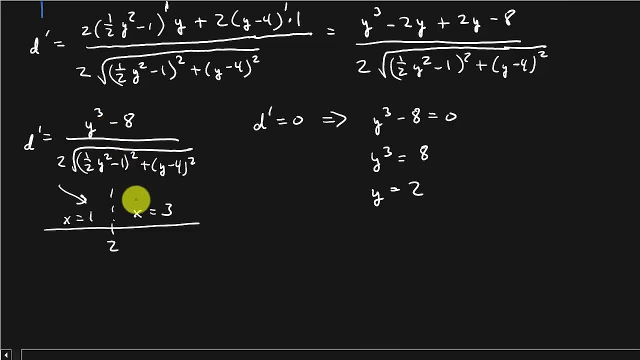 So if we plug the 1 in, that's going to give us a negative. We plug the 3 in, that's going to give us a positive. And you can see: y equals 2 is a a minimum, Okay, And so this is the y coordinate of the point we're looking for. 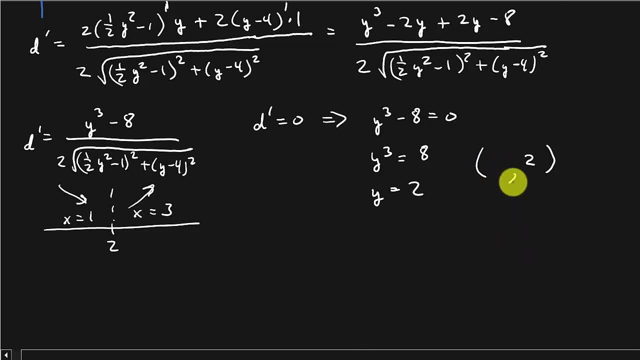 Well, now we want what. We want: the x coordinate of the point. Well, what was our function? Let's see. Our function was: y squared equals 2x. So if I plug the 2 in for y squared, that's going to be 2 squared equals 2x. 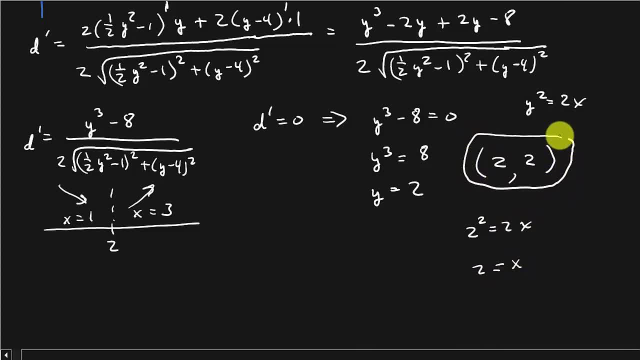 So we get: x is equal to 2.. And so that's the point That's the closest. This is the point on the parabola that's closest to the point 1, 4.. Okay, That would be this point here. 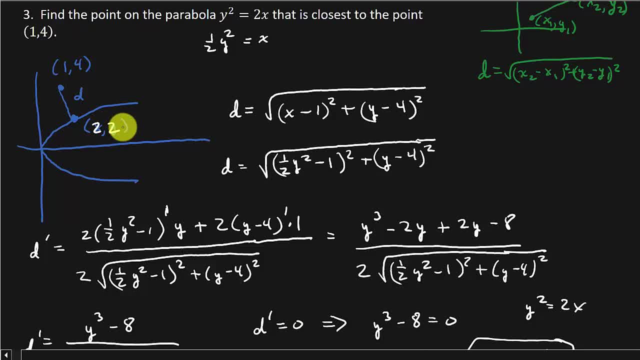 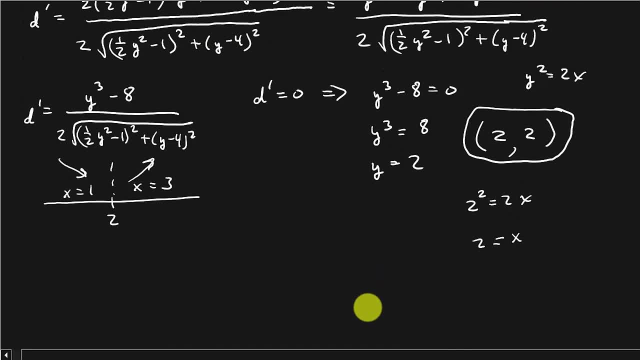 This would be the point 2, 2.. All right, So you know that it wasn't too bad. I mean it. it got a little messy on the derivative, but it's it's not bad. I mean, you know, luckily it came out like this: 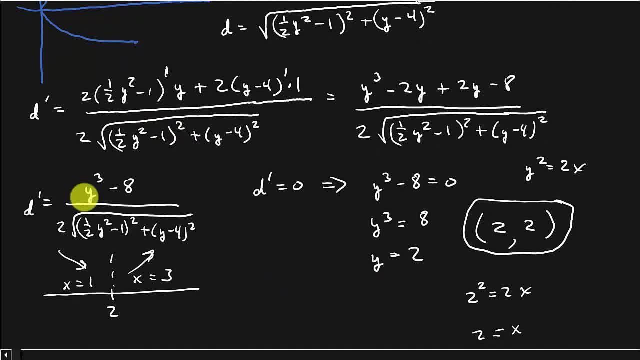 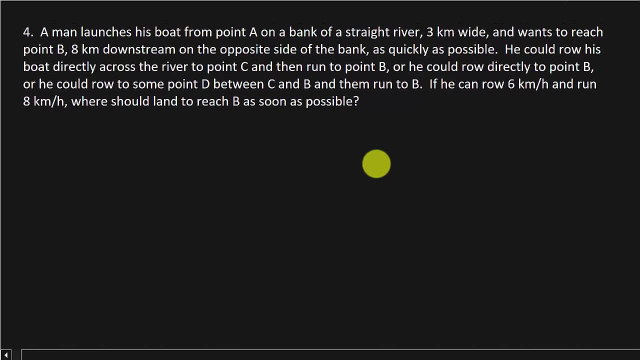 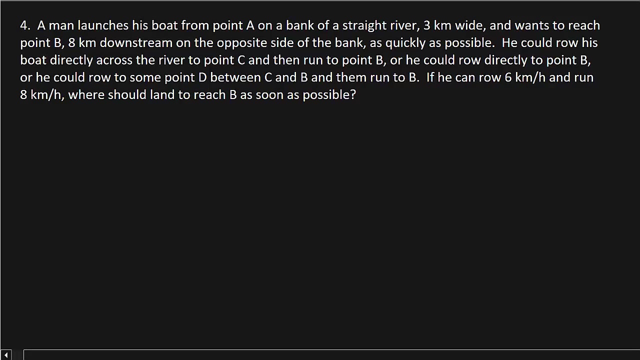 This made it nice there. And then, of course, a fraction is just 0 when the numerator is 0. So we didn't have to worry about the denominator. All right, What about this one? All right. So for this example we have: a man launches his boat from point A on the bank of a straight 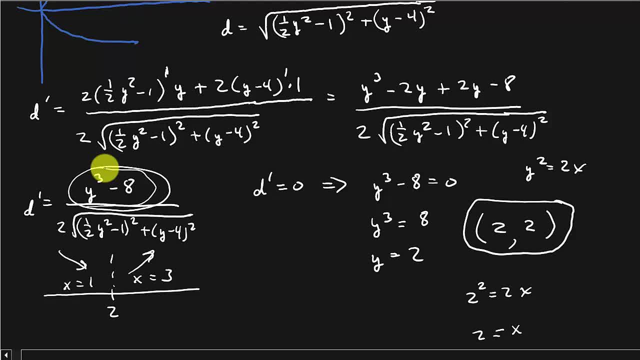 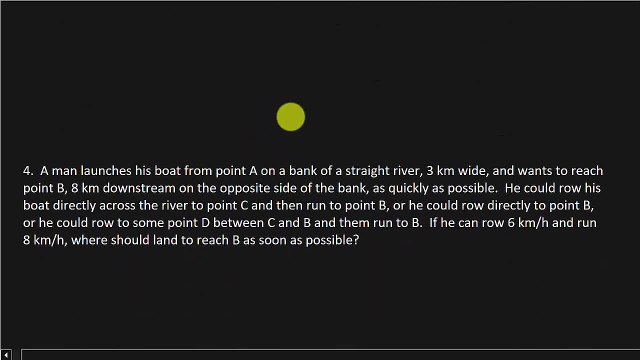 came out like this: this made it nice there. and then, of course, a fraction is just zero when the numerator is zero. you know, luckily it came out like this: this made it nice there. and then, of course, a fraction is just zero when the numerator is zero, so we didn't have to worry about the denominator. all right, what about this? 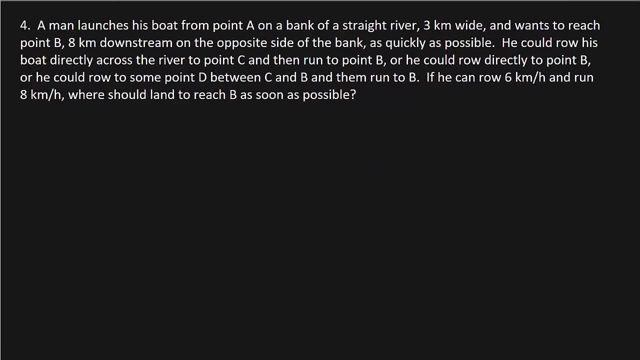 one, all right. so for this example we have, a man launches his boat from point a on the bank of a straight river three kilometers wide, and wants to reach point B, eight kilometers downstream, on the opposite side of the bank. as quickly as possible he could row his boat directly across the river to point C and then run. 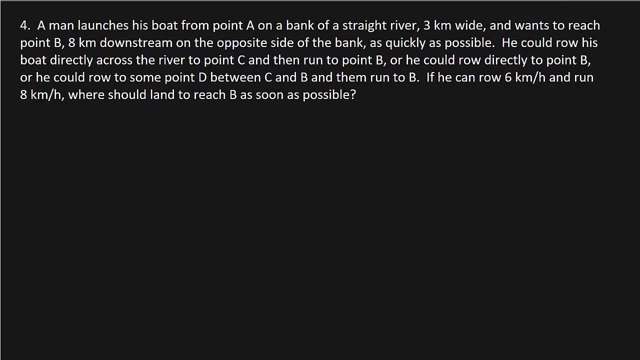 to point B, or he could row directly to point B, or he could row to some point D between C and B, and then that should be then there and then run to B. if he can row six kilometers an hour and run eight kilometers an hour, where should he land? 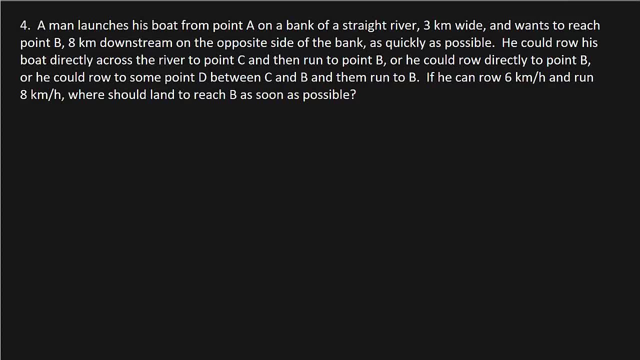 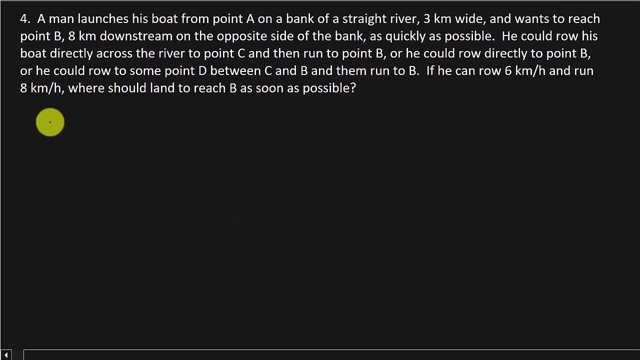 to reach B as soon as possible. so the best thing here is going to be to draw a picture. so if we see, all right. so if we draw the river and he launches his point, his boat, from point a and we know that the river is three kilometers wide and he 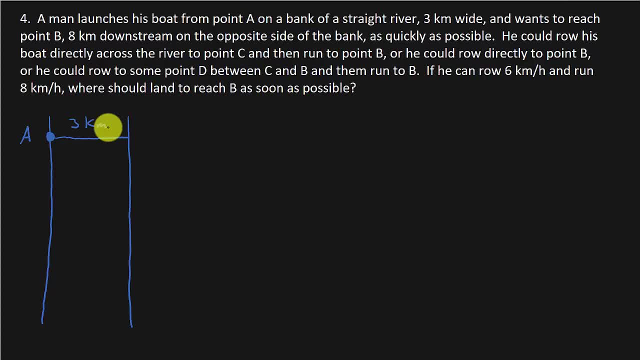 wants to reach a point B, eight kilometers kilometers downstream, on the opposite side of the bank. so that would be a point B right here and it is eight kilometers downstream, all right. so it says he could row his boat directly across the river to point C. so that means he would be going straight across. 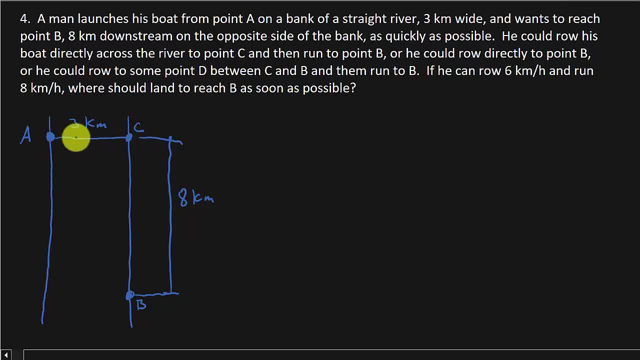 to some point C and then. so he could row straight across and then run down, or he could row directly to B, so that's from a directly to B. he does nothing but row. or he could row to some point D, which we'll call this D here. that's between C and B. 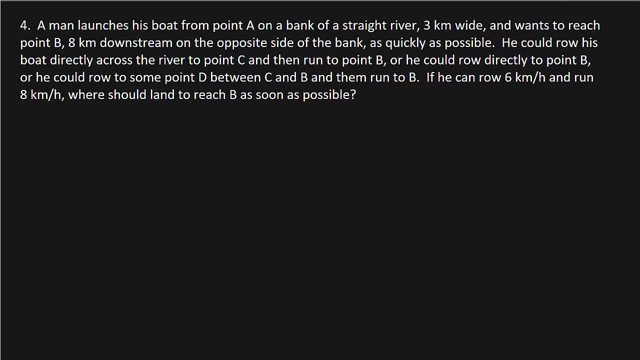 river three kilometers wide, and wants to reach point B, eight kilometers downstream on the opposite side of the bank, as quickly as possible. Okay, That's a good one. He could row his boat directly across the river to point C and then run to point B. 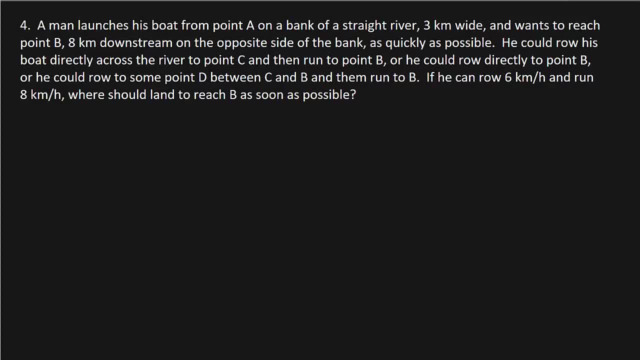 or he could row directly to point B, or he could row to some point D between C and B, and then that should be then there- and then run to B. If he can row six kilometers an hour and run eight kilometers an hour, where should he land? to reach B as soon as possible? 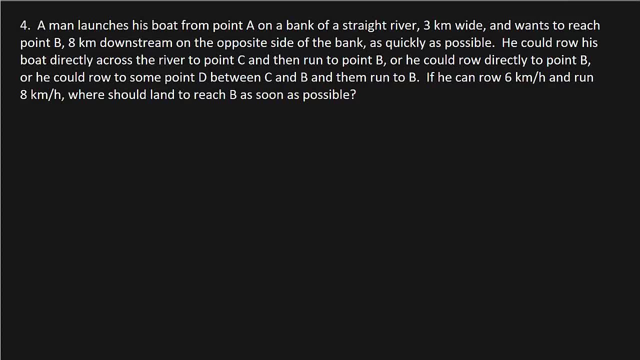 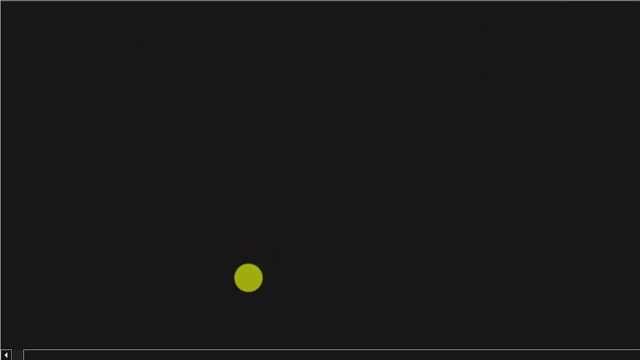 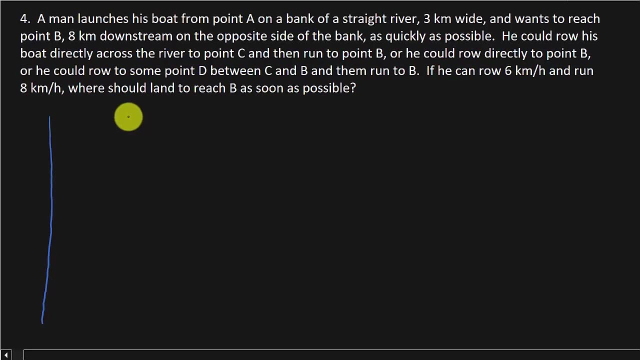 So the best thing here Is going to be to draw a picture. So if we, what happened there, let's see, all right. So if we draw the river and he launches his point, his boat, from point A and we know, 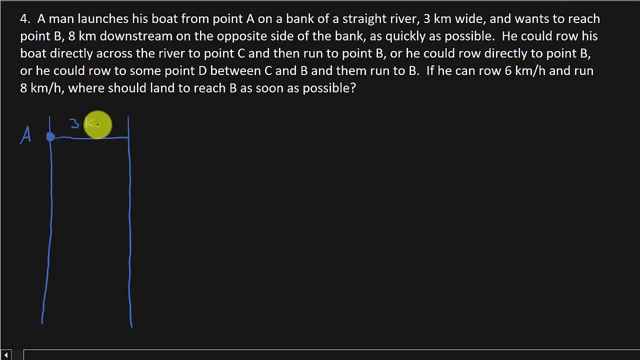 that the river is three kilometers, Three kilometers wide, And he wants to reach a point B eight kilometers downstream, on the opposite side of the bank. So that would be a point B right here And it is eight kilometers downstream, All right. 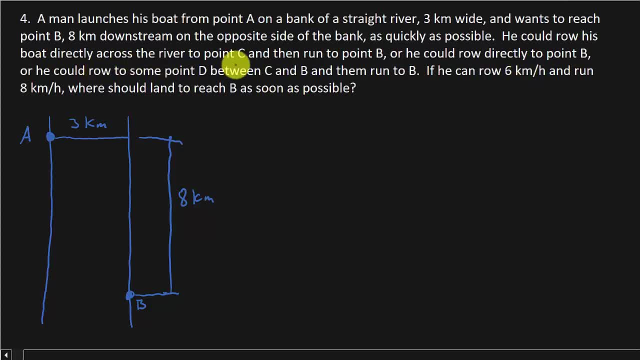 So it says he could row his boat directly across the river To point C. so that means he would be going straight across to some point C And then so he could row straight across and then run down, or he could row directly to B. So that's, from A directly to B. He does nothing but row, or he could row to some point. 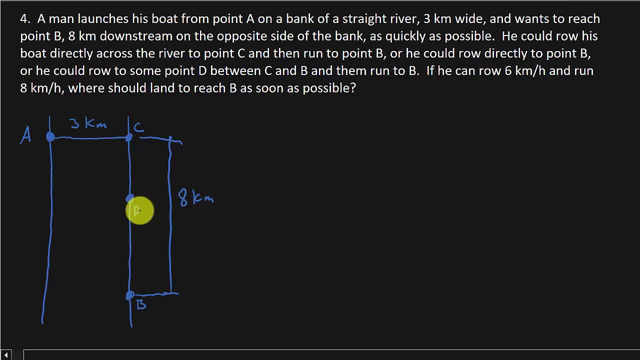 D, which we'll call this D here. That's between C and B, But the point B- he should not be going straight across the river Right and then run to b, all right, so. so how far would this point need to come down? 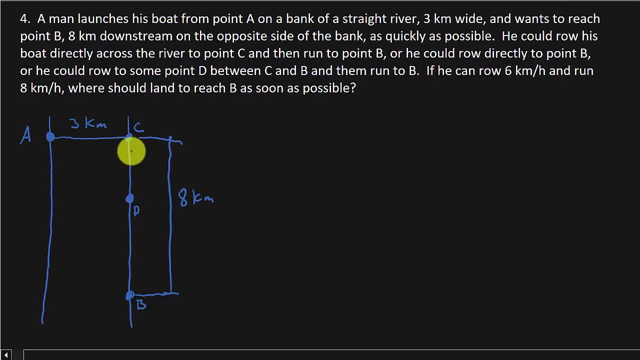 and then run to B, all right, so. so how far would this point need to come down? well, let's see if we can figure that out. we'll call that X, and so we know this distance here is 8 minus X, all right, so what we want to do is we want to minimize the time, right, we want the we. 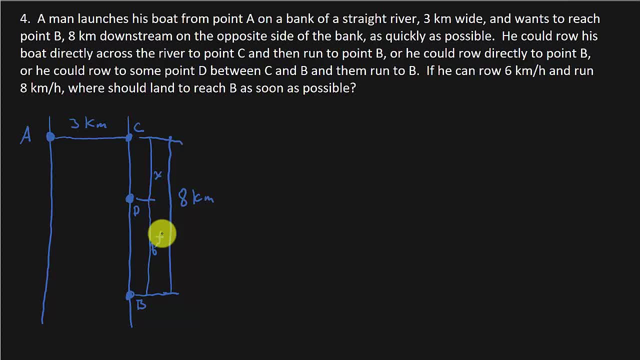 want the shortest time. well, how are we going to do this? well, we know that distance is equal to rate, times, time, which tells us that time is equal to distance over rate. all right, so that's what we're trying to minimize this time. so we need, we need- distance. 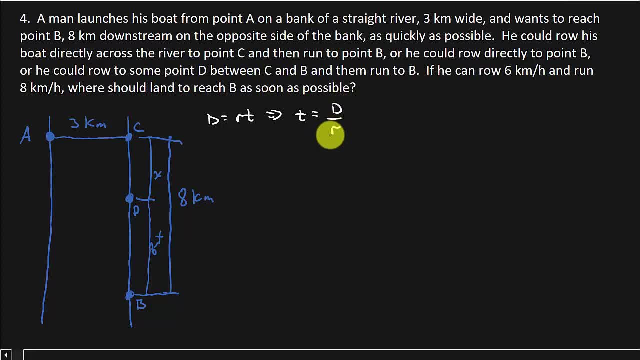 and we need the rate, all right. so if we, if we draw a line from A to D, all right, what would that mean? if we're drawing to our distribuion line, the distribution center would be taking a line frequency equal to that. and if we're drawing a line from X to D, what 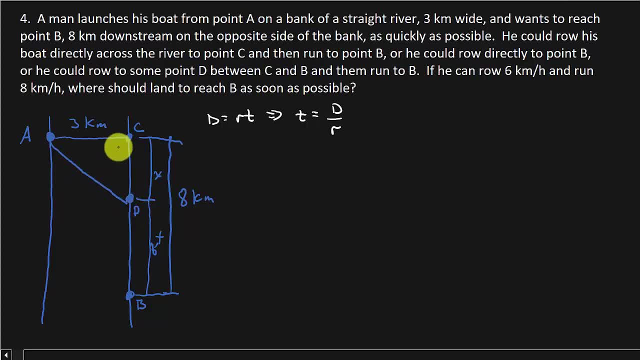 does that mean? well, before we know this, we don't know that, but we're going to call this- would this distance here be from A to D? Well, remember, this is a right triangle, so this side here would be x squared plus 9, right? So if we write down rowing the time it takes, 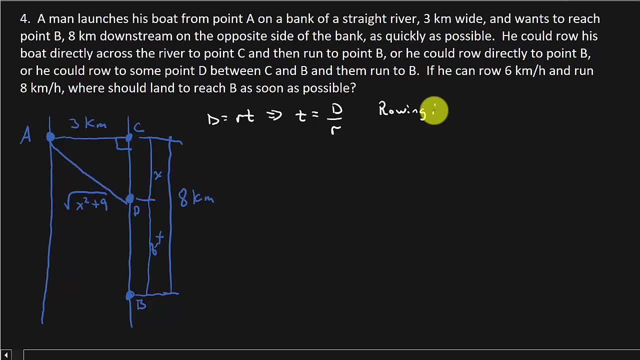 him to row. that would be what? The distance, which is this distance here, from A to D, which is the square root of x, squared plus 9, over the rate. Well, how fast does he row? He rows 6 kilometers per hour. So that's the time it's going to take him to row. Now, what about? 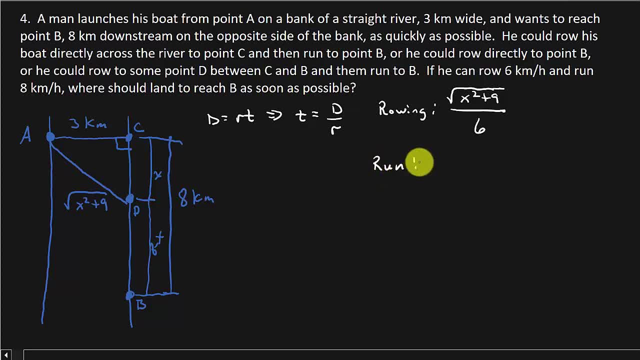 running. How long will it take him to run? Well? what's the distance he has to run? That would be 8 minus x over the rate that he runs. Well, he runs 8 kilometers per hour, So this is the time it takes him to row. this is the 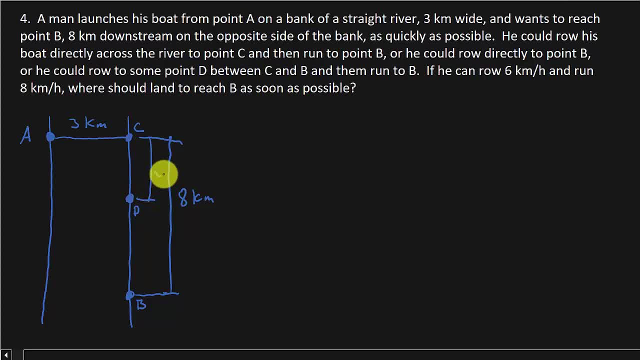 well, let's see if we can figure that out. we'll call that X, and so we know this distance here is 8 minus X. all right, so what we want to do is: we want to minimize the time. right, we want them, we want the shortest time. well, how are we going to? 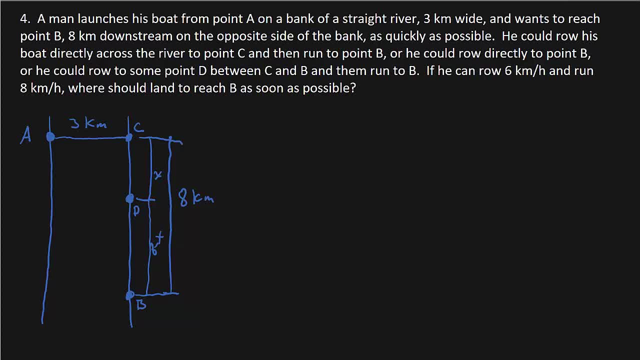 do that. well, we know that distance is equal to rate, times, time, which tells us that time is equal to distance over rate. all right, so that's what we're trying to minimize as time. so we need, we need distance, we need the rate, all right, so if we, if we draw a line from a to D, all right, 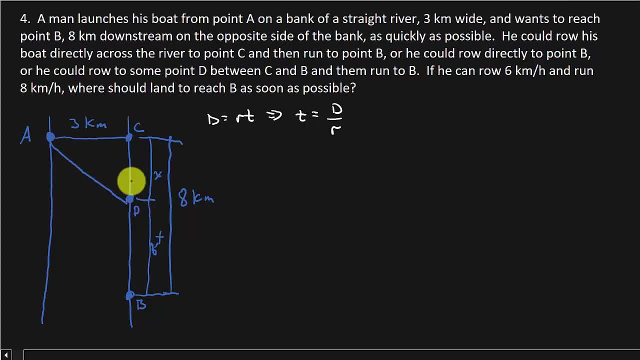 what would this distance here be from a to D? well, remember, this is a right triangle, so this side here would be x squared plus 9, right? so if we, if we write down roping the time it takes him to row, that would be what the distance, which is this distance here from a to D, which is the square root of 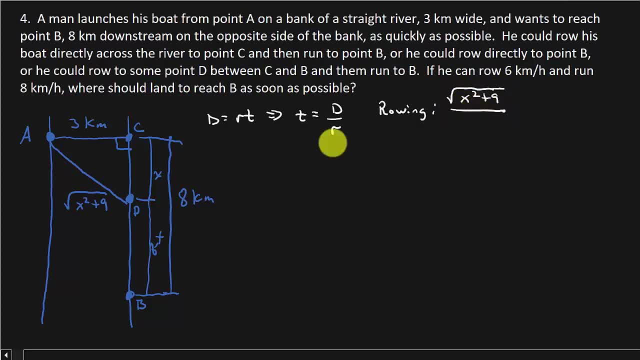 x squared plus 9 over the rate. well, how fast is he row? he rose six kilometers per hour. so that's the time it's going to take him to row. now what about running? how long will it take him to ruin? well, what's the distance he has to ruin? that would be 8 minus X over the rate that he runs. well, 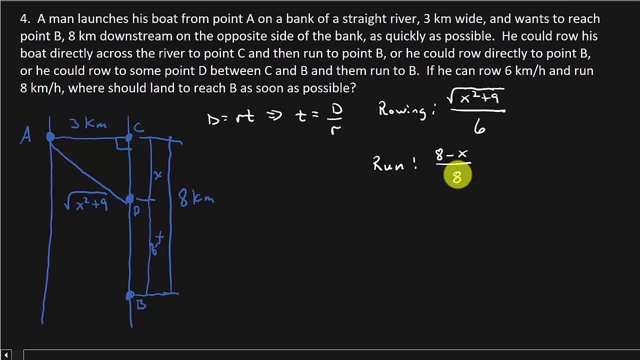 he runs 8 kilometers per hour, so this is the time it takes him to row, this is the time it takes him to run, so we need that total time. so we'll call that: T of X is equal to the square root of x squared plus 9 over. 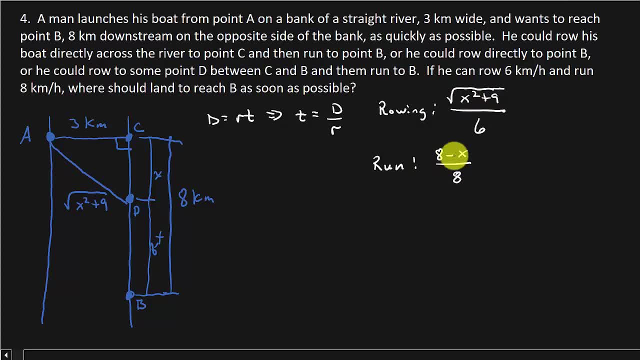 time it takes him to run. So we need that total time. So we'll call that: t of x is equal to the square root of x, squared plus 9, over 6, plus 8, minus x over 8.. All right, So there's our time, So we need to take. 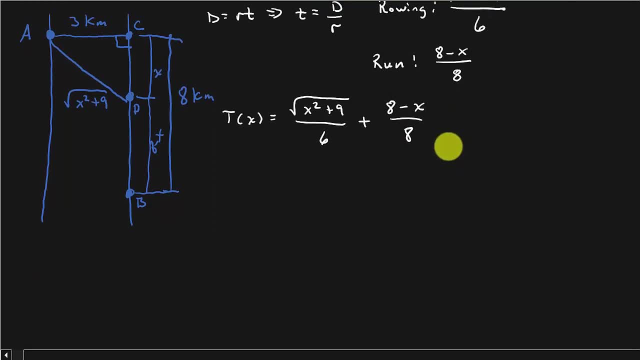 the derivative right. We need to take the derivative. But before we take the derivative, I want to do. I want to do something real quick. It'll make it a little bit easier to see how we take the derivative. So that's 1 sixth square root of x squared plus 9,. 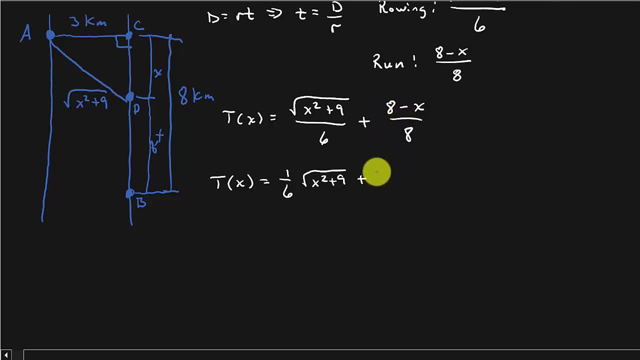 plus, and then this is 8 over 8, which is 1, minus 1 eighth x. I just split this fraction up, All right, So I think writing it like this it'll make it easier to take the derivative. 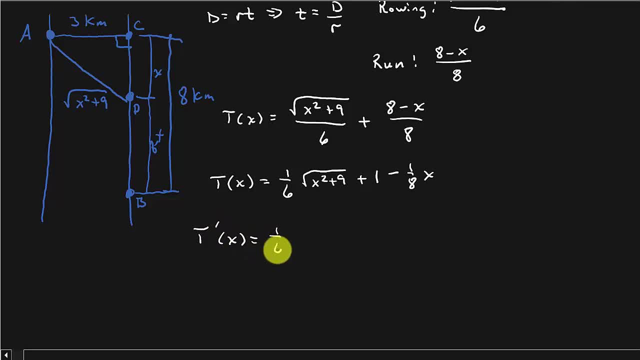 So we have t prime of x is equal to 1 sixth. All right. So remember, earlier we took the derivative of square root. Use that little shortcut. So the shortcut to take the derivative of a square root is just 2 times the square root. Okay, So remember it's 2 times whatever. 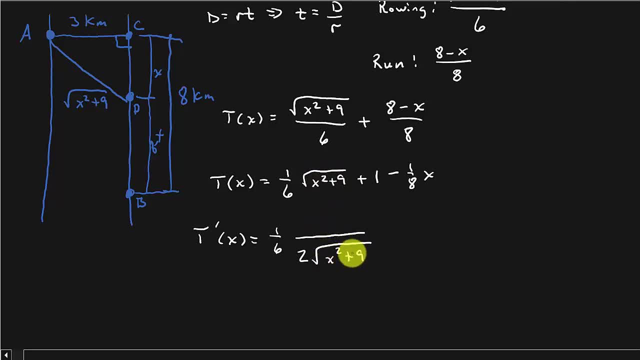 this is: And then what goes in the numerator, The derivative of what's underneath the square root, which is 2x, And then the derivative of 1 is 0.. And then the derivative of minus 1 eighth: x is minus 1 eighth. 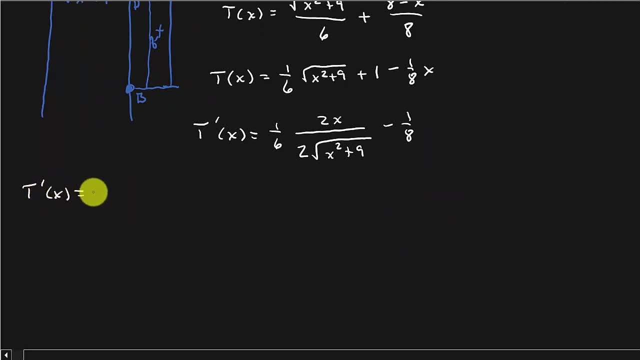 And so we get t. prime of x is equal to x over 6 square root of x squared plus 9 minus 1 eighth. So I just all I did there is I canceled the 2's. All right, Now we need. 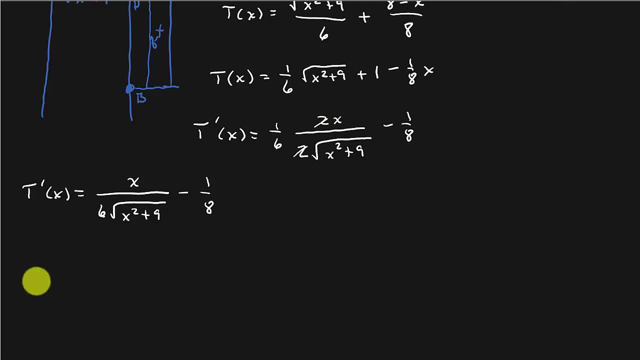 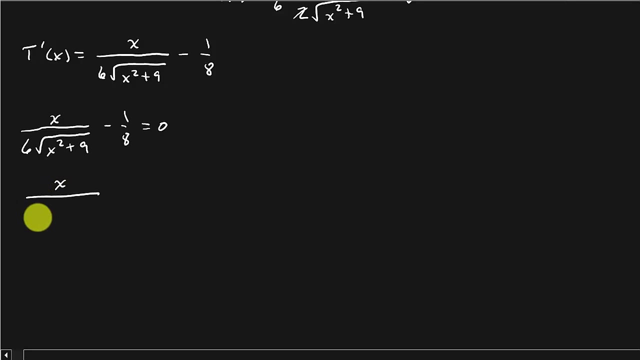 to set this equal to 0 and solve for x. So if I got x over 6 times square root, x squared plus 9 minus 1 eighth equals 0.. So I get x over 6 times the square root of x, squared plus 9 equals 1 eighth. All right, 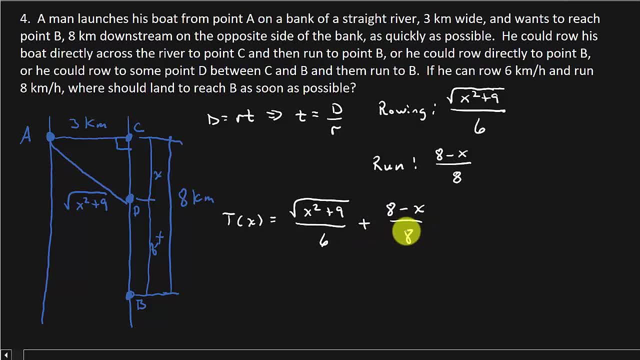 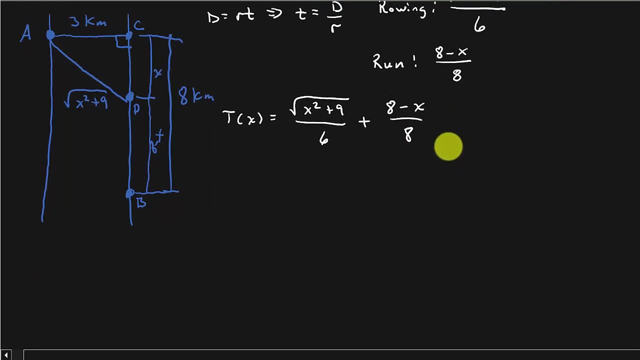 6 plus 8 minus X over 8. all right, so there's our time. so we need to take the derivative. right, you need to take the derivative. but before we take the derivative, I want to do. I want to do something real quick. it'll make it a 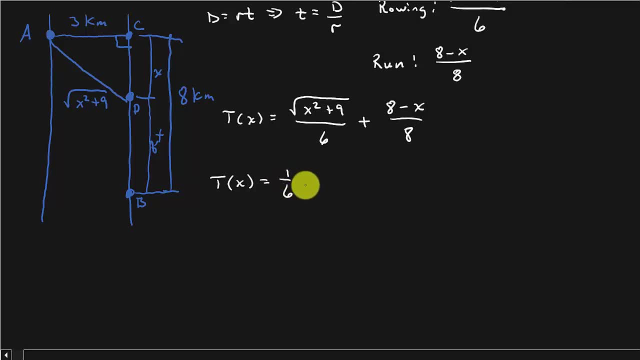 little bit easier to see how we take the derivative. so that's one-sixth square root of x squared plus 9 plus, and then this is 8 over 8, which is 1 minus one eighth X. I just split this fraction up, alright, so I think writing it like this: 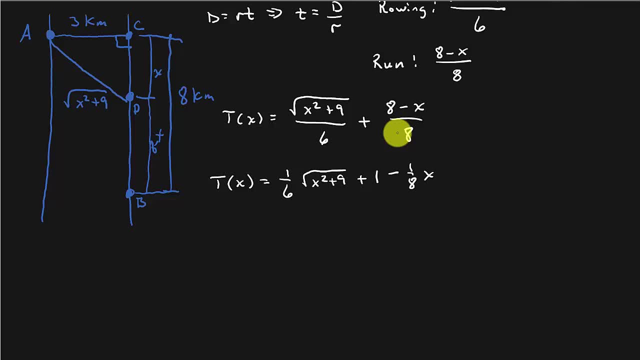 it'll make it easier to take the derivative. so we have T prime of X is equal to 1- 6, all right, so remember earlier we took the derivative of square root. use that little shortcut. so the shortcut to take the derivative of a square root is just 2 times the square root. okay, so remember it's 2 times. 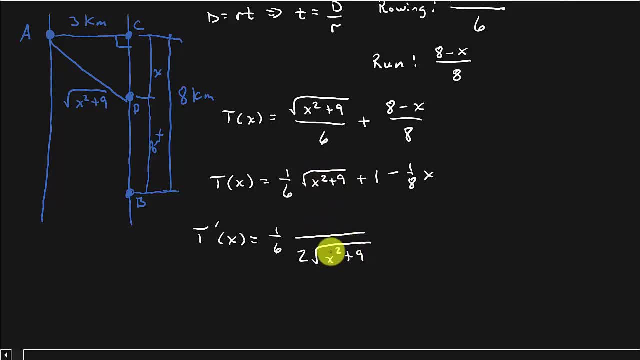 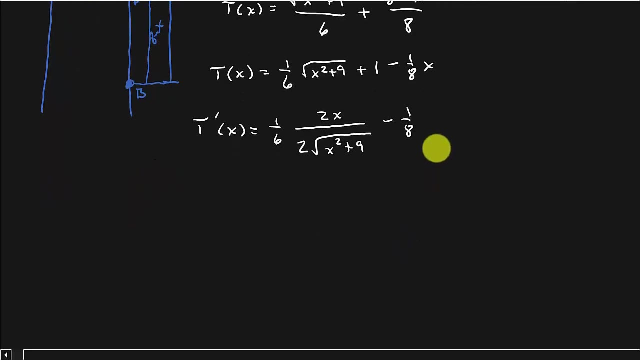 whatever this is. and then what goes in the numerator? the derivative of what's underneath the square root, which is 2x, and then the derivative of 1 is 0, and then the derivative of minus 1, 8, X is minus 1, 8, and so we get T prime of X. 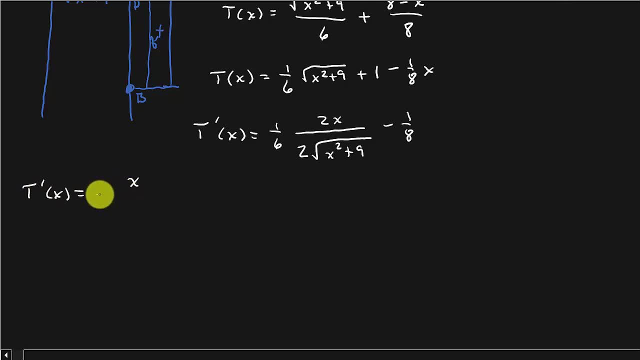 is equal to X over 6. square root of x squared plus 9 minus 1, 8. so I just all I did there is I cancelled the twos. all right, now you we need to set this equal to 0 and solve for X. so if I got X over 6 times, 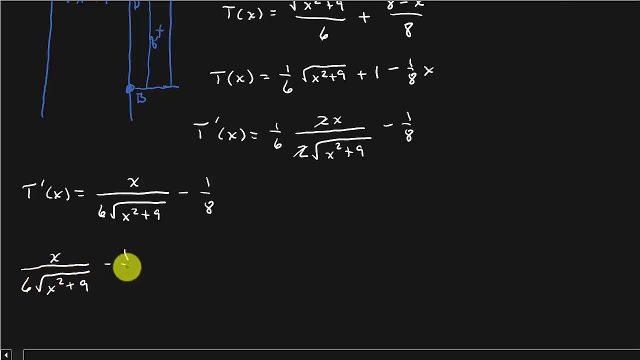 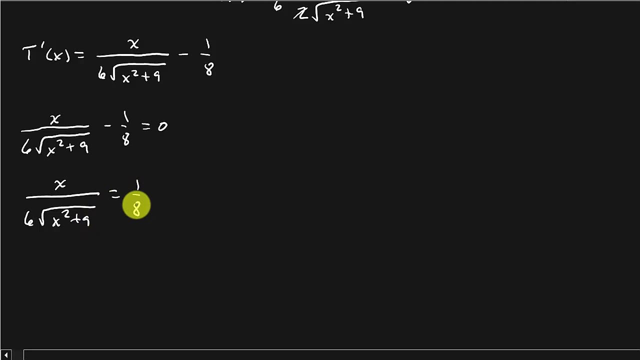 square root. x squared plus 9 minus 1, 8 equals 0. so I get X over 6 times the square root of x, squared plus 9, equals 1- 8. all right, so solving this we're going to get, let's see- what is that going to be, that's. 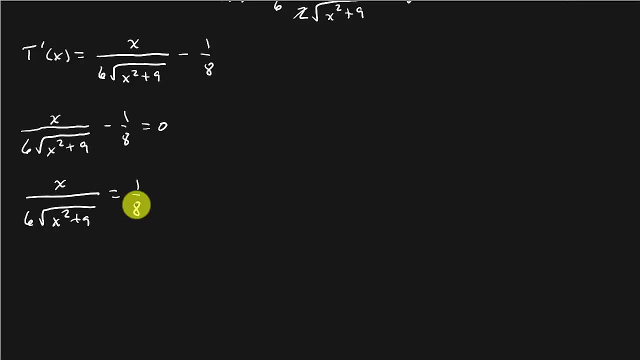 All right, So solving this, we're going to get. let's see what is that going to be. 4 over 3x equals the square root of x squared plus 9.. I just moved the 8 up. 8 over 6 is: 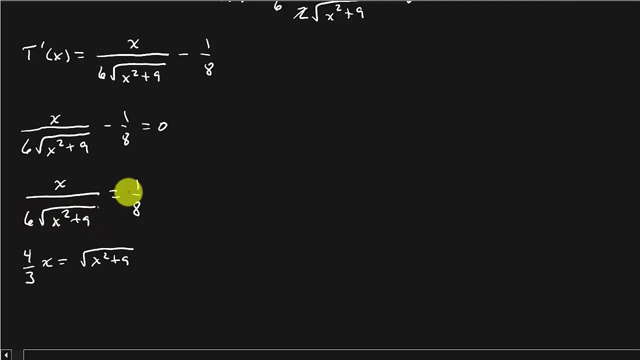 4 thirds, And then this square root of x squared plus 9, I just moved it to the other side- Then we're going to square both sides, So that's going to be 16 over 9. x squared equals and that's going to be x squared plus 9.. 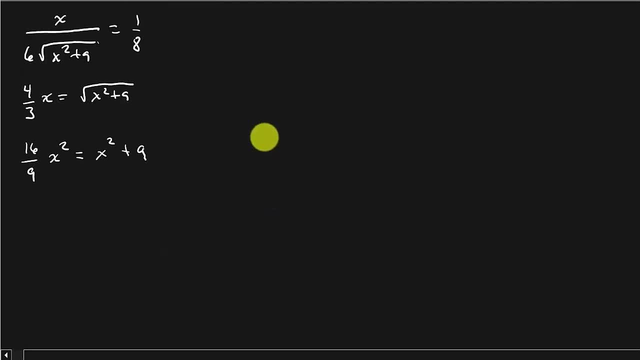 All right Now. well, let's see what happens. Maybe if I multiply everything through by 9, get rid of those fractions, that's going to be: 16 x squared equals 9 x squared plus 81. And so I get 7 x squared plus 81,- ah, I'm sorry, equals 81.. And so x squared equals. 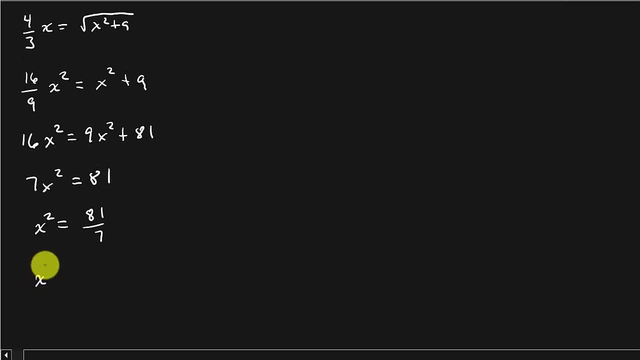 81 over 7, and so x squared equals 9 over square root, not x squared. x equals 9 over square root of 7. all right, that's our only critical number. all right, it now keep in mind when I, when I go from this step to this step. it is plus or minus, but we know it's not minus. okay, because that. 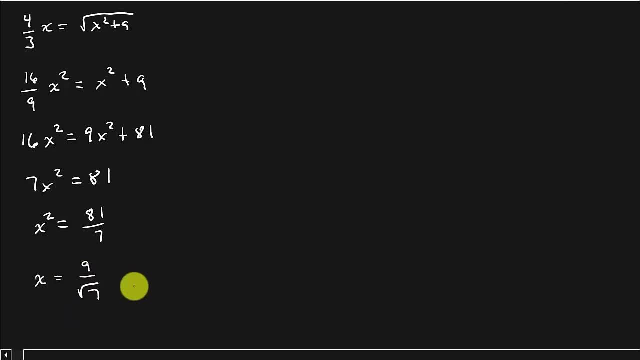 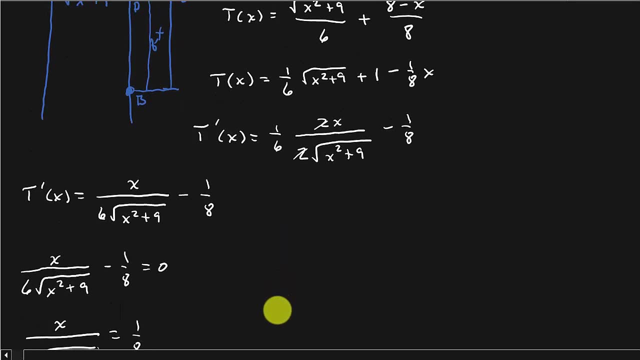 distance can't be negative, so we only use the positive. all right, so we've got 9 over square root of 7. now let's come back up here real quick. so let me just write that 9- I mean x- equals 9 over square root of 7. now the one thing that we've got to look at here is that we're on the interval 0. 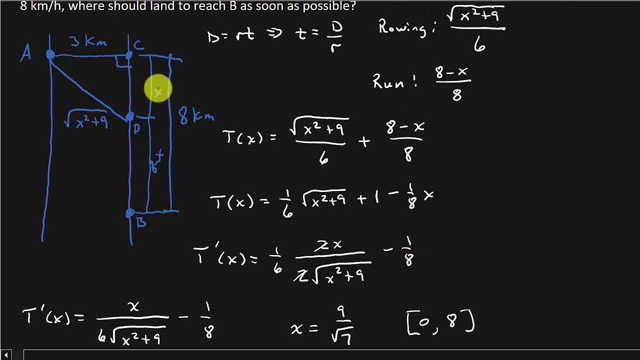 to 8. see, that's that's. that's the interval 0 to 8. so that's the interval 0 to 8. so that's the interval 0 to 8. so that's the all that X can be. X can be 0, so that means we would just go straight across. 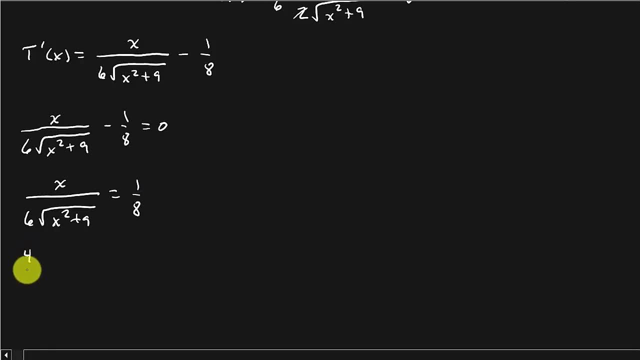 going to be 4 over 3. X equals the square root of x squared plus 9. I just moved the 8 up: 8 over 6 is 4 thirds, and then this square root of x squared plus 9, and just moved it to the other side. then we're going to square both sides. so 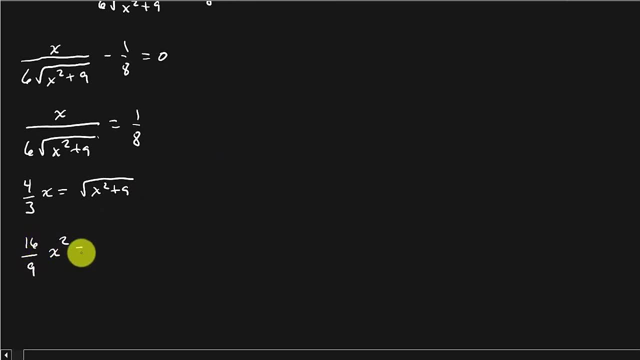 that's going to be 16 over 9 x squared equals, and that's going to be x squared plus 9. all right now. well, let's see what happens. maybe, if I multiply everything through by 9, get rid of those fractions. that's going to be 16 x squared equals. 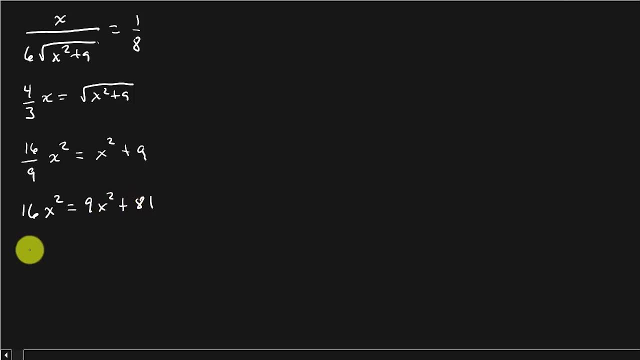 9 x squared plus 81, and so I get 7 x squared plus 81- now, I'm sorry, equals 81, and so x squared equals 81 over 7, and so x squared equals 9 over square root, not x squared x equals 9 over square root of 7. all right, that's our only. 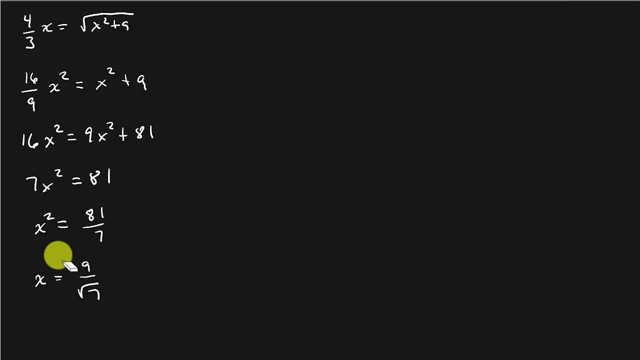 critical number. all right, it now keep in mind when I, when I go from this step to this step. it is plus or minus, but we know it's not minus. okay, because that distance can't be negative, so we only use the positive. all right, so we've got. 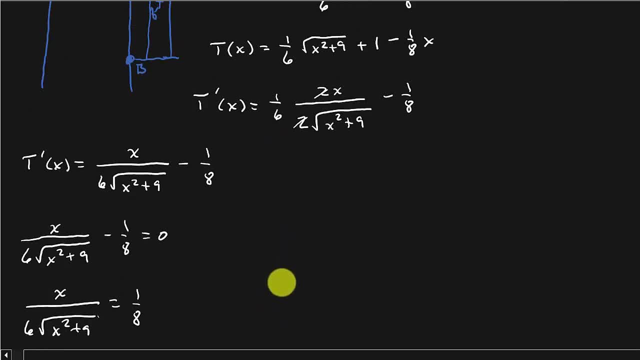 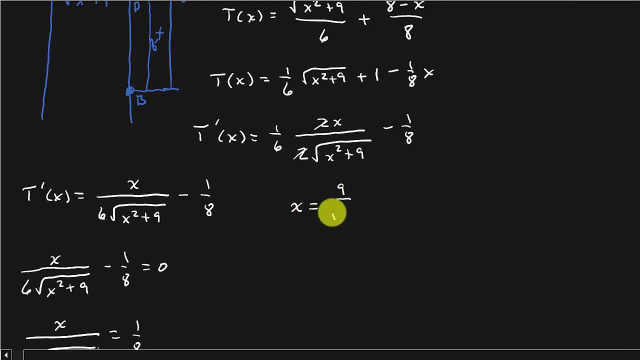 9 over square root of 7. now let's come back up here real quick. so let me just write that 9- I mean X- equals 9 over square root of 7. Now the one thing that we've got to look at here is that we're on the interval 0 to 8.. 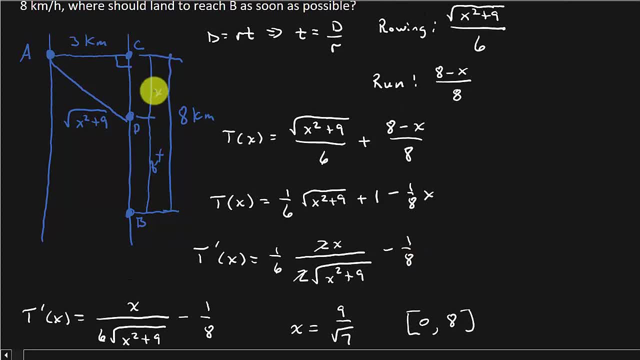 See, that's all that x can be. x can be 0, so that means we would just go straight across. Or x can be 8. And if it's 8, that means we go directly to b, But it can't be anything less than 0, and it can't be anything more than 8.. 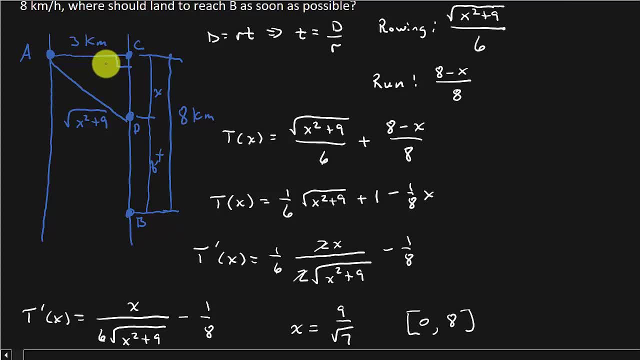 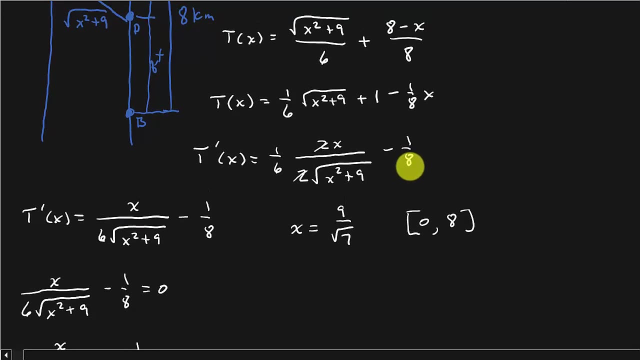 or X can be 8, and if it's 8 that means we go directly to B. but it can't be anything less than 0 and it can't be anything more than 8. so we have- we have a closed interval here. so we've got to take all three values, the 9 over square. 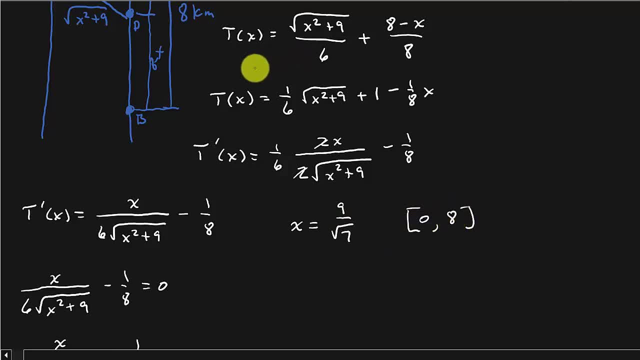 root of 7, the 0 and the 8 and we have to plug it back into the original equation to see which one gives us what the smallest value. okay, so if I do T of 0- and I'm not going to show me plugging the numbers in, but T of 0 is 1.5, T of 9. 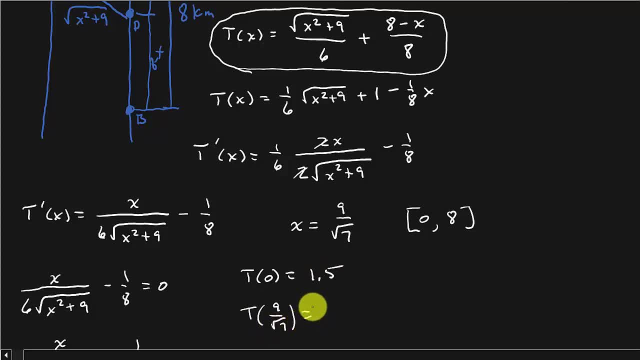 over square root of 5, 7, that is 1.33, and T of 8 is equal to 1.42 and you can see, of the 3 that we evaluated, that's our smallest. so that means X is equal to 9 over square root. 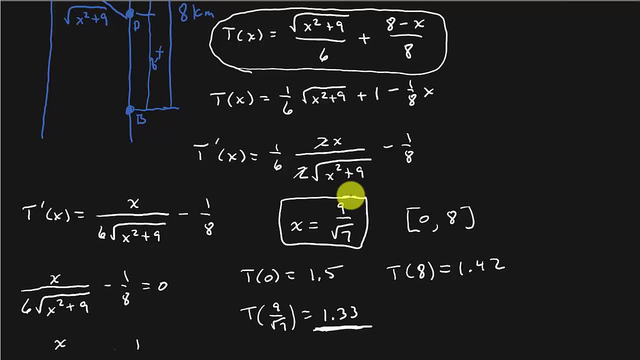 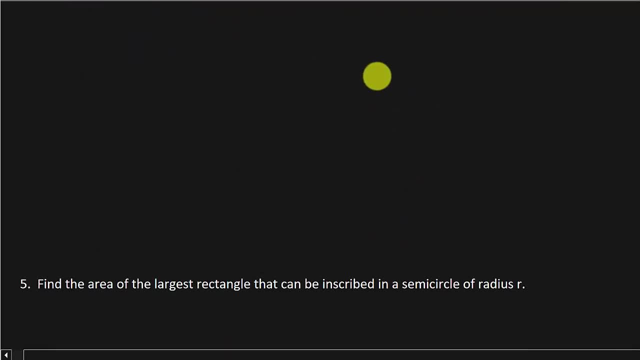 of 7, and that's your answer. all right, all right, so let's take a look at the next problem. all right, so find the area of the largest rectangle that can be inscribed in a semicircle of radius R. all right, so let's, let's draw a picture, okay? so we 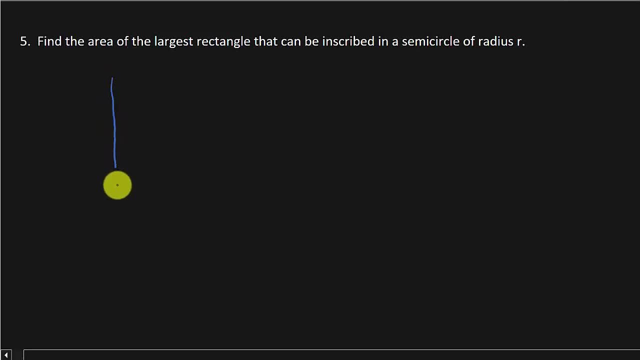 draw a picture. so if I draw a picture, the semicircle is gonna be right there and this right here is the. this is: I'm drawing it in the middle, okay, and so we know that this is our. this is negative R. okay, that's the radius of the circle. and so now, if I draw me a rectangle in here, I 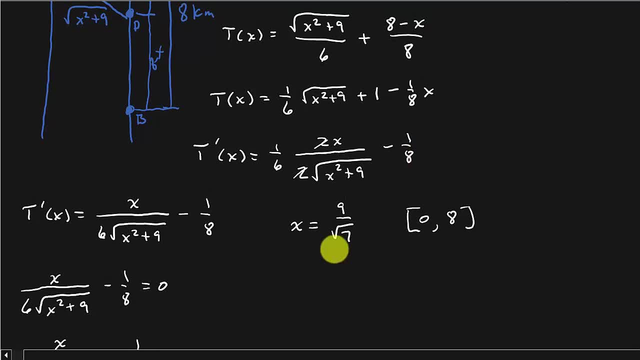 So we have a closed interval here. So we've got to take all three values- the 9 over square root of 7, the 0, and the 8, and we have to plug it back into the original equation to see which one gives us what. 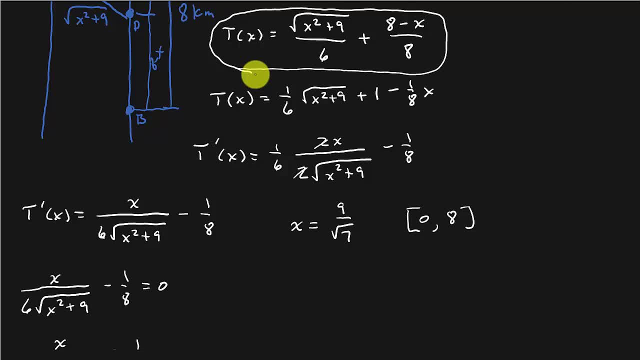 The smallest value. Okay, So we're going to take the smallest value and we're going to plug it back into the original equation. So if I do t of 0, and I'm not going to show me plugging the numbers in- 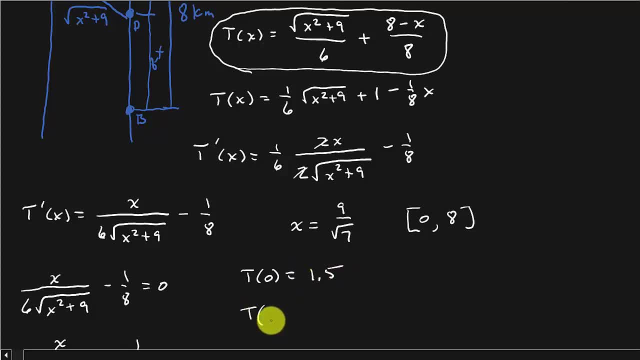 but t of 0 is 1.5, t of 9 over square root of 7, that is 1.33, and t of 8 is equal to 1.42.. And you can see, of the three that we evaluated, 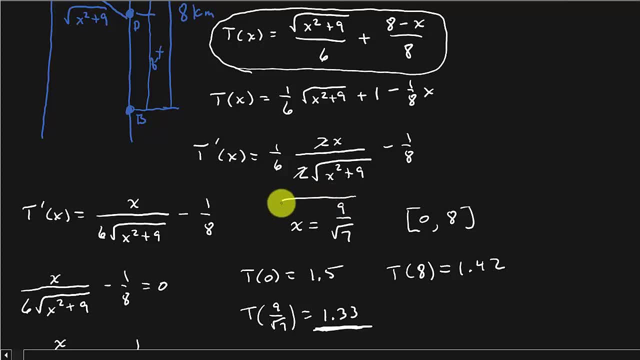 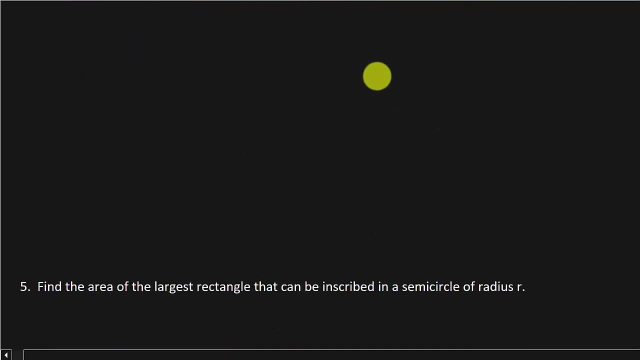 that's our smallest. So that means x is equal to 9 over square root of 7.. And that's your answer. Alright, Alright. So let's take a look at the next problem. Alright, Alright. So find the area of the largest rectangle that can be inscribed in a semicircle of radius. 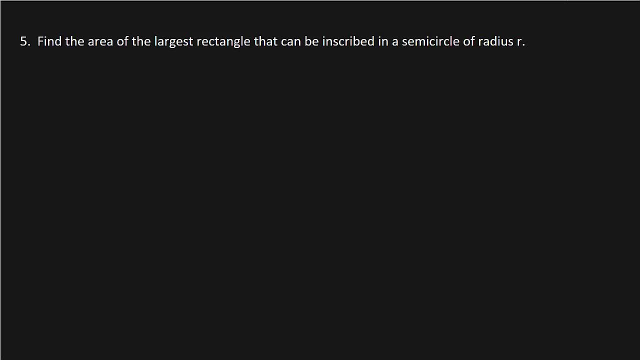 Alright, So let's draw a picture. Okay, So we draw a picture. So if I draw the semicircle, it's going to be right there And this right here is the. this is I'm drawing it in the middle. 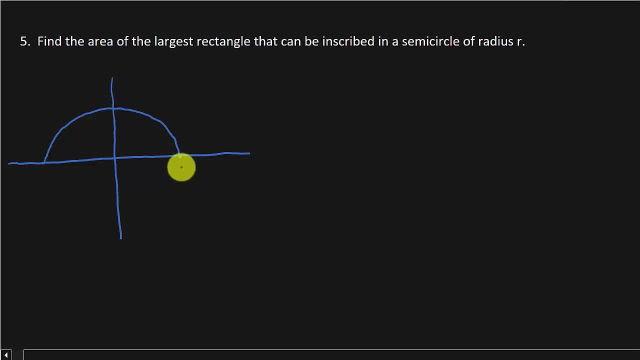 Okay, Okay, And so we know that This is r, This is negative r. Okay, That's the radius of the circle, And so now, if I draw me a rectangle in here, I want the largest area for the rectangle. 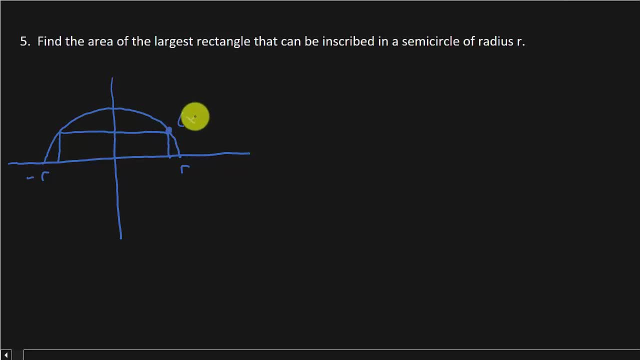 Alright, So we can, we can have a point here: x, y. So I know this distance here is y, This distance, here it goes out x, x units And from here it goes out x units, right, 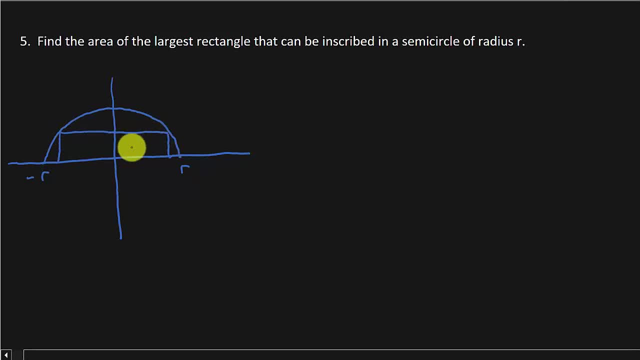 I want the largest area for the rectangle. alright, so we can, we can have a point here: XY. so I know this distance here is Y, this distance, here it goes out X, X units and from here it goes out X units. right, it goes X units this way, X. 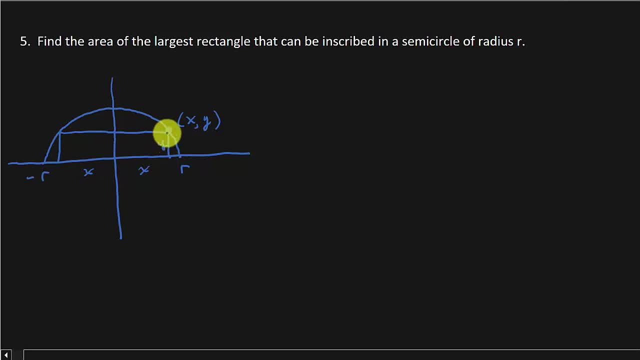 units this way, alright, because if I plot the point X, Y, X, Y. and so what do we want? to maximize the area? well, what's the area of this rectangle? well, the area is length times width. so see, that's 2x times Y. well, now we have to do what we. 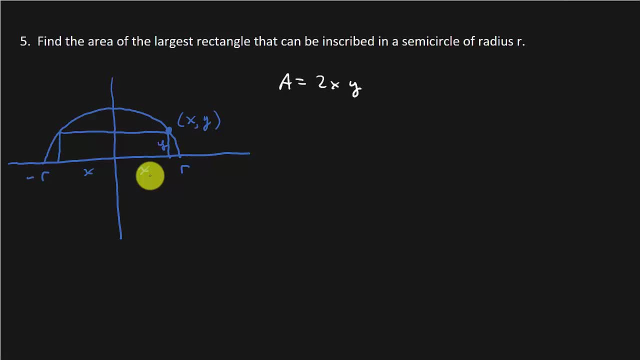 have to take the derivative of this thing, don't we see that we've got to take the derivative. so I need to somehow get this area here, all in terms of X or all in terms of Y? well, well, to get rid of the Y, we can use the fact that we know this point here. this: 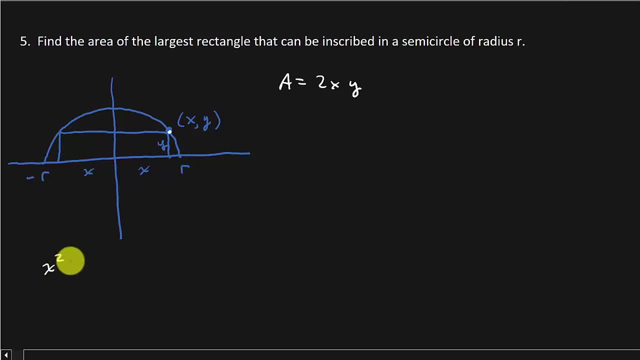 point XY lies on the circle. X squared plus Y squared equals R squared. remember that from algebra. when you find in the equation of a circle, say we place the center of the circle here at 0, 0, all right, and so if we solve this, we get Y. 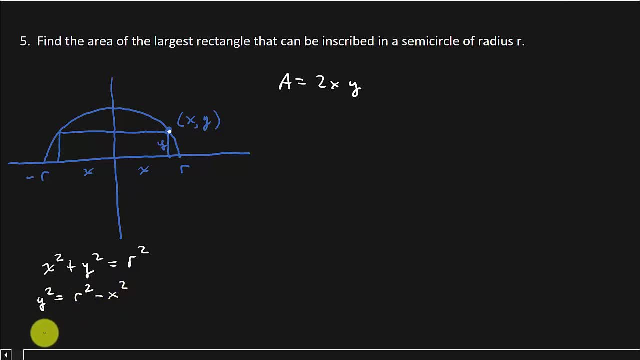 squared is equal to R squared minus X squared. so Y is equal to the square root of R squared minus X squared. now, that's plus or minus. okay, that's plus or minus here, but we use the positive because we're using the part that's above the x-axis. if we were drawing it down here, we would 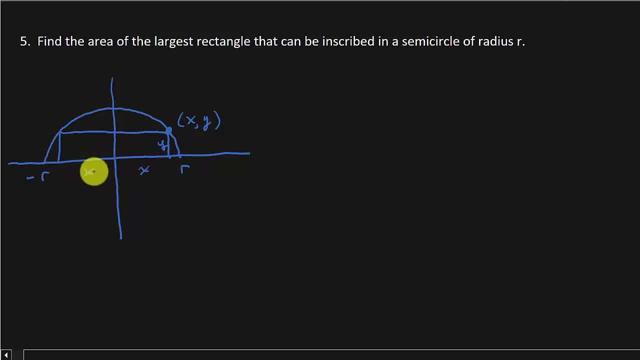 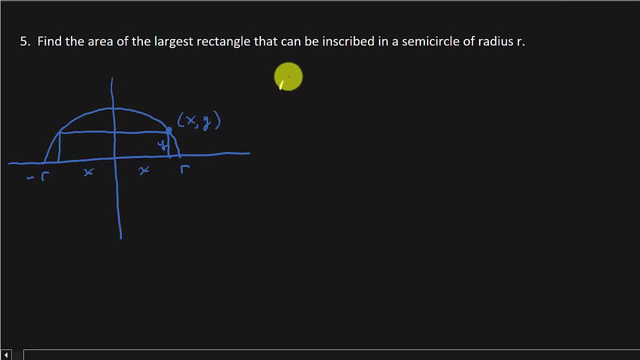 Well, what's the area of this rectangle? Well, the area is length times width. So see, that's 2x times y. Well, now we have to do what We have to take the derivative of this thing, don't we? 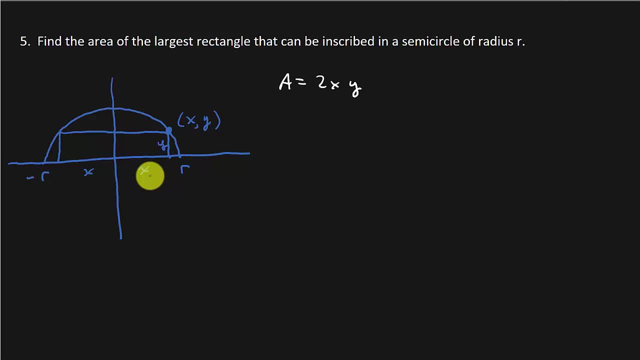 See that We've got to take the derivative. So I need to somehow get this area Okay, area here all in terms of x or all in terms of y. Well, to get rid of the y, we can use the fact that we know this point here. this point x, y lies on the circle x squared plus. 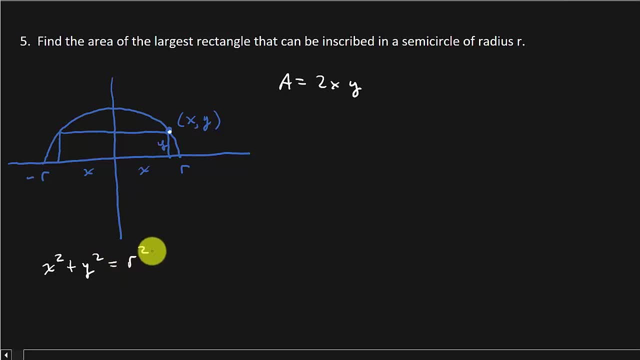 y squared equals r squared. Remember that from algebra. when you find an equation of a circle, say we place the center of the circle here at 0,, 0,, all right. And so if we solve this we get: y squared is equal to r squared, minus x squared, So y is equal to the square. 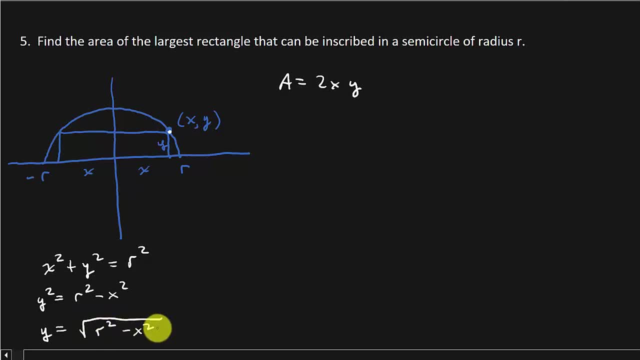 root of r squared minus x squared. Now, that's plus or minus. okay, That's plus or minus here, but we use the positive because we're using the part that's above the x-axis. If we were drawing it like this, we'd be drawing it like this. We'd be drawing it like this: 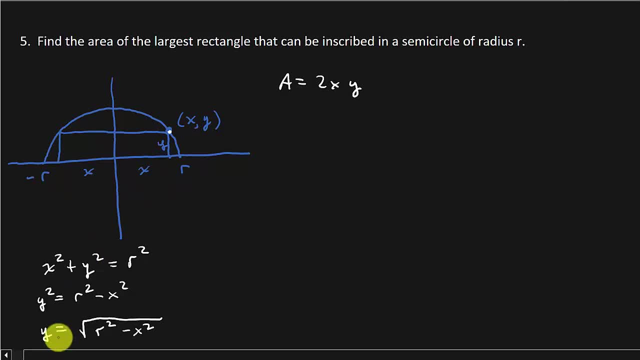 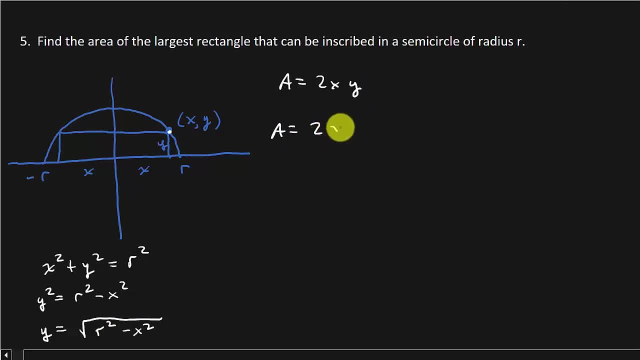 this y with this. So we've got: area is 2x times the square root of r squared, minus x squared. Now, what's the domain of our function? Well, that's going to be what? 0 less than or equal to x, less than or equal to r. okay, Because you know, for one thing we've got. 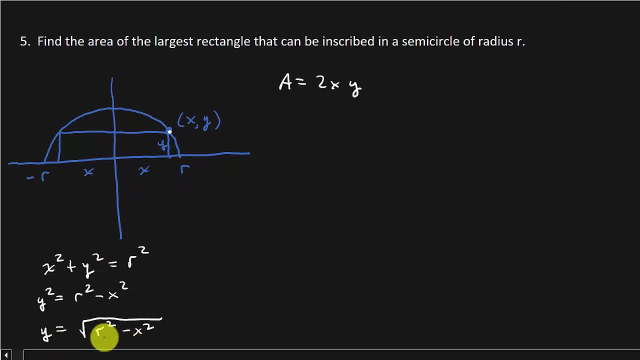 use the negative. so so we have: Y is equal to this, so we can replace this Y with this. so we got: area is 2x times the square root of R squared minus X squared. now what's the? what's the domain of our function? well, that's going to be what? zero less than or equal to X. 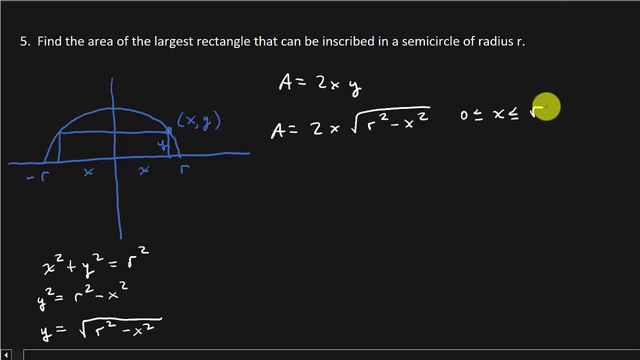 less than or equal to R. okay, because you know, for one thing, we've got a, we can't have a negative underneath that. so we can't have a negative underneath that. so let's point out the first function here: for the negative, that is equal to zero. 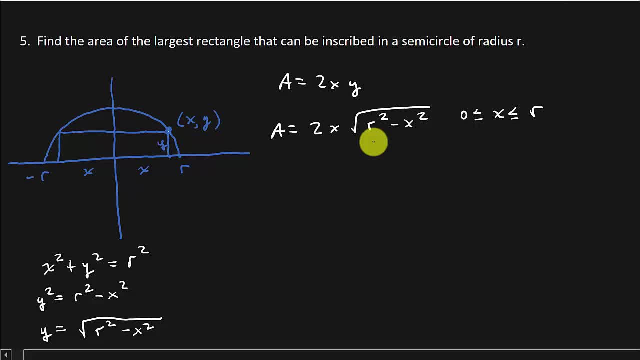 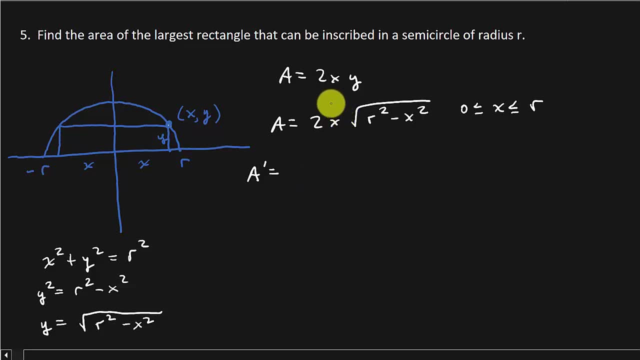 plus zero again. so that's peach cheese 4 times four. so that's what? absolutely whatever that is squared of the surface support, that'saboide all right, but then what's the derivative? the derivative is equal to 0. sum of total Teacher level of instant based is equal to 2 times 0. so times the freedom of induction, or: 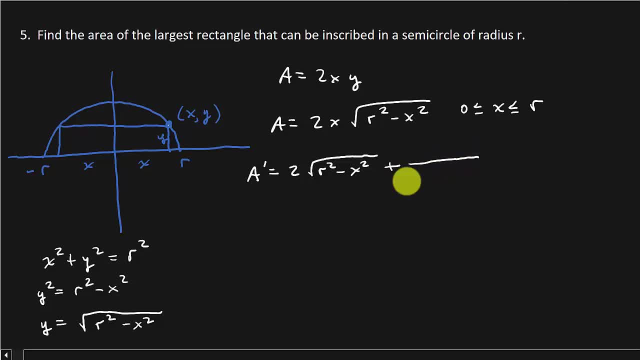 iek. what's the derivative of which is zero plus 1? is square root of R squared minus X squared. shortcut for finding the derivative of a square root. and then what goes up here? negative 2x. okay, see the derivative of what's underneath the radical is negative 2x, and then times. 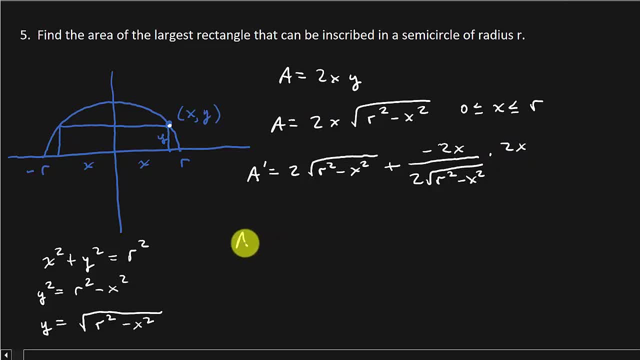 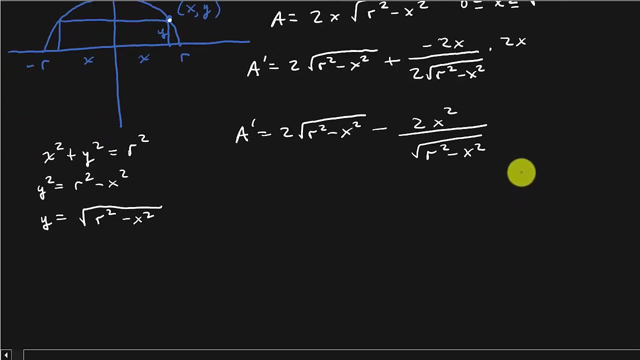 the first function, so times 2x. so I get a: prime is equal to 2 square root r squared minus x squared minus. what is that? 2x squared over the square root of r squared minus x squared. Alright. so now let's set this thing equal to zero, so I'm going to get 2 square root. 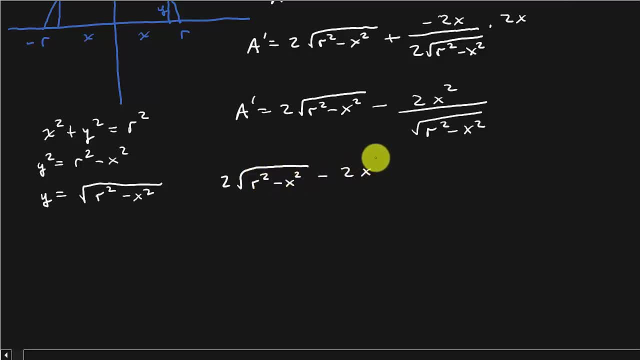 r squared minus x squared minus 2x squared over the square root of r squared minus x squared equals zero, So I'll just move this over. so that's going to be 2. square root of r squared minus x squared equals 2x squared over r squared minus x squared square root of that. 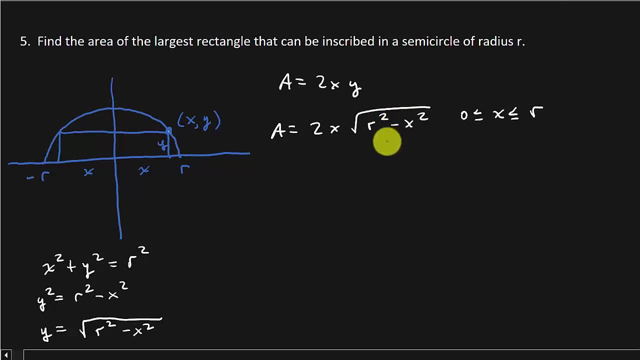 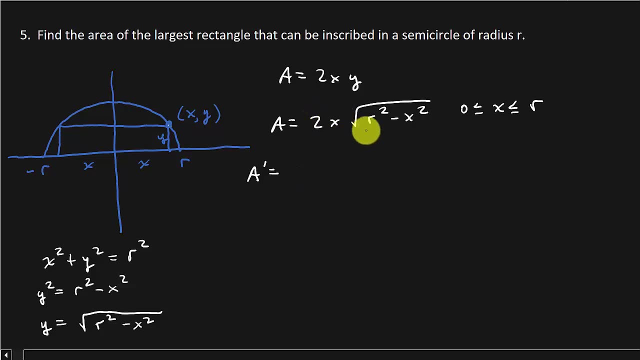 a. we can't have a negative underneath the radical, All right. So now we have to take the derivative. So the derivative: well, this is product rule. I've got 2x times the square root of r squared minus x squared. So the derivative of the first function is 2 times the second function. 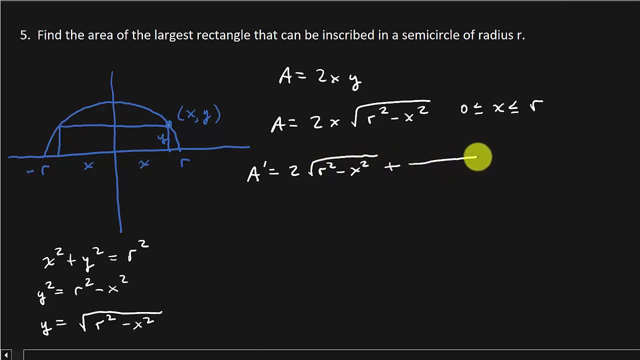 plus the derivative of the second function, And once again, here's a shortcut for finding the derivative of a square root. And then what goes up here? Negative 2x. Okay, See, the derivative of what's underneath the radical is negative 2x. And then 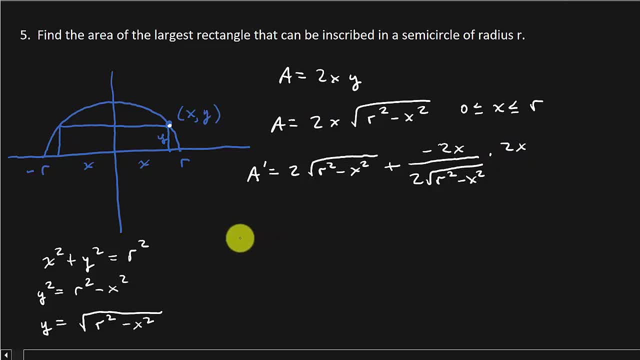 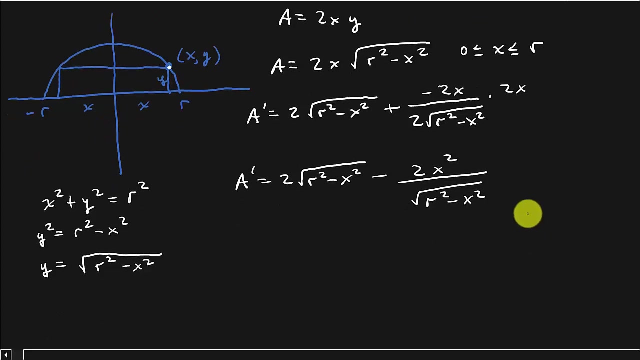 times the first function, So times 2x. So I get a: prime is equal to 2 square root r squared minus x squared minus. what is that? 2x squared over the square root of r squared minus x squared. All right, So now let's set this thing equal to 0.. So I'm going to get 2 square. 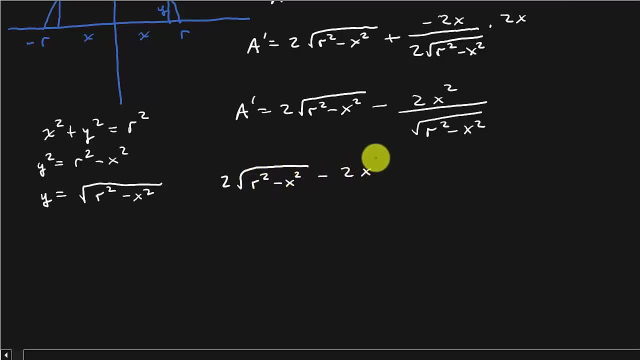 root of r squared minus x squared minus 2x squared over the square root of r squared minus x squared equals 0.. So I'll just move this over. So that's going to be 2. square root of r squared minus x squared equals 2x squared over r squared minus x squared square root of that, And so. 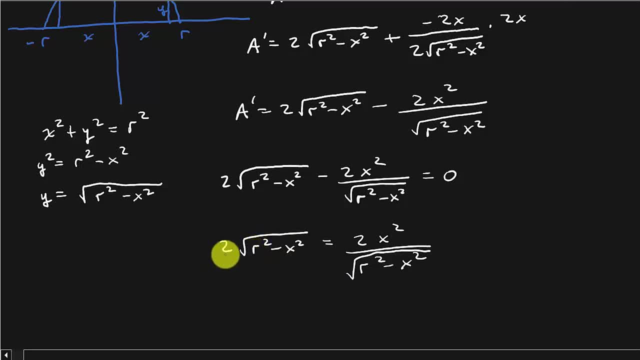 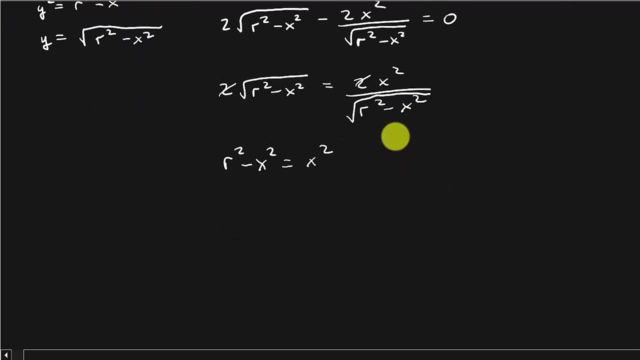 then I can multiply. But look at this, I can cancel those 2s out. You see that? And then if I multiply this times this, that's going to give me r squared minus x squared equals x squared, And so I get. 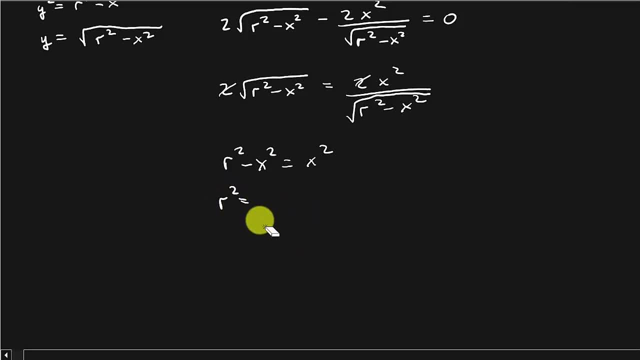 r squared is equal to 2x squared, And so that's going to give me x squared is equal to 2x squared, And so that's going to give me: x squared is equal to r squared over 2.. And so x is equal to what? 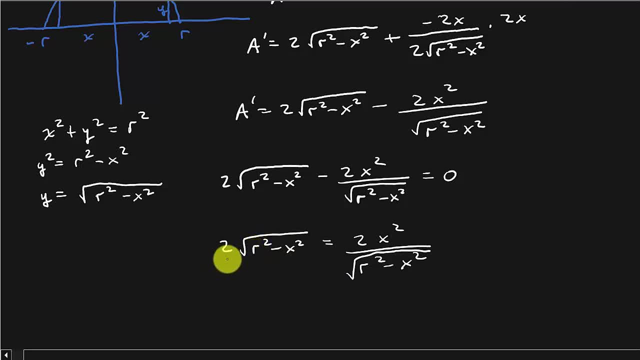 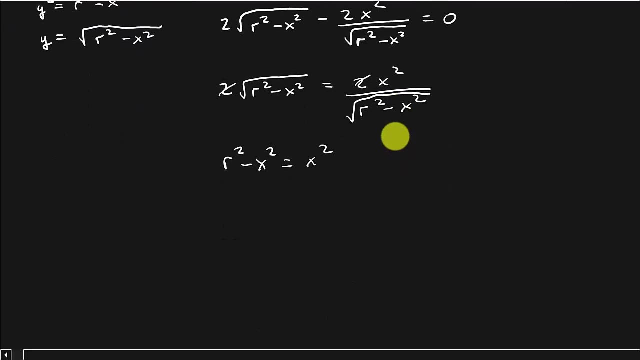 And so then I can multiply. but look at this, I can cancel those 2's out. you see that? and then if I multiply this times this, Okay, That's going to give me r squared minus x squared equals x squared. 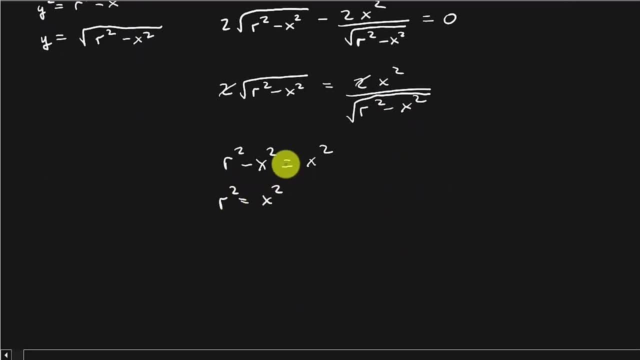 And so I get: r squared is equal to 2x 2x squared. and so that's going to give me: x squared is equal to r squared over 2, and so x is equal to what r over square root of 2.. 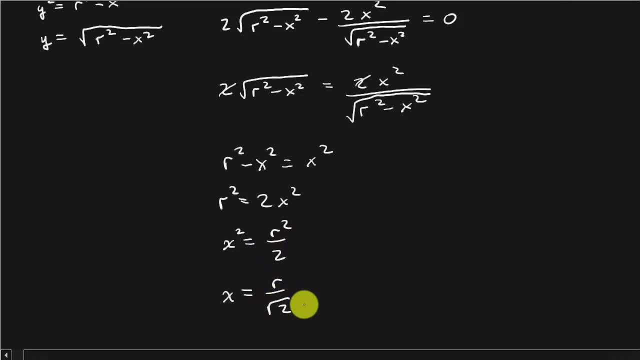 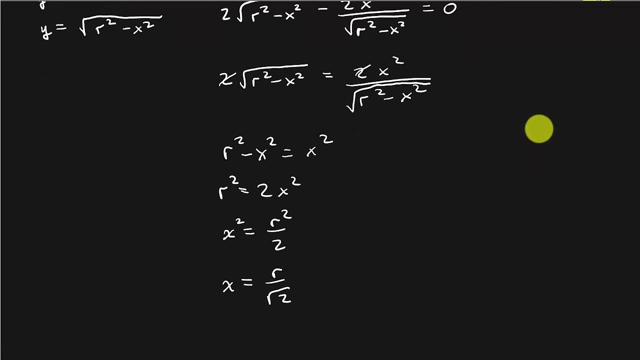 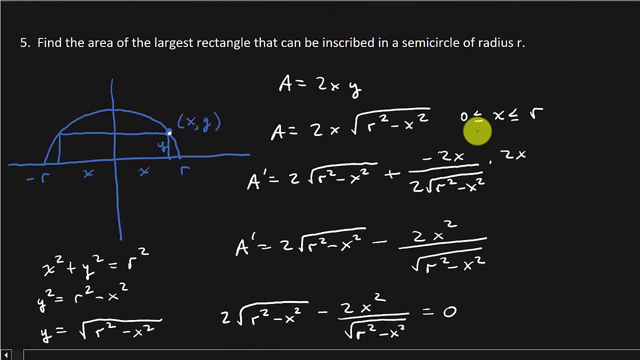 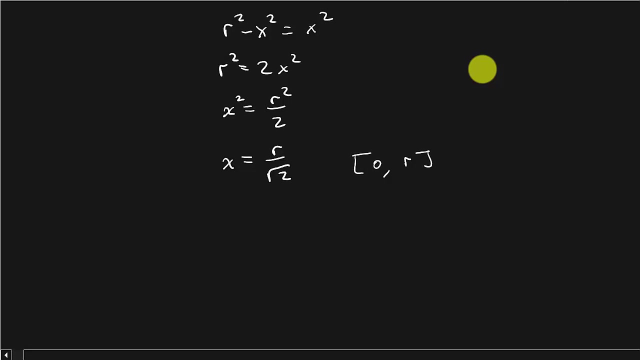 Alright, and this is going to be a maximum. okay, this is going to be my maximum. and also, remember we're between zero and r, remember this up here: we're between zero and r. I mean, you know, you know it's a maximum. this is, this is positive, right, we know. 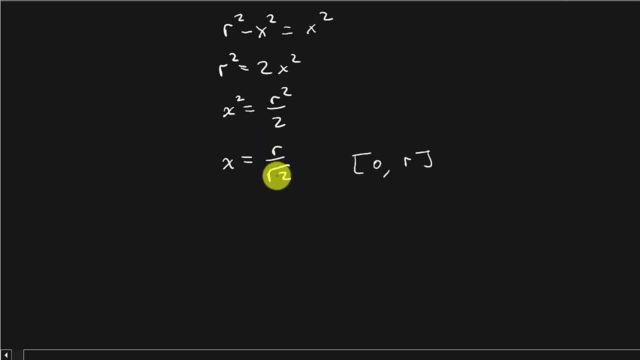 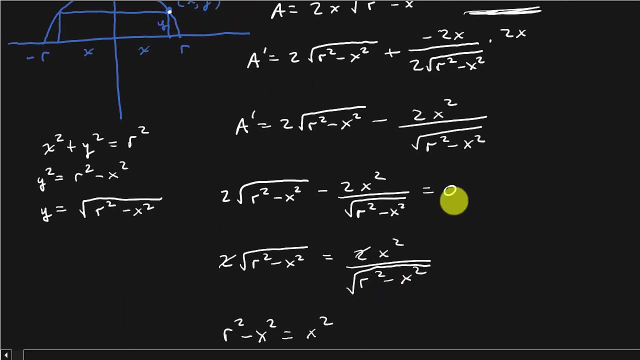 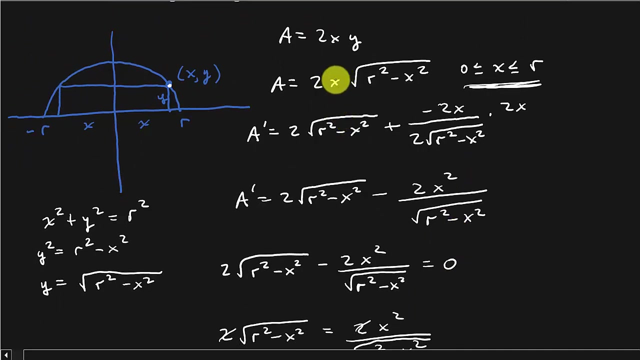 this is positive because r is positive, square root of 2 is positive. So if we do, if we do a of a of zero and a of r, I mean- just look at this up here- a of zero. So if I plug zero in here, see that's zero times. whatever that is is zero. 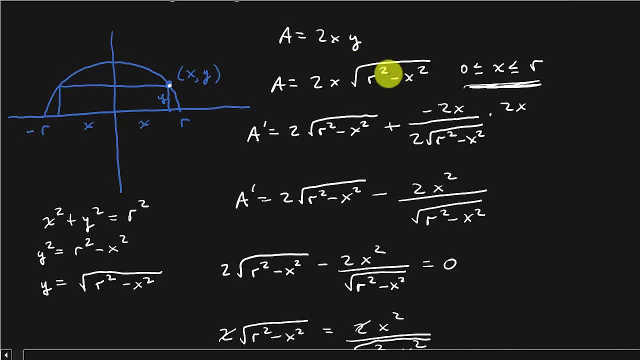 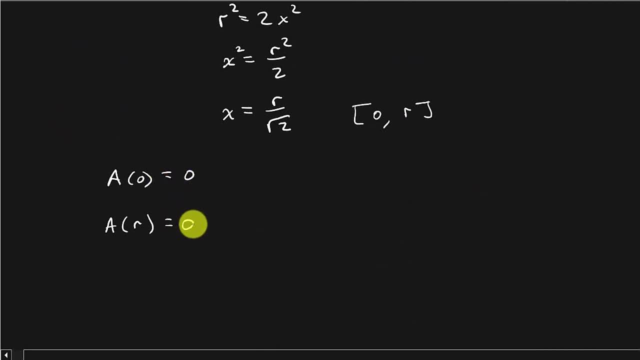 And then if I plug r in, that's r squared minus r squared, that's zero, and so that makes the whole thing zero. So both of these are equal to zero, and so we know this gives us our maximum area. Now remember, let me erase this. 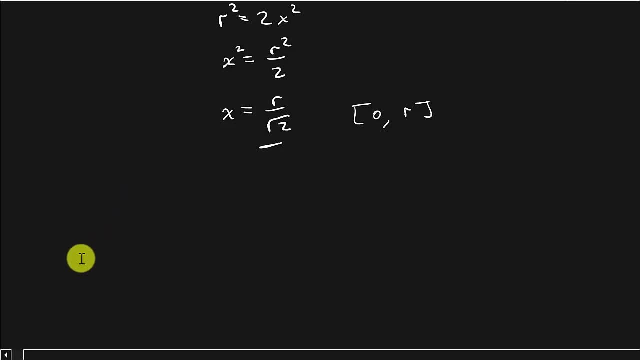 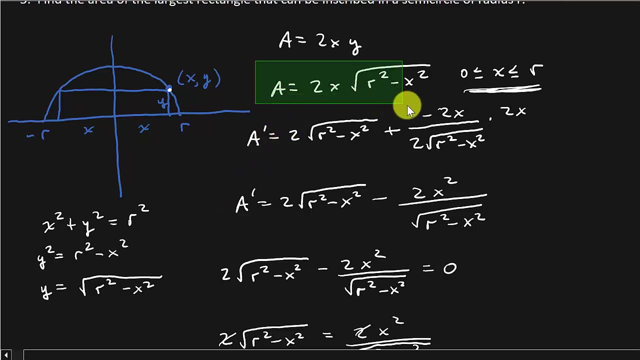 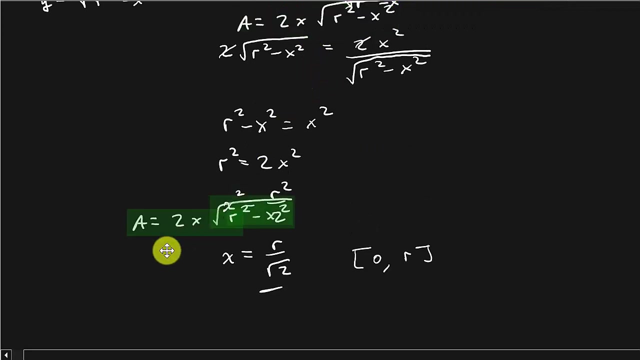 They want to know what is the maximum maximum area. That's what they're asking for. So what I'm going to do is I'm going to grab this and I'm going to pull it down here so we can, so we can see the function. alright. 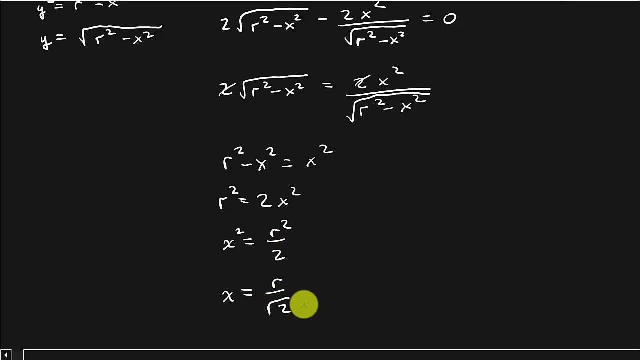 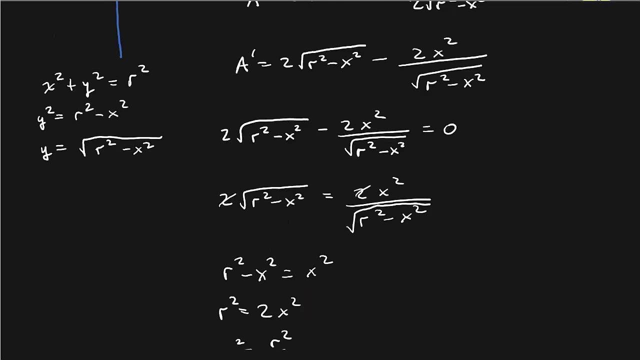 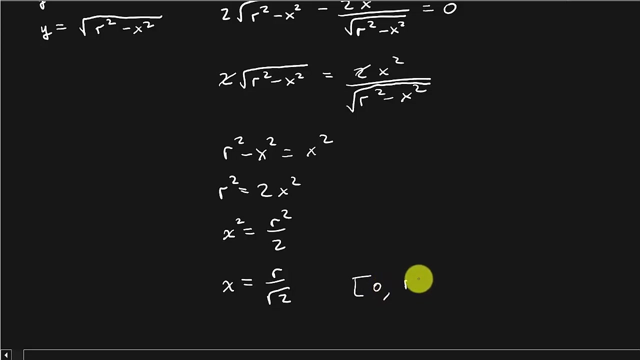 r over square root of 2.. All right, And this is going to be a maximum. OK, This is going to be my maximum. And also, remember we're between 0 and r, Remember this up here: We're between 0 and r, So I mean, you know it's a maximum. 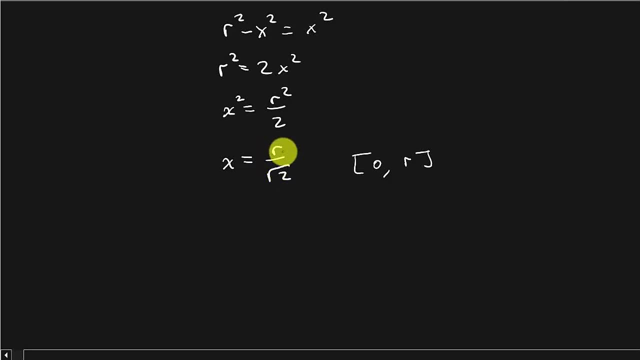 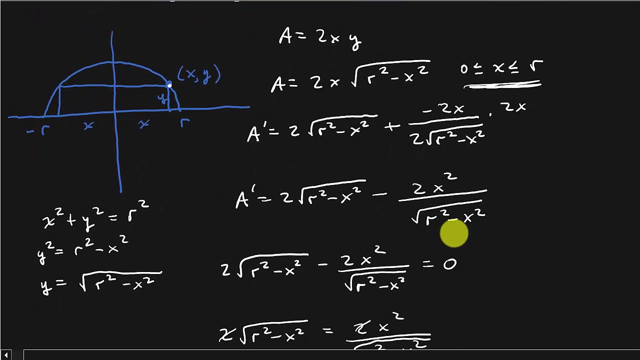 This is positive. right, We know this is positive because r is positive, Square root of 2 is positive. So if we do a of 0 and a of r, I mean- just look at this up here- a of 0.. So if I plug 0 in here, See: 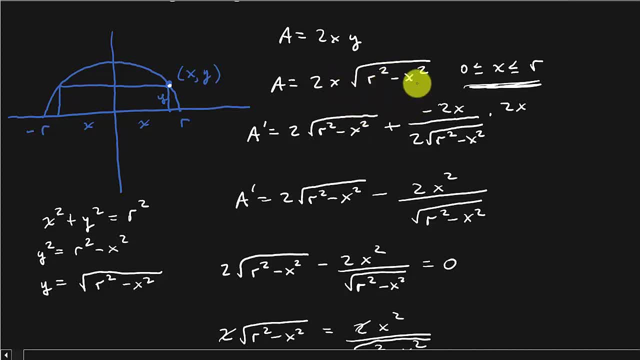 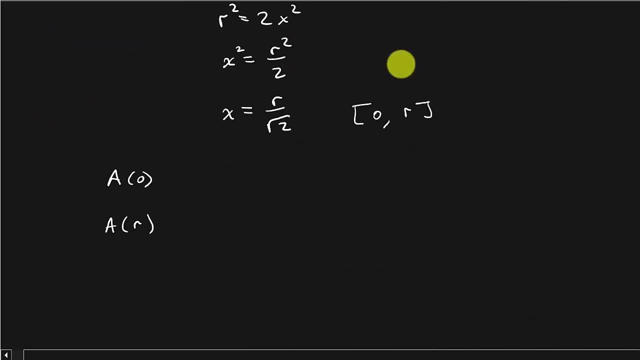 that's 0 times whatever that is, It's 0.. And then if I plug r in, That's r squared minus r squared, That's 0. And so that makes the whole thing 0. So both of these are equal to 0. And so we know. 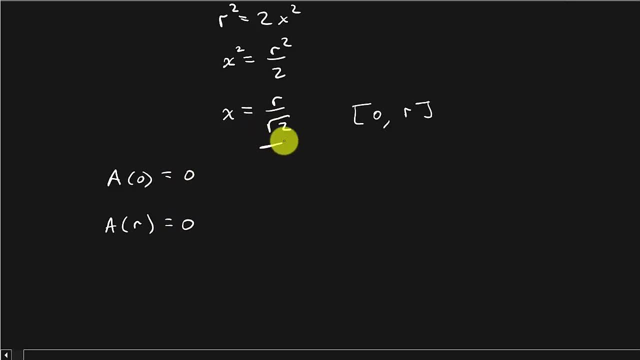 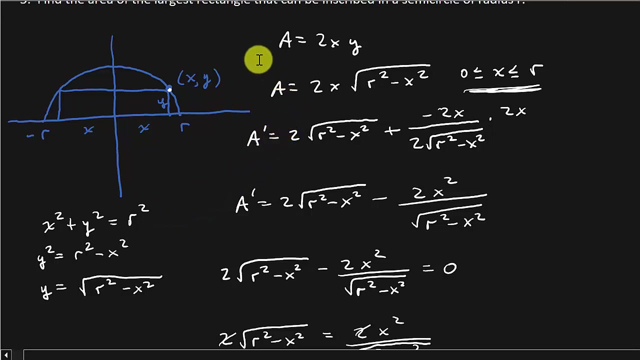 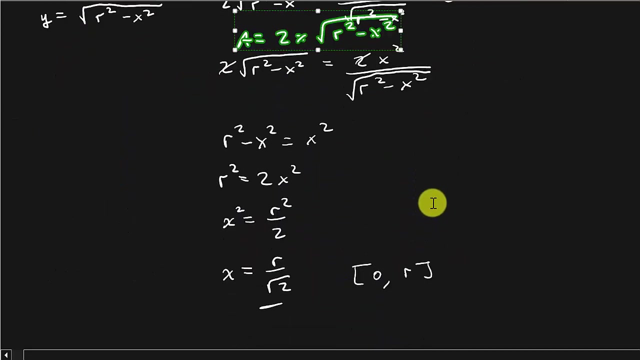 this gives us our maximum area. now remember, let me erase this. they want to know what is the maximum maximum area. that's what they're asking for. so what I'm going to do is I'm going to grab this and I'm gonna pull it down here. so 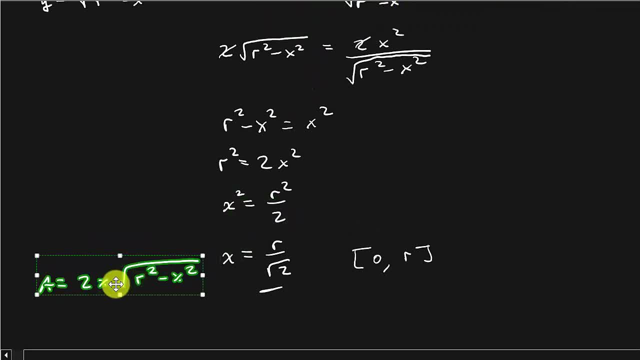 we can. so we can see the function. all right, so the maximum area is equal to well, I'm gonna take this and plug it in for X. so that's 2 times R over the square root of 2 times the square root of R squared minus R over the square. 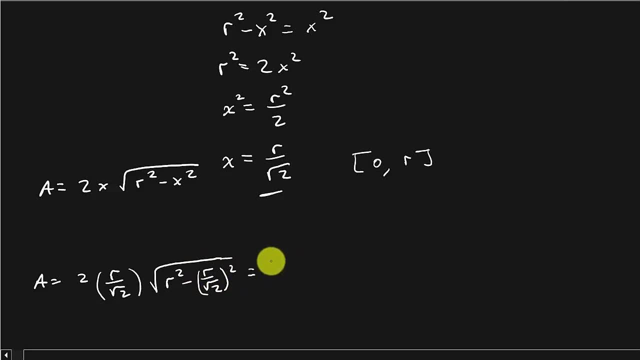 root of 2, and so that's going to be 2 times R over square root of 2, times the square root of R squared minus R squared over 2, which this is going to be 2 times R over the square root of 2. 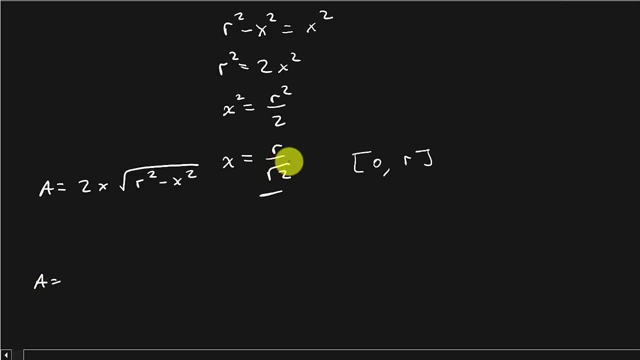 So the maximum area is equal to well, I'm going to take this, I'm going to take this and plug it in for x. So that's 2 times r over the square root of 2 times the square root of r squared minus. 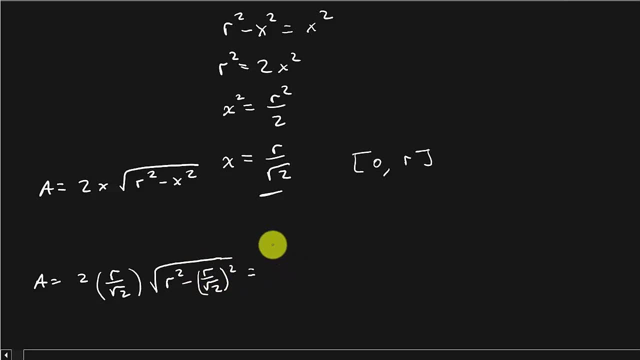 r over the square root of 2.. And so that's going to be 2 times r over square root of 2 times the square root of r squared minus r squared over 2.. Which this is going to be 2 times r over the square root of 2 times the square root. now, 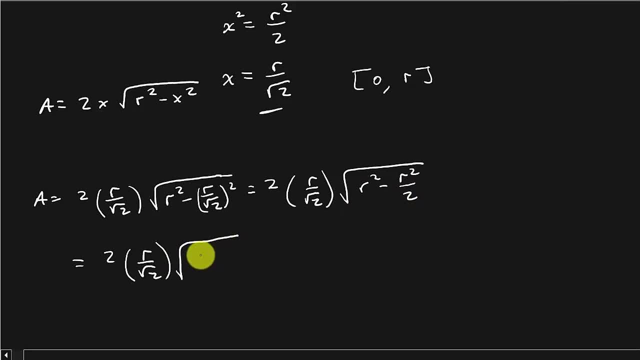 r squared minus r squared over 2, well, that's just r squared over 2.. So this is going to be 2 times r over square root of 2, times r over square root of 2, which is 2r squared over 2, which is r squared. 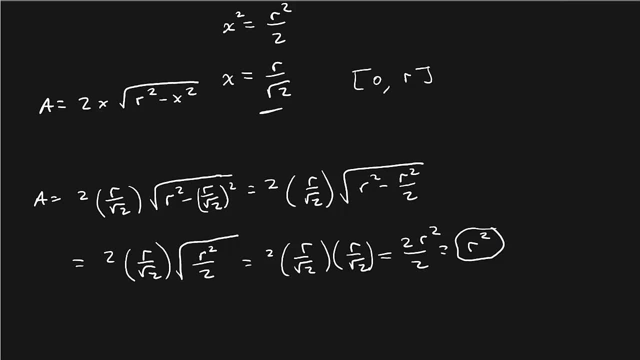 And that is your maximum area. Alright, so you know, doing these optimization problems, it's not. it's not that bad. You just got you got to. the main thing is getting that function that you're trying to maximize or minimize. 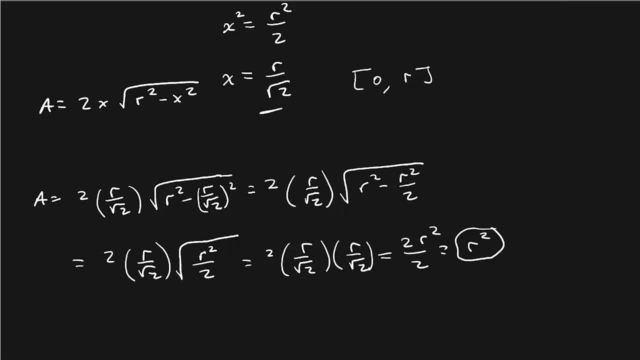 And getting it all into one In terms of one variable And then taking the derivative. That's all you're doing, Alright, So I hope this helped. I've got a. I've got more videos on optimization problems. There's a bunch of videos I have. it's just one problem per video. 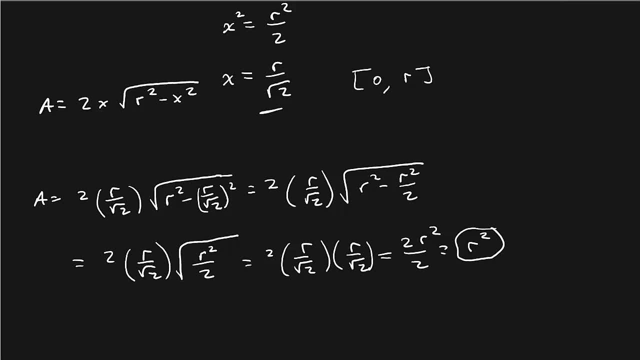 This right here is just a bunch of problems in one video, Alright, But if but if you want to look at some different kinds of problems, just search my channel for optimization And a bunch of them will come up. So I hope the video helped. 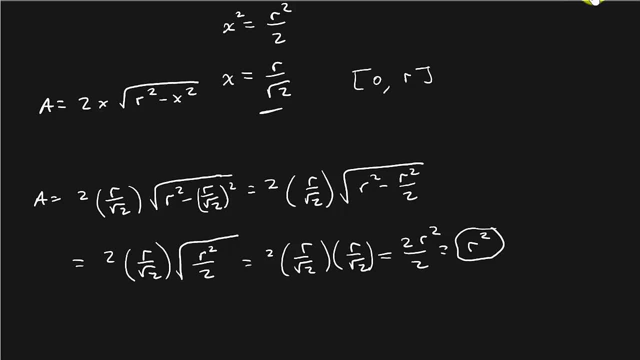 Check out my other videos. Give me a like, share and subscribe. Thanks for watching and I'll see you later.